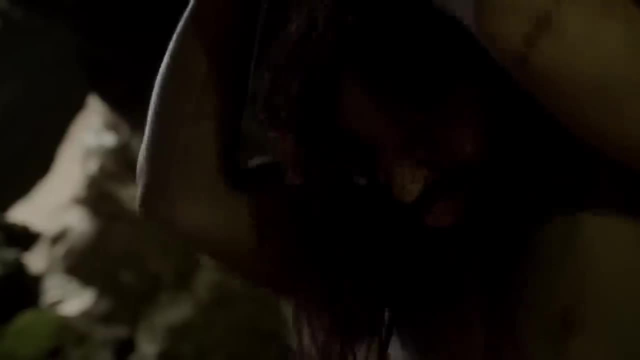 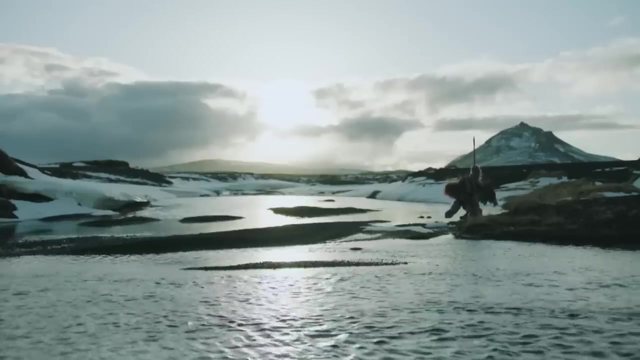 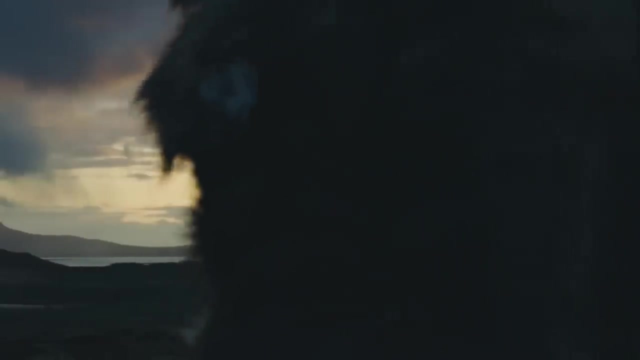 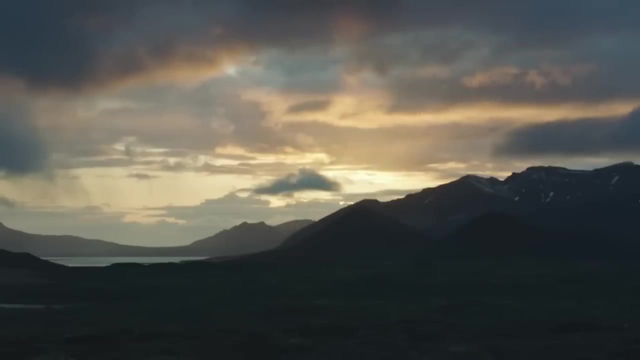 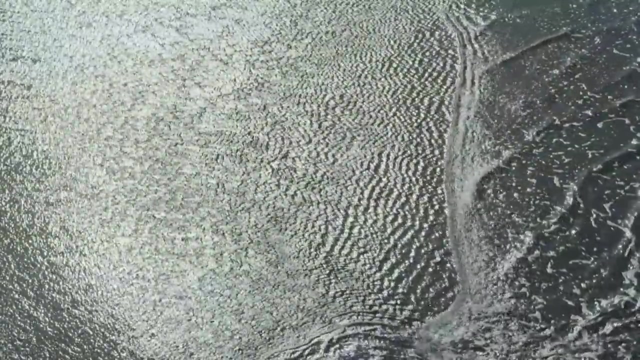 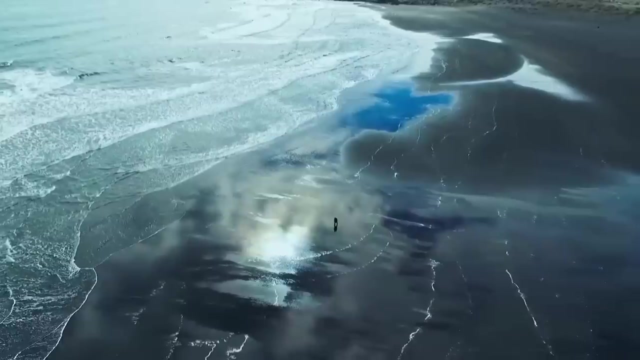 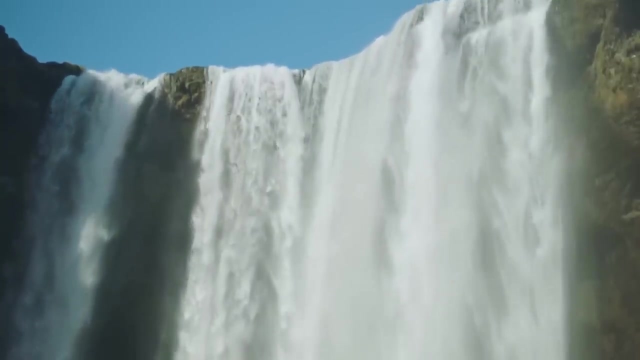 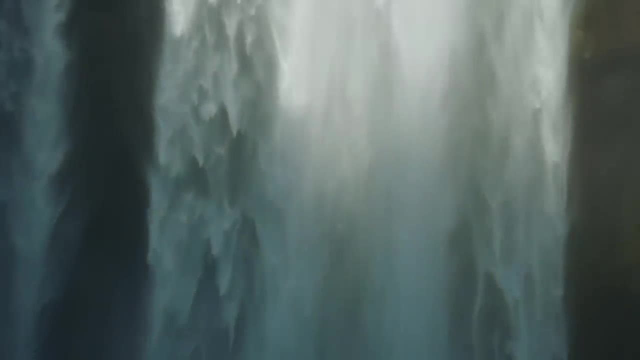 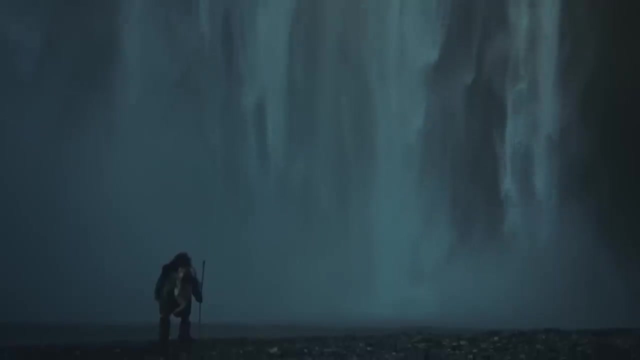 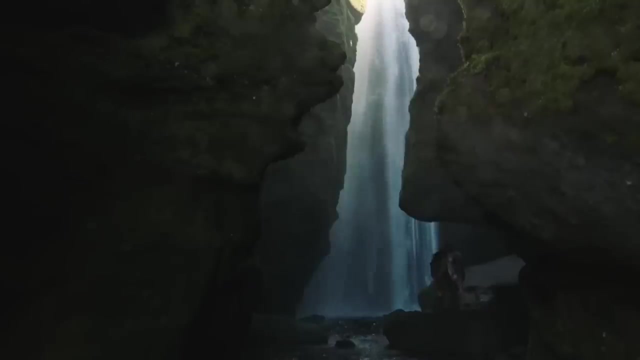 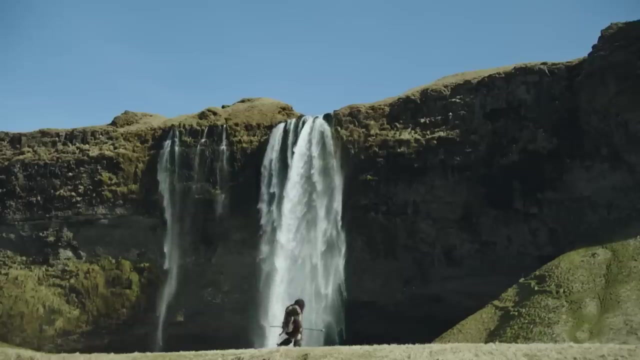 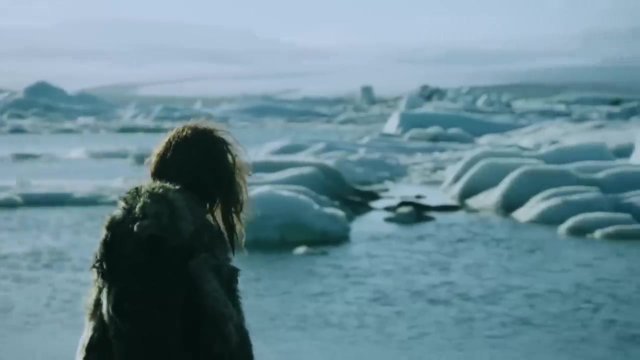 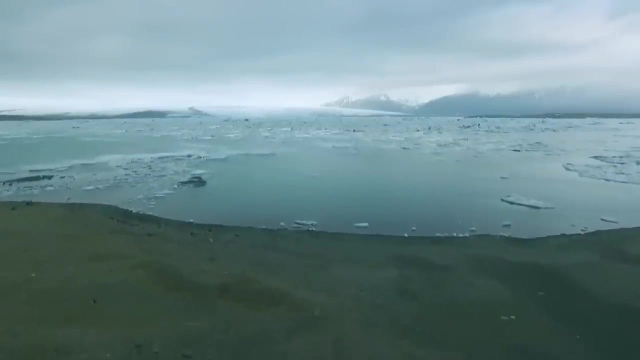 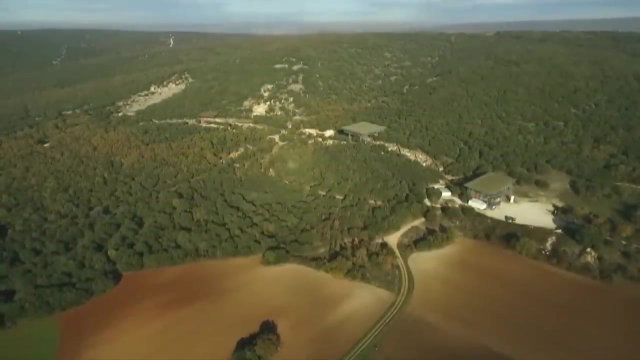 An individual who belonged to groups is now left out in solitude, With no one to share the fear of extinction. he endures life for a while. What could have been his last thoughts? Could his memory be found in us today, 950 meters above sea level? 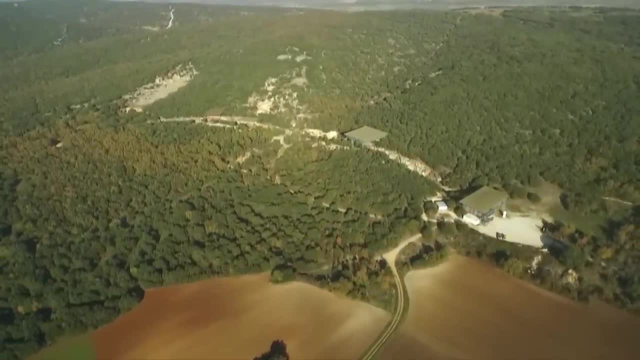 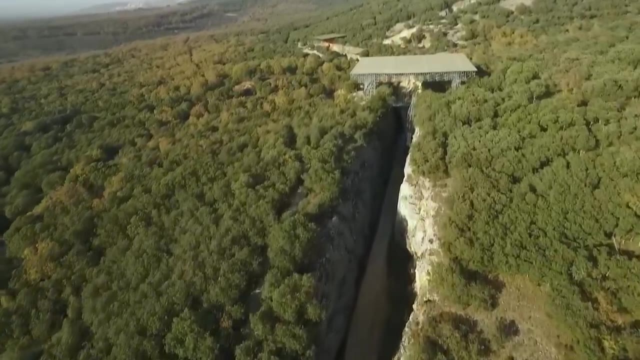 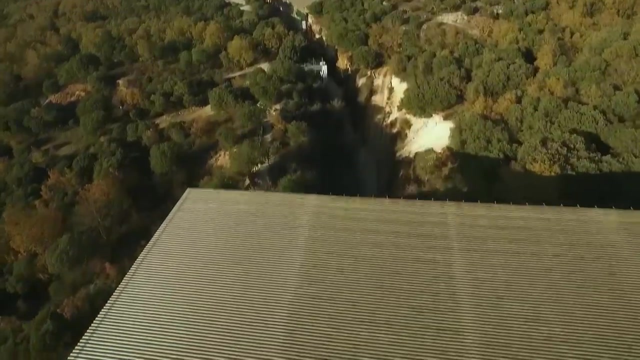 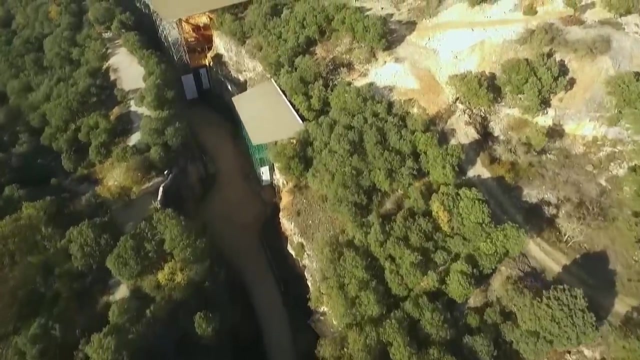 at the northeastern tip of the Spanish highlands In the late 1890s a limestone hill was discovered while building a tunnel for train tracks There, an astonishing discovery was made From one million years ago to 0 AD. 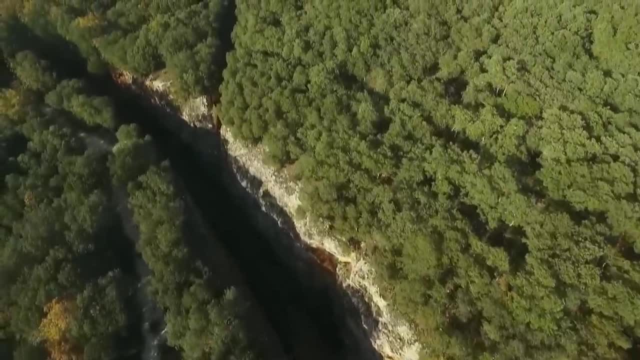 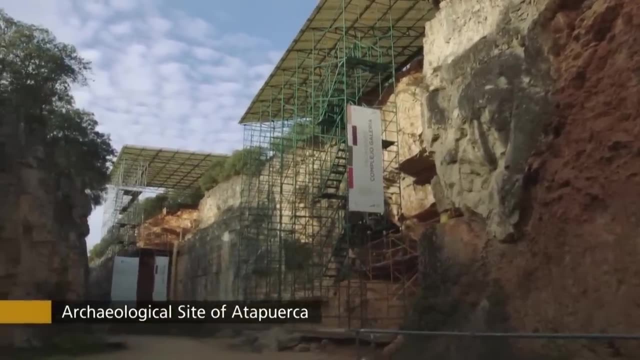 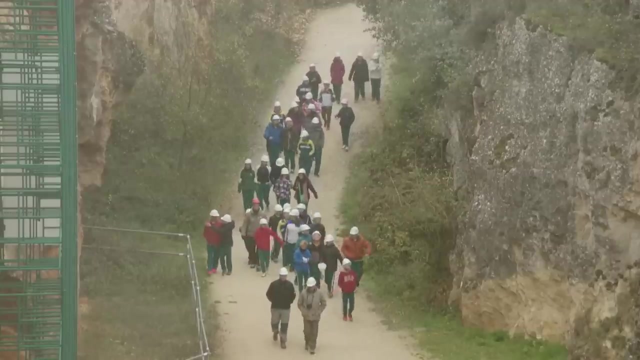 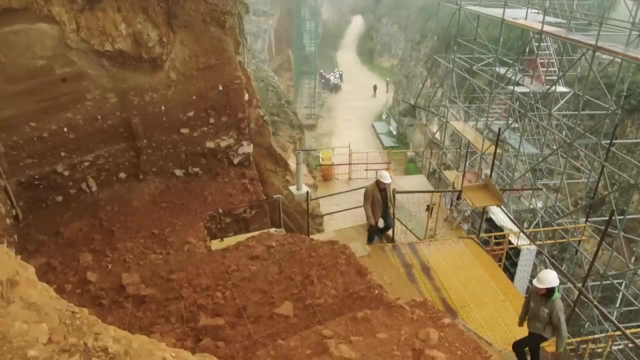 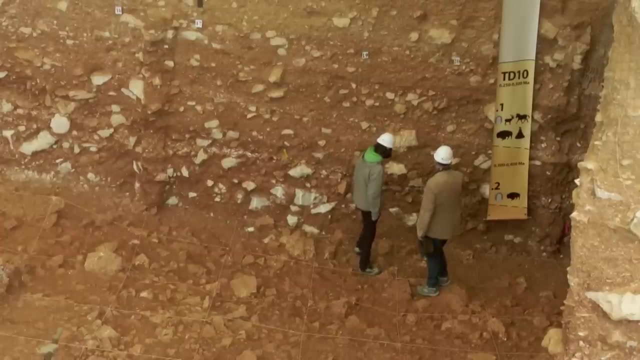 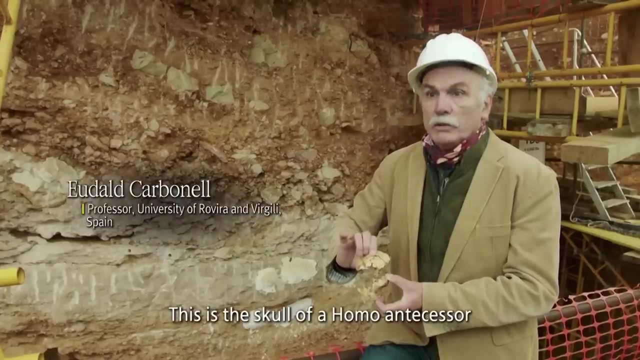 the hill had been a human habitat. In 1976, a student discovered a human jawbone here. Since then, it became the greatest archaeological site in the world. It became the greatest archaeological site in the 20th century. I have in my hands the skull of a Montecésor. 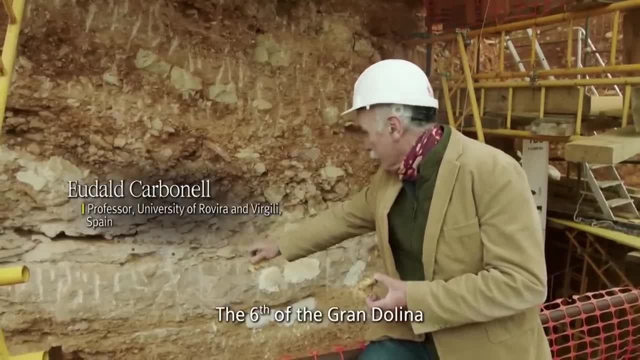 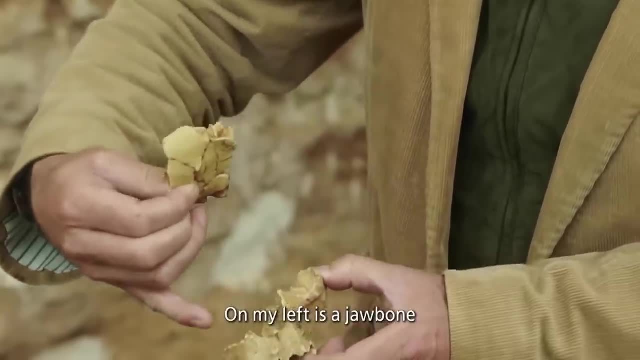 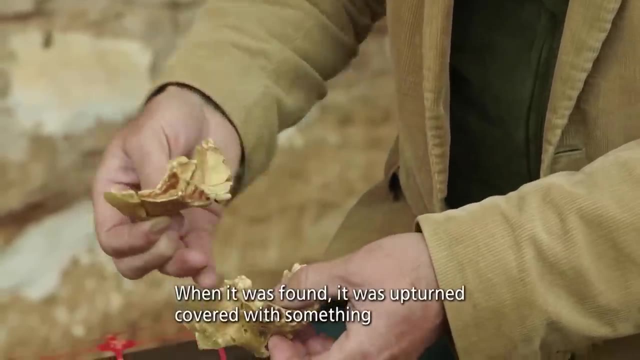 A Montecésor appeared just at this level, at level 6, at the base of the Grandolina. In my left hand I have the maxillary. We found it face down in the ground, all covered with material. We lifted it when it escaped. 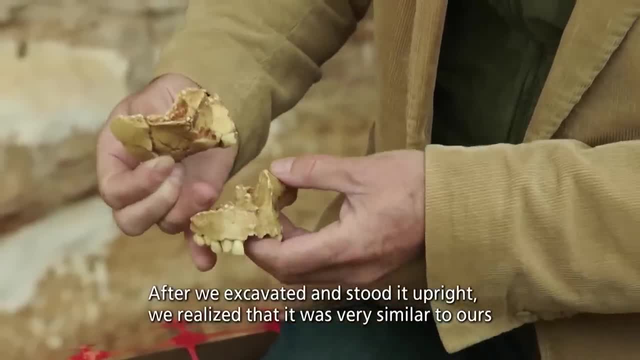 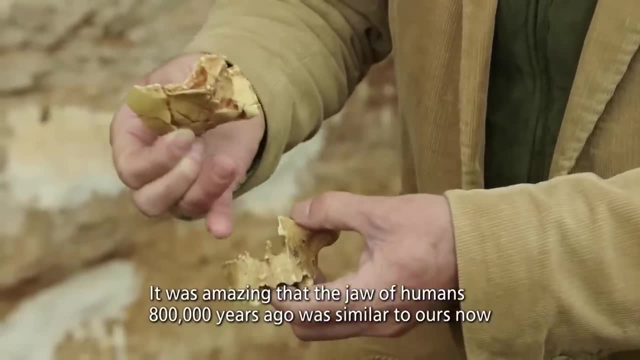 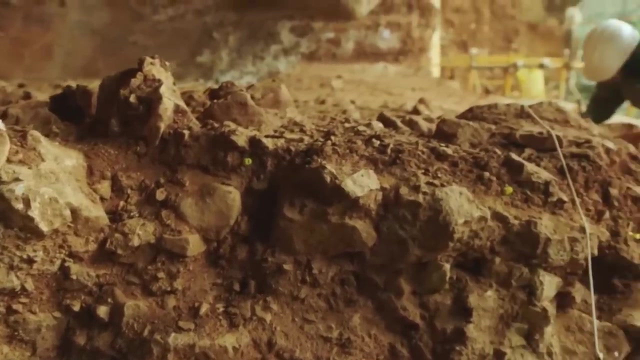 and we saw precisely that this maxillary was very similar to our species. We were surprised that an hominid 800,000 years ago had a maxillary very similar to ours. Archaeology begins from bones and stones. A scrupulous search is made to find clues. 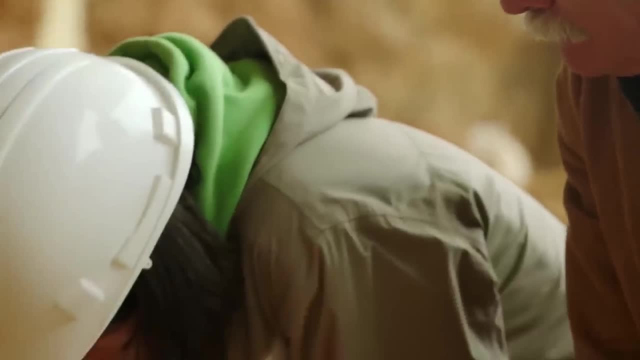 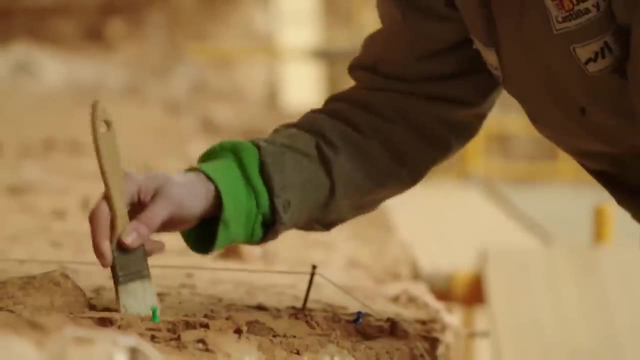 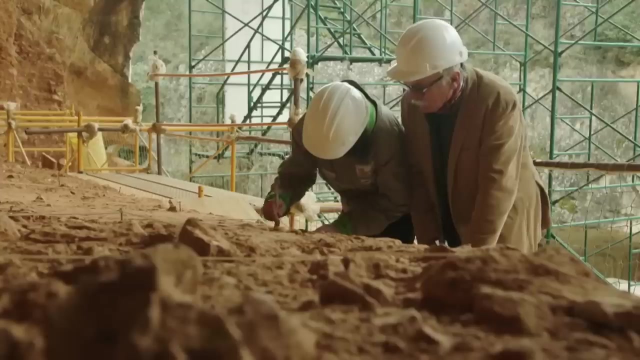 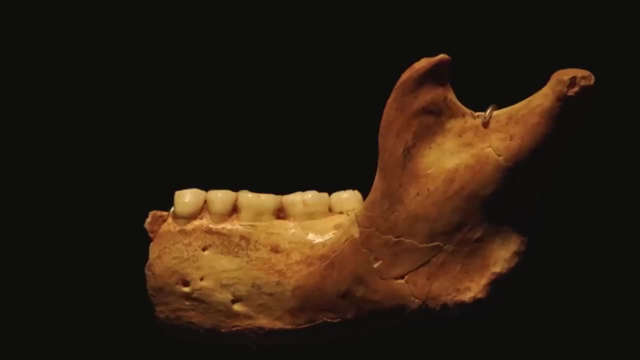 to understand who became modern humans and how. we homo sapiens are one of them. The largest number of human remains have been found since historic times. Time was dusted off and pieces were put together. Another species other than homo antecessor. 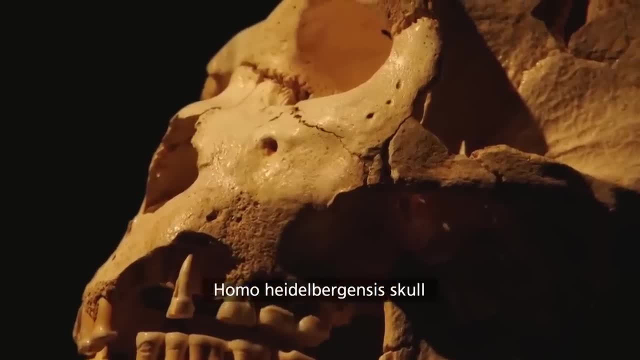 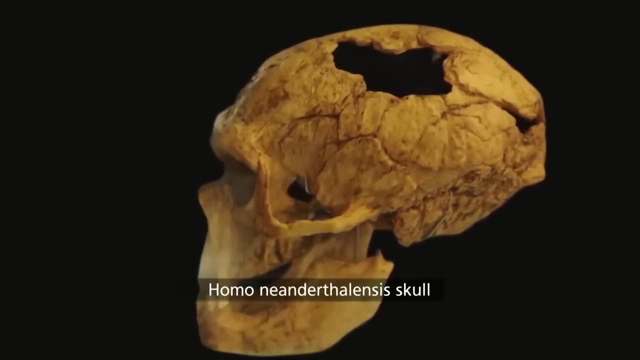 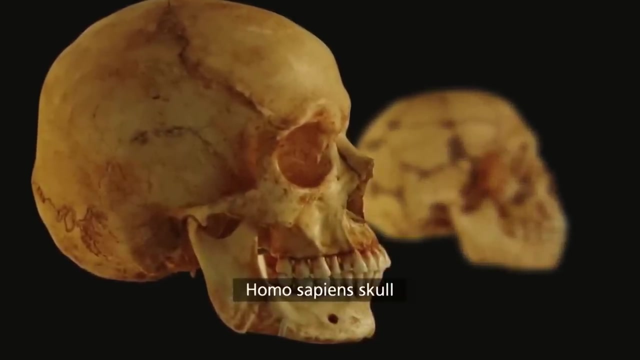 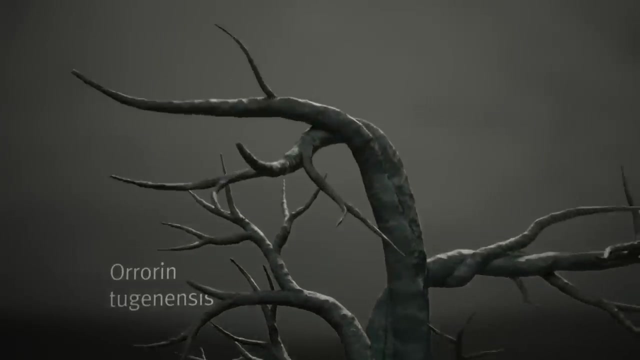 had existed for a million years, There was homo heidelbergensis. After a couple thousands of years, Neanderthals came along. Us homo sapiens arrived at the end. The genealogy of the human race is like a tree with many branches. 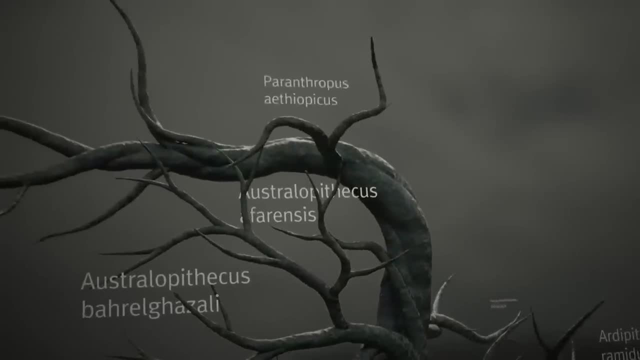 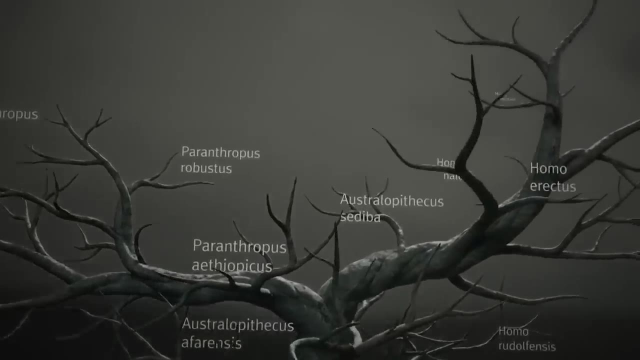 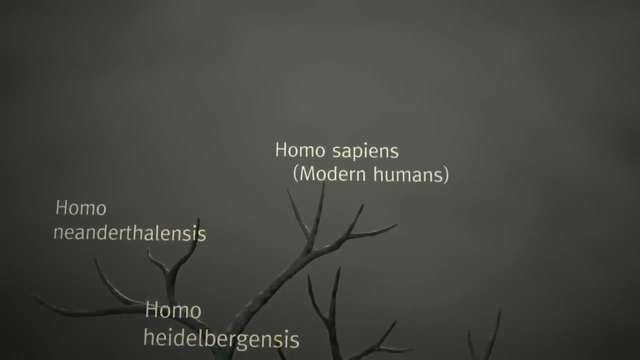 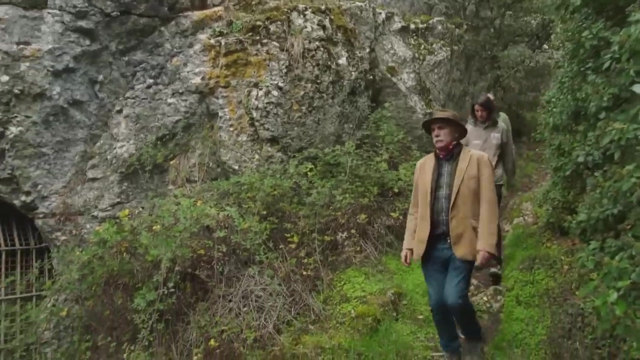 Breaking away from chimpanzees seven million years ago, humans have evolved into diverse species. The four types of humans found here were recent inhabitants of the Earth. Now we are the last survivors on the tree of human genealogy. It is unclear why we are the only ones left. 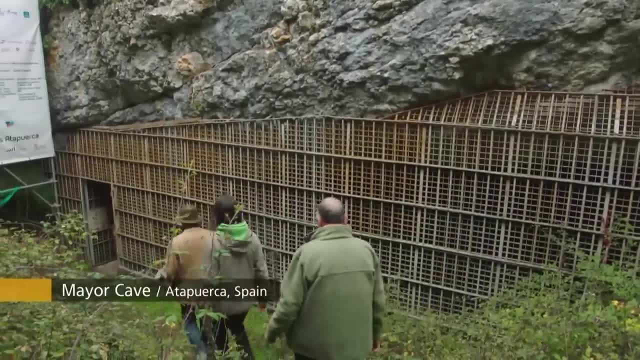 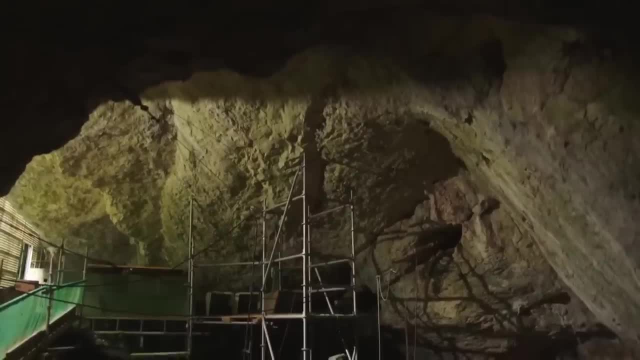 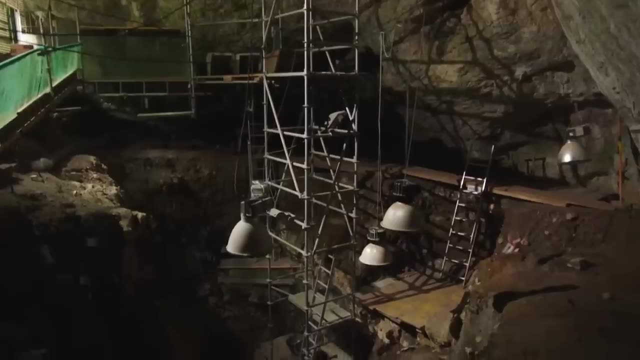 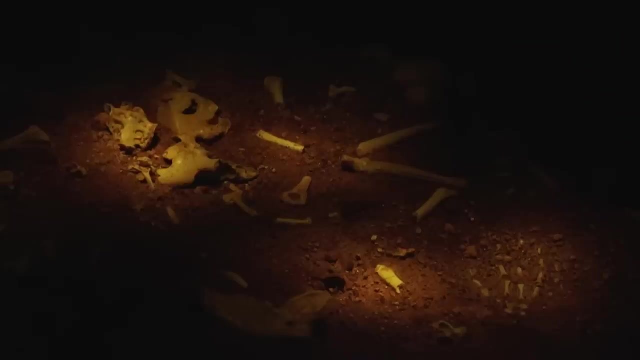 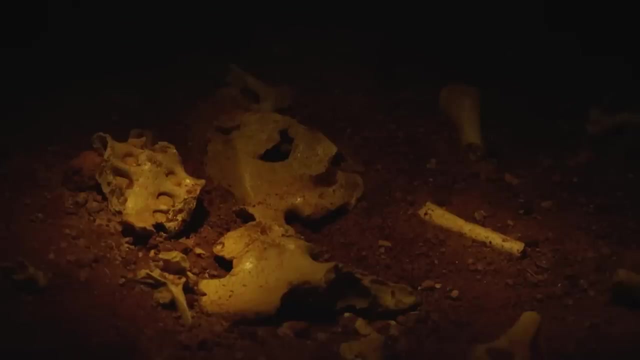 We can only take small steps towards the truth. The truth can be uncomfortable sometimes. A large pit full of bones was discovered while digging 13 meters below the ground. 5,500 pieces of bones belonging to 28 people in total, Mostly in their late teens and twenties. 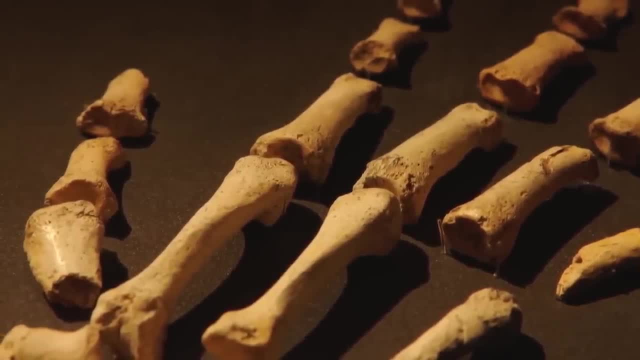 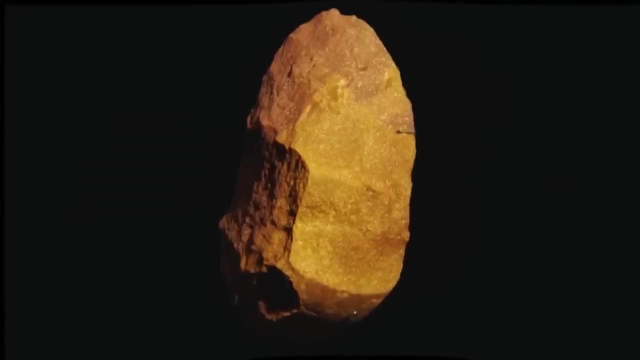 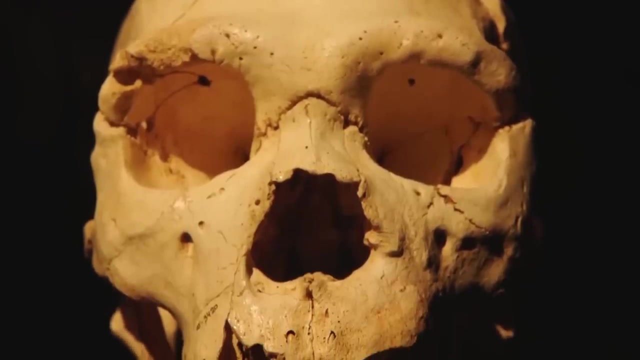 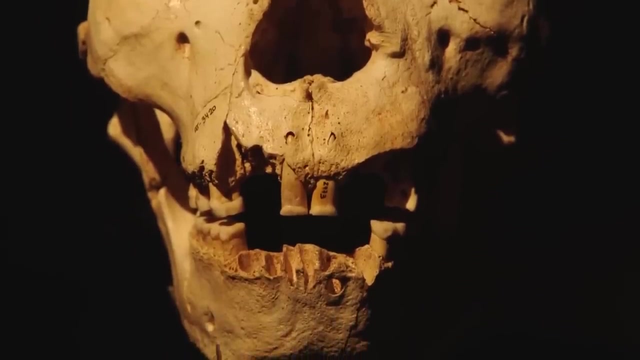 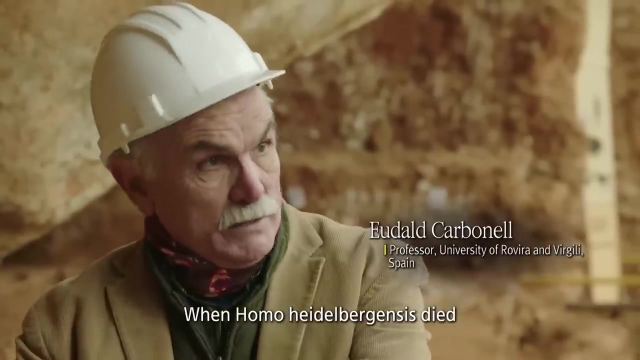 They had been buried in a mass grave. Another strange thing was this stone axe. It is made of quartzite, which is too soft to make tools. Homo heidelbergensis was the owner. What had happened to them? If it is only an intentional accumulation of corpses? 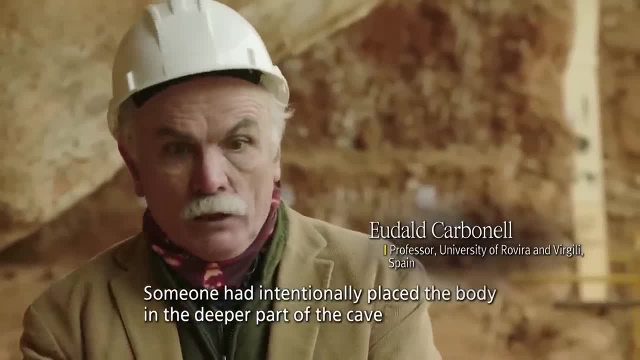 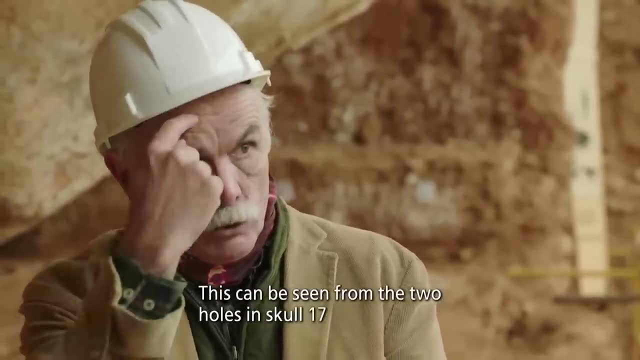 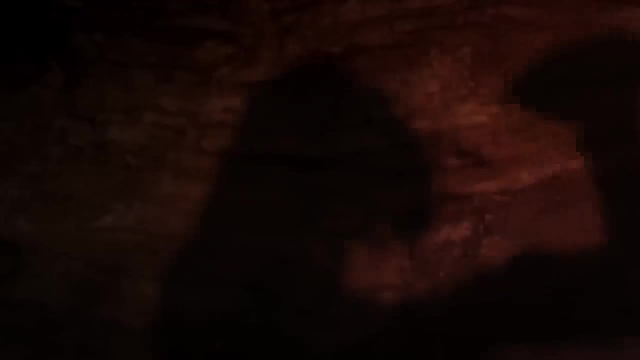 that is, when someone was killed or died, they deposited it in their interior. We do know that this was the case, because skull number 17 has two perforations. In fact, when they played this part, they were able to figure it out. 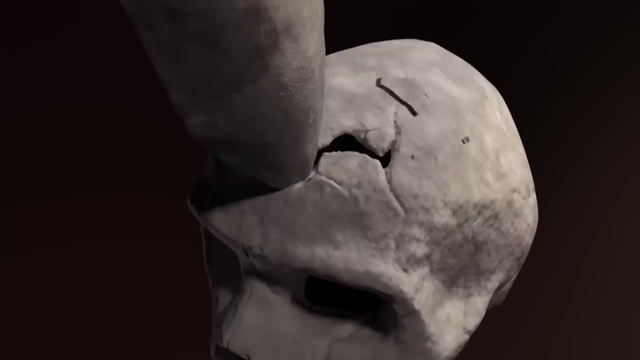 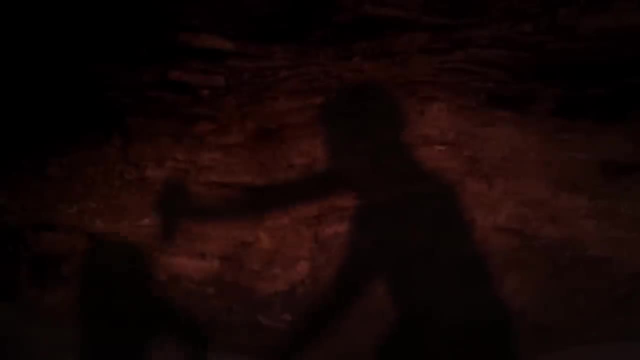 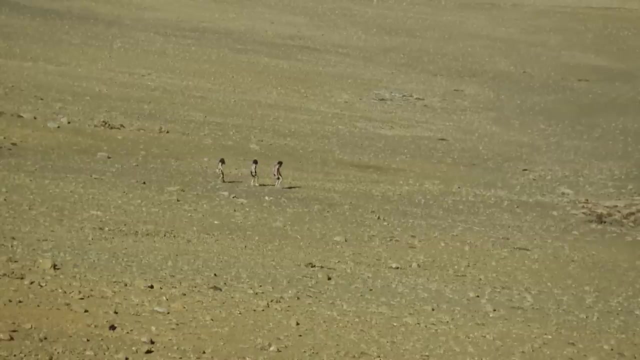 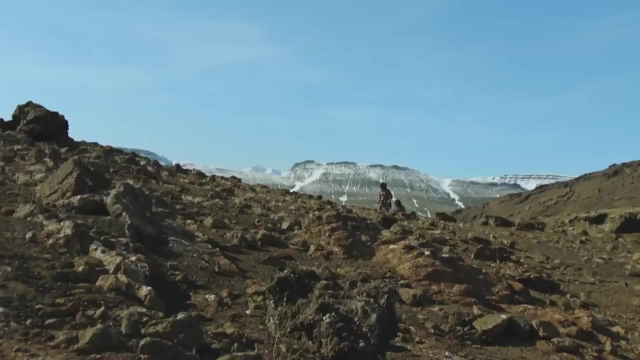 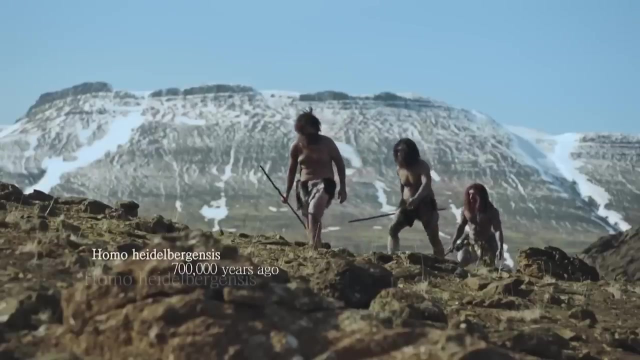 The continuous hits near the left eye socket of the skull. They were a deliberate murder. Somewhere over there there is a dark, dark mirror: Homo heidelbergensis, a human species that appeared 700,000 years ago and lived for 500,000 years. 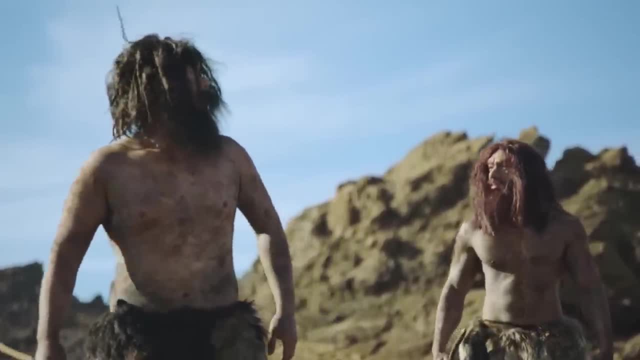 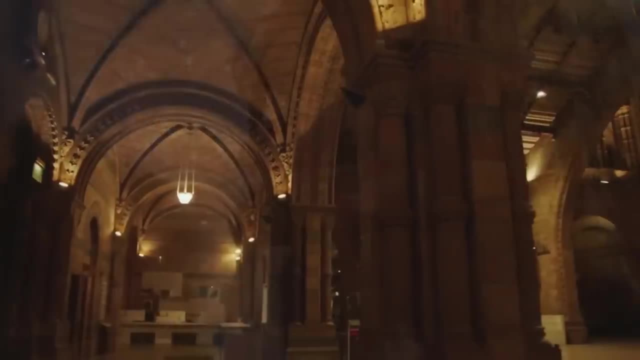 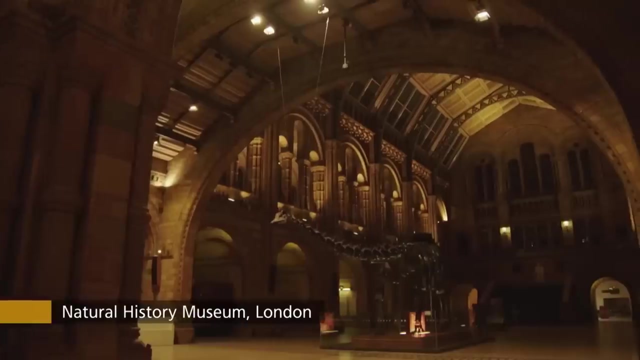 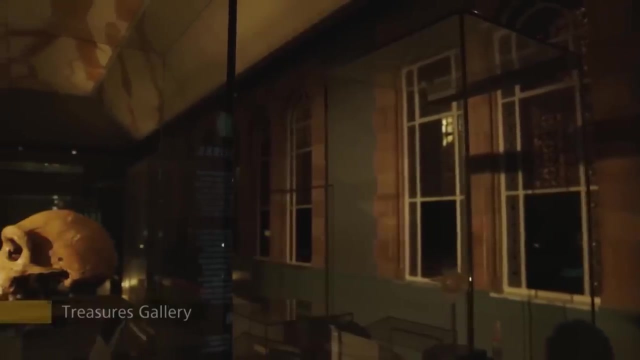 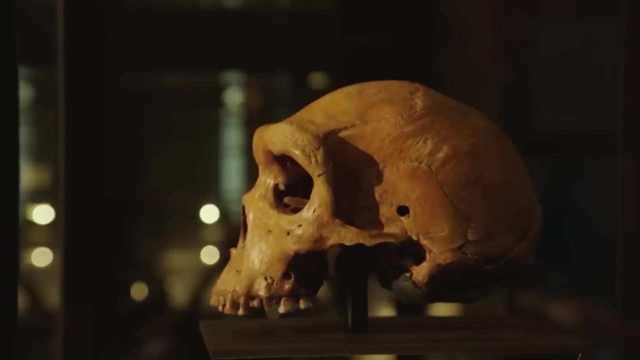 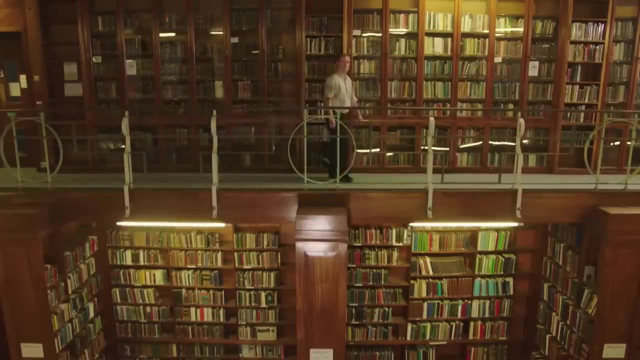 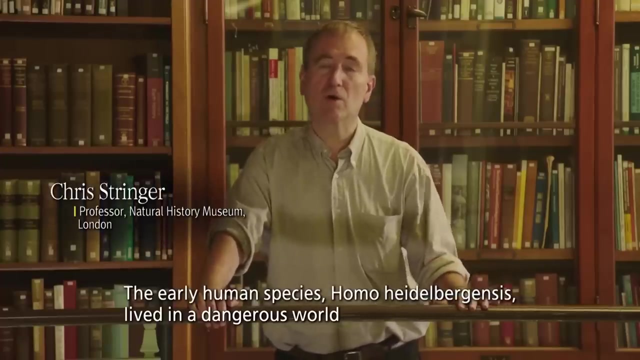 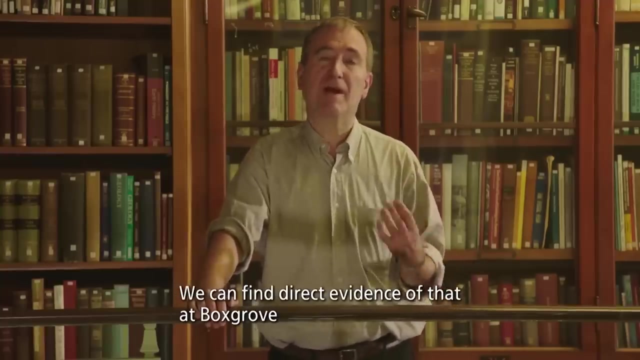 They are a shared ancestor between Neanderthals and us, known as the first humans who practiced intraspecies killing. The cold silence reveals another truth: The early human species, Homo heidelbergensis, lived in a dangerous world alongside animals like lions, hyenas, wolves and bears, and we can find direct evidence of that at Boxgrove. 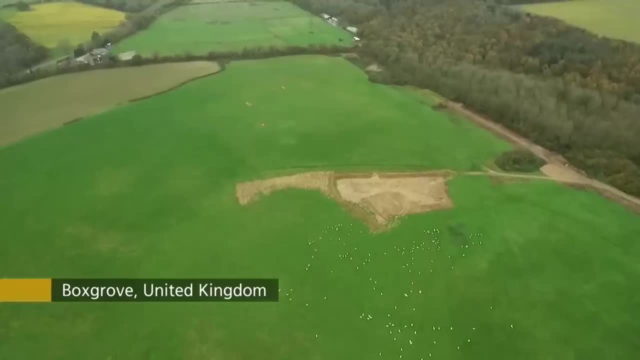 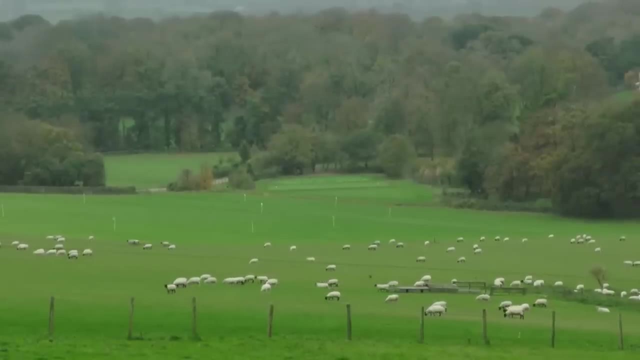 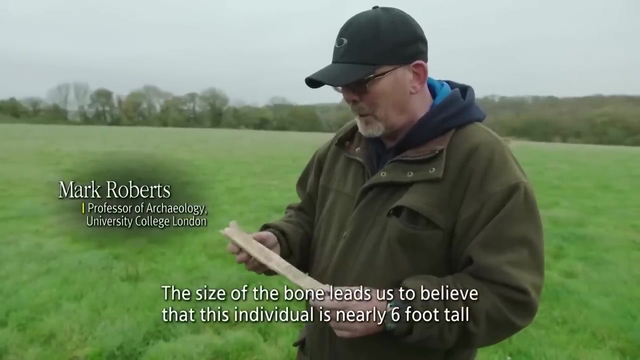 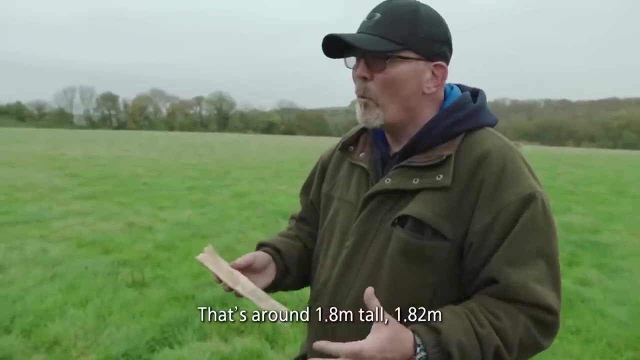 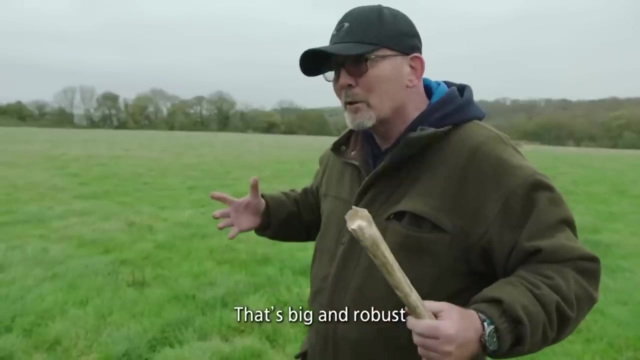 Boxgrove, located in southern England, used to be a quarry. Here a leg bone belonging to a well-built man in his twenties was found. The size of the bone leads us to believe that this individual is nearly six foot tall, so that's around one meter eighty tall. one meter eighty-two. that's big and robust. 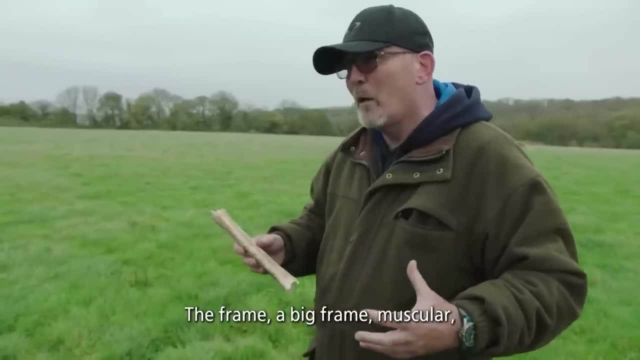 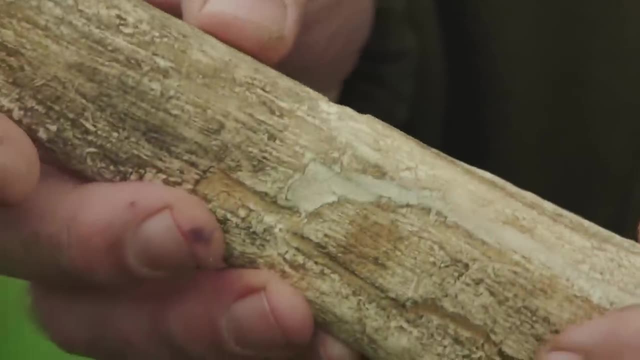 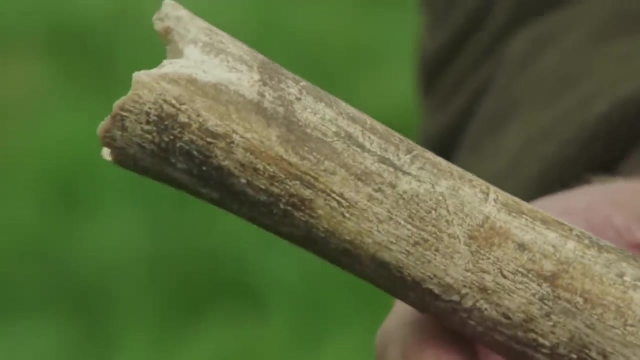 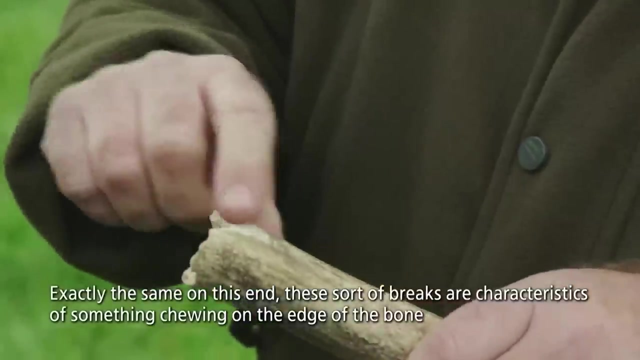 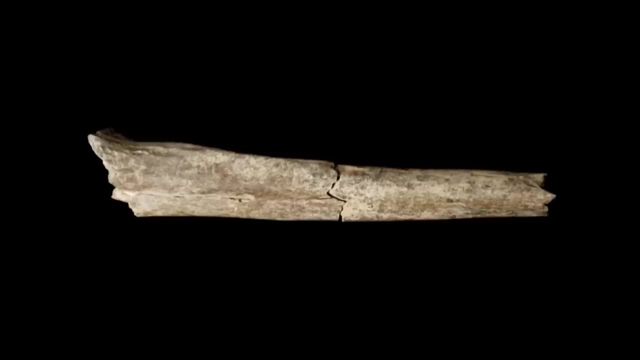 So the frame, a big frame, muscular, something maybe like a modern-day rugby player, The bone also reveals its final moments, Manner of an animal chewing on that end of the bone and exactly the same on this end. These sort of breaks are characteristic of something chewing on the ends of the bone. 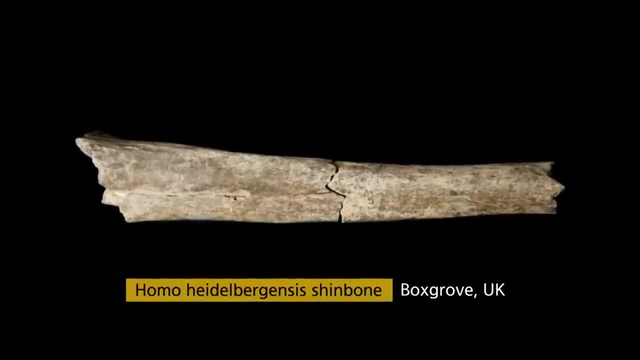 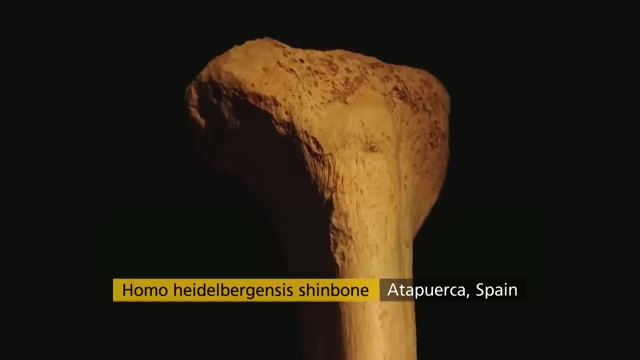 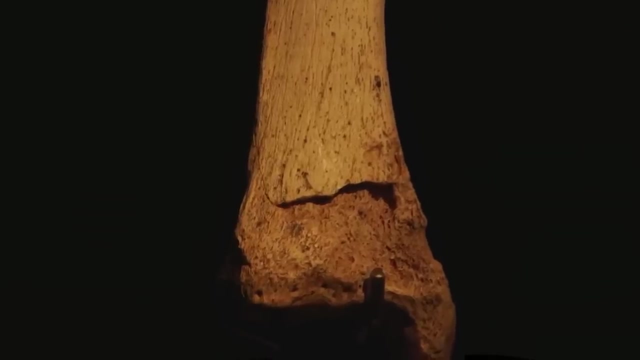 The owner of this bone had been eaten by an animal. You can see an unusual amount of scars on Heidelbergensis' bone, which is proof of his exhausting life. You can see an unusual amount of scars on Heidelbergensis' bone, which is proof of his exhausting life. 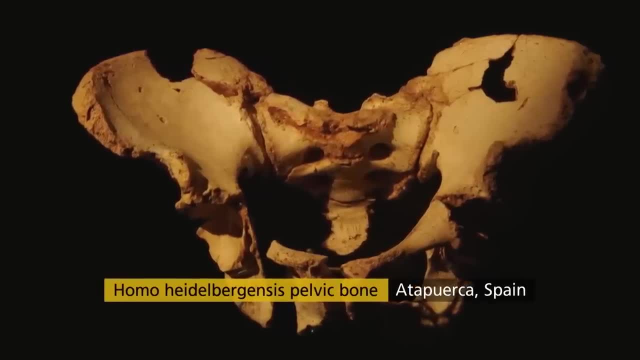 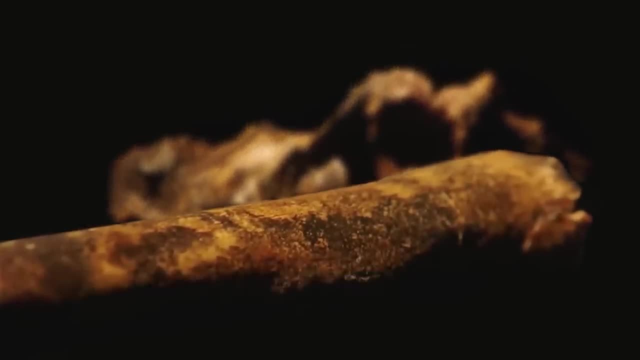 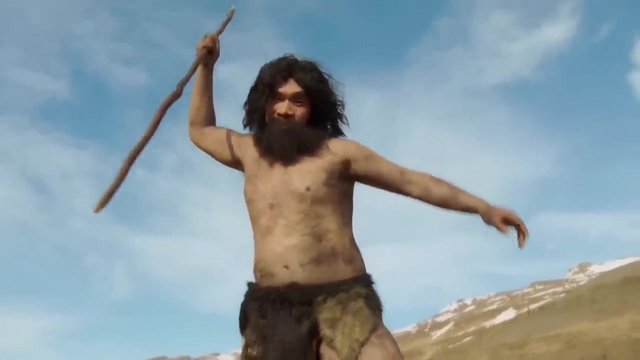 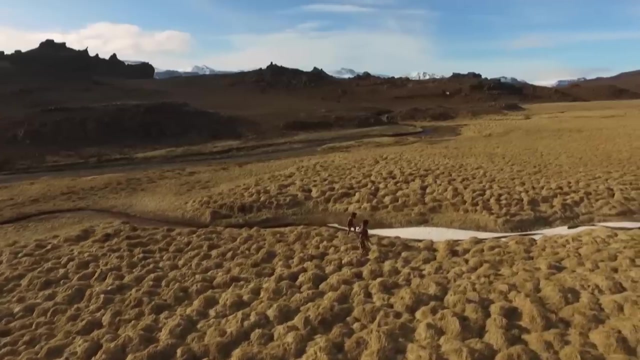 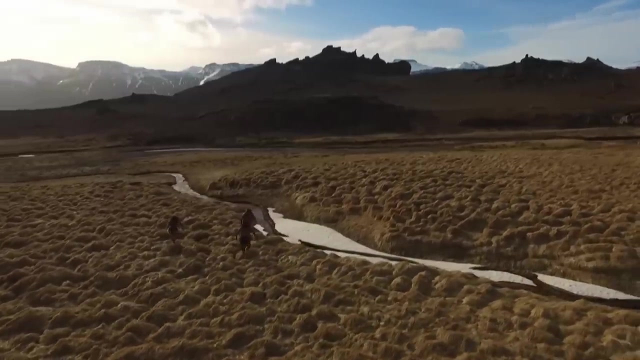 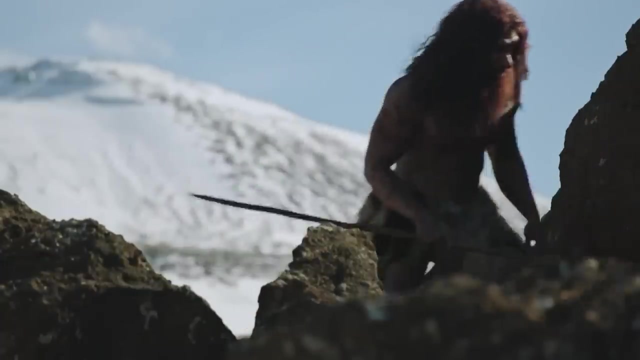 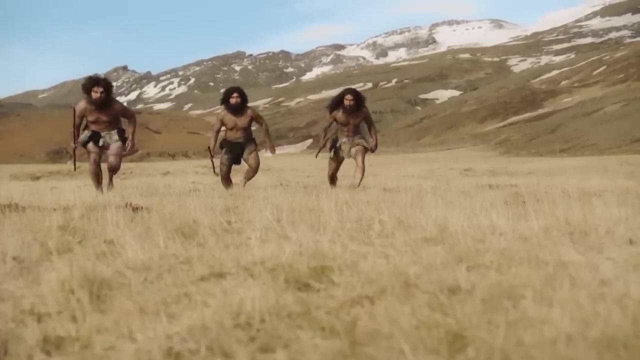 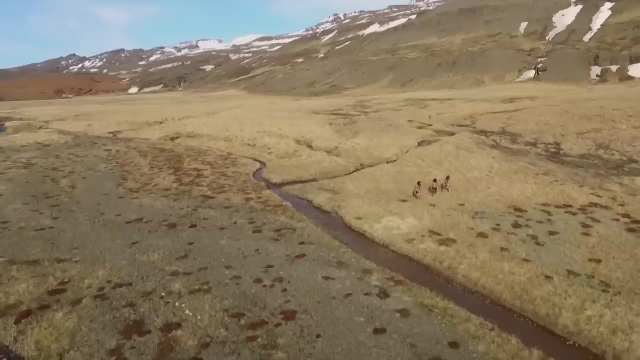 Still, his robust frame could easily withstand a ninety kilogram body weight. Homo heidelbergensis: the most intelligent humans on the earth. Two to three human species co-existed with them, But none of them managed to out-survive Homo heidelbergensis. 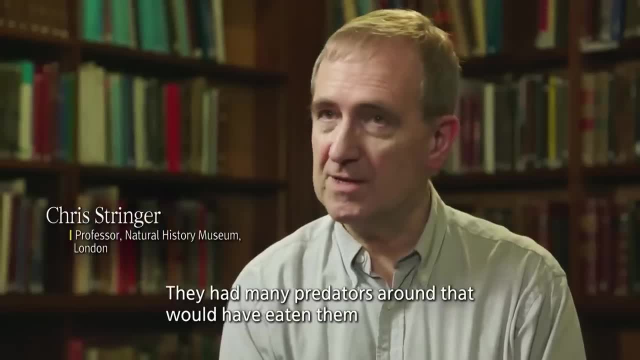 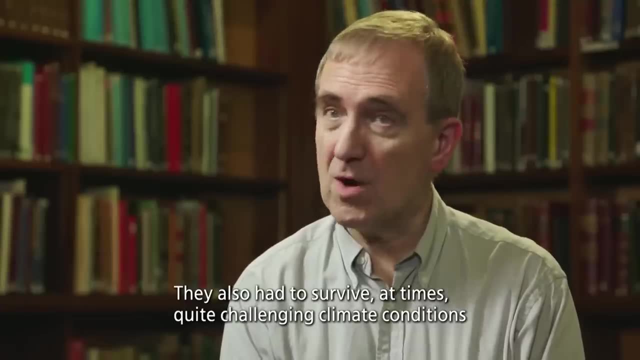 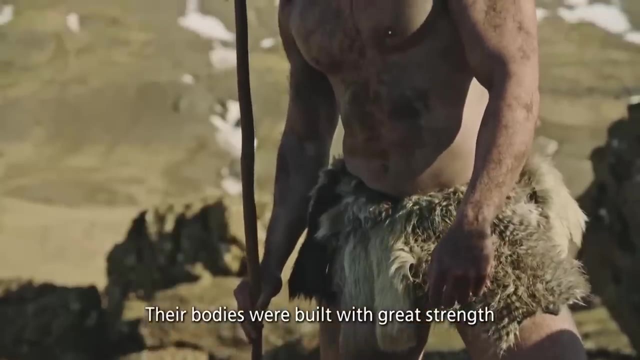 Life was certainly dangerous for these people. They had many predators around that would have eaten them. They also had to survive, at times, quite challenging climate conditions. The winters could have been very cold. And, yes, their bodies were built with great strength. They had a lot of muscles. they had very thick bones. 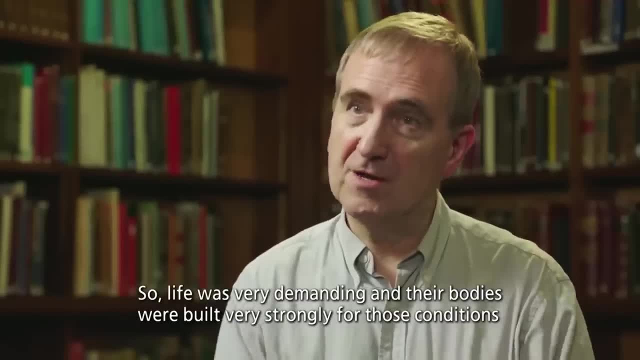 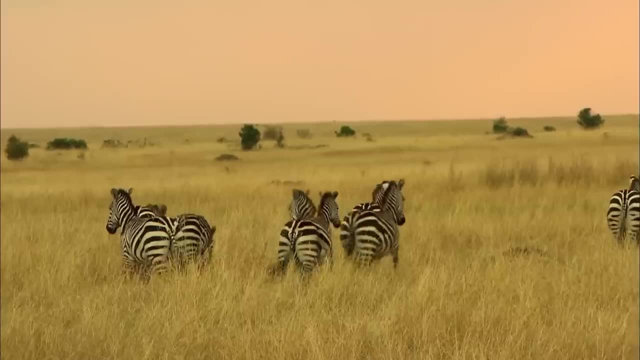 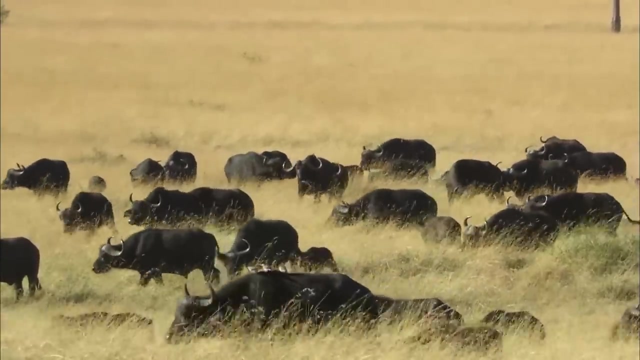 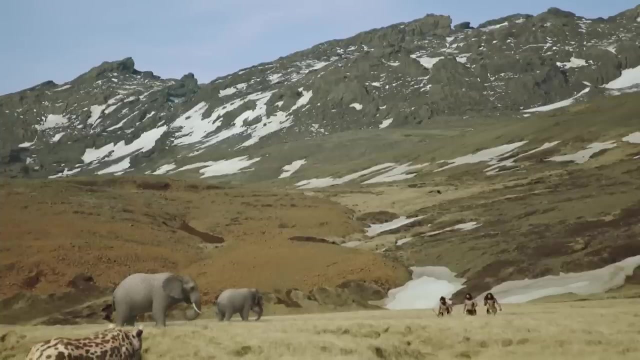 So life was very demanding and their bodies were built very strongly for those conditions. The ecosystem was different from what it is now. Zebras weighed 80 kilograms more. An African buffalo had horns two and a half times longer. Presumably humans had to grow bigger. 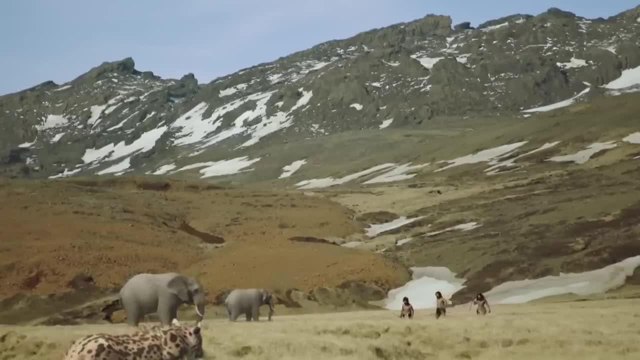 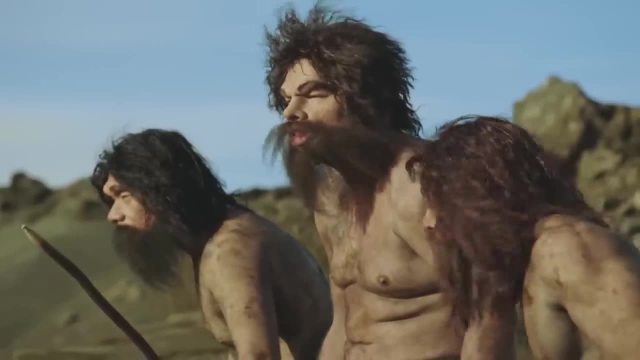 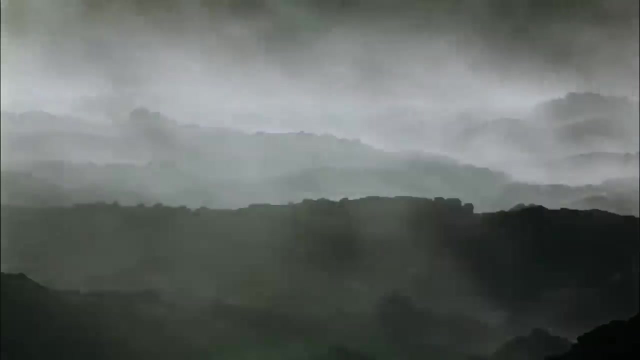 2 00-話. The glacial period came and the earth became more arid. 0 00-話. Fierce competitions for food were inevitable. 1 00-話. Zondas raised its heads in noticeable protest. 5 00-話. 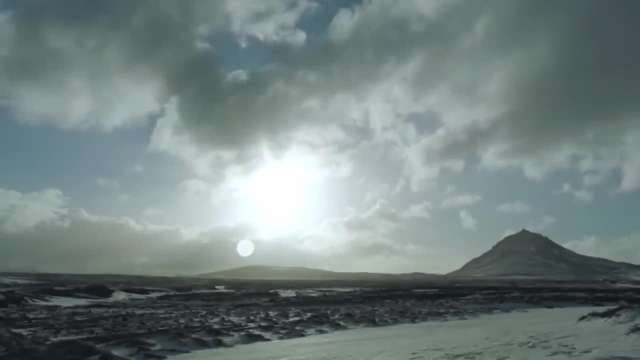 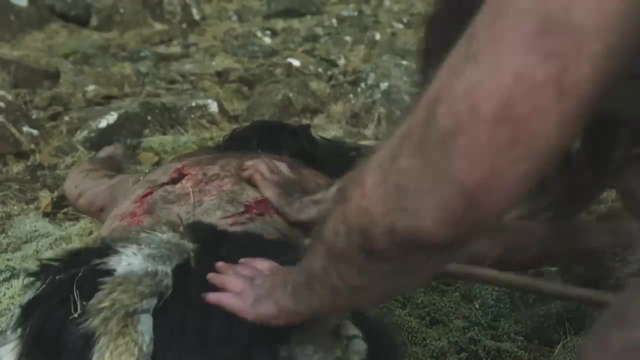 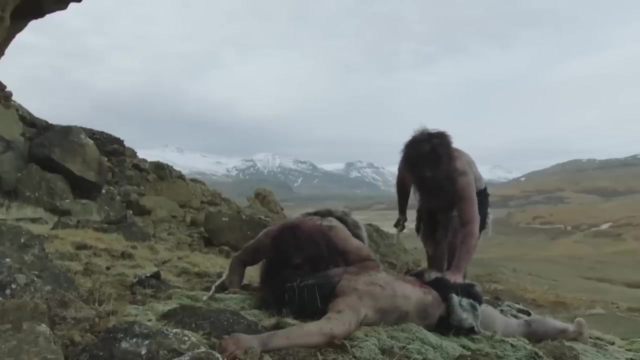 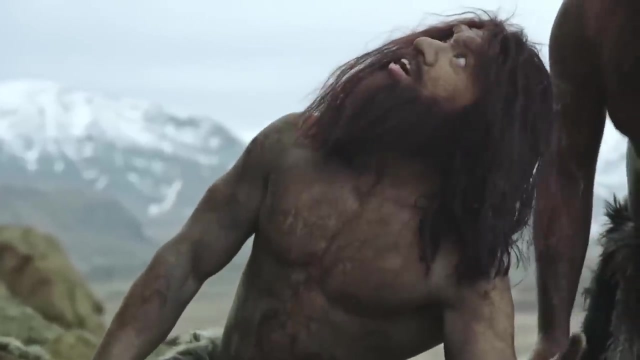 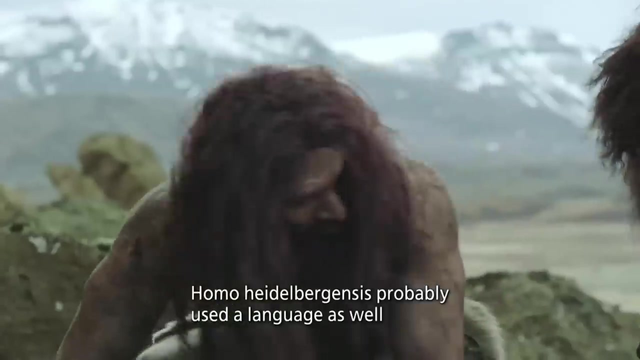 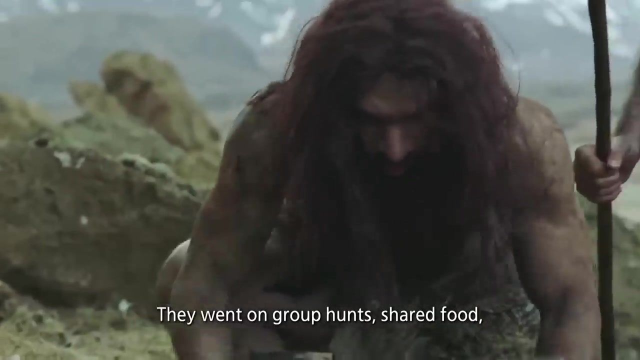 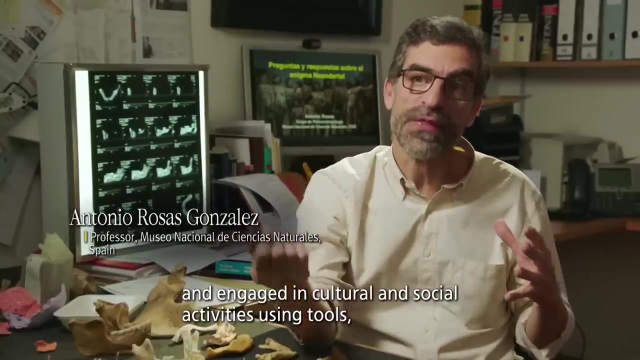 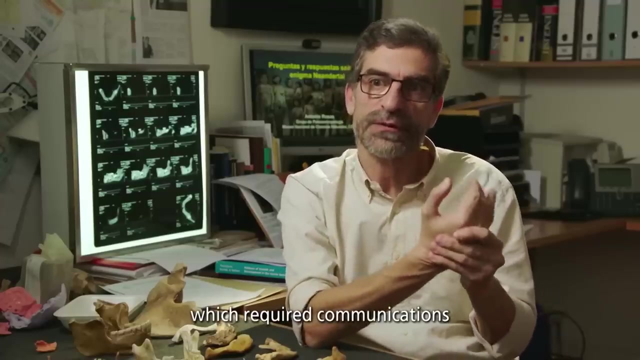 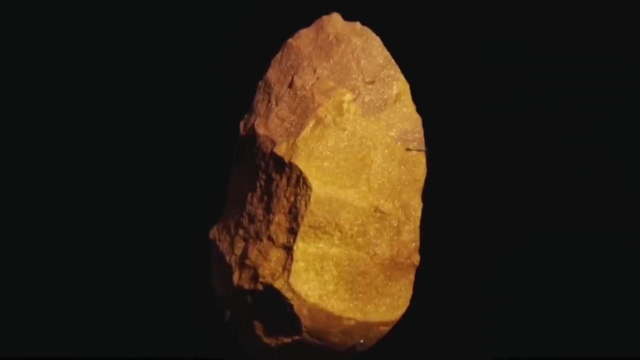 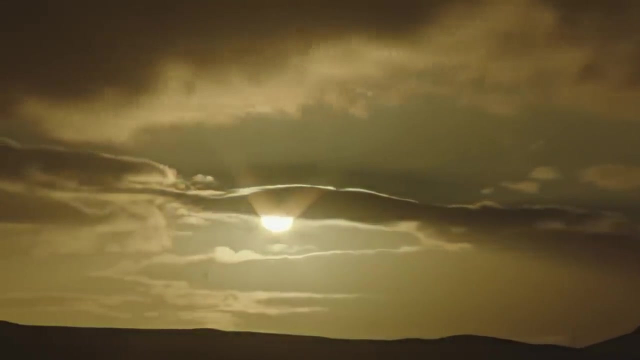 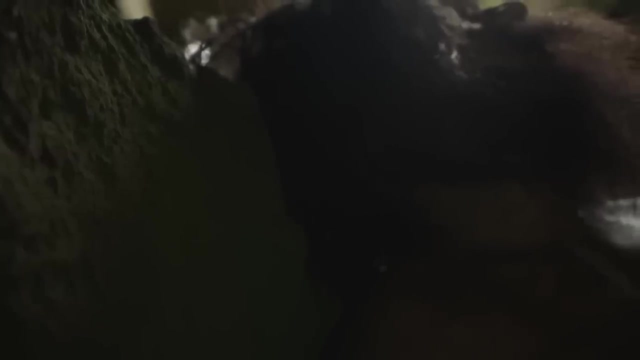 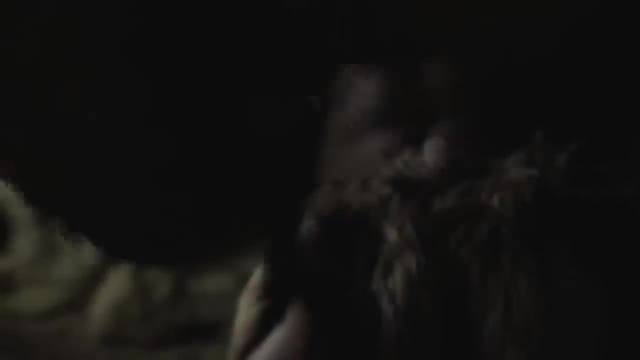 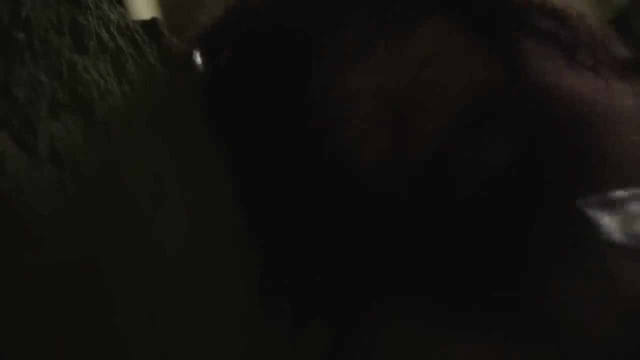 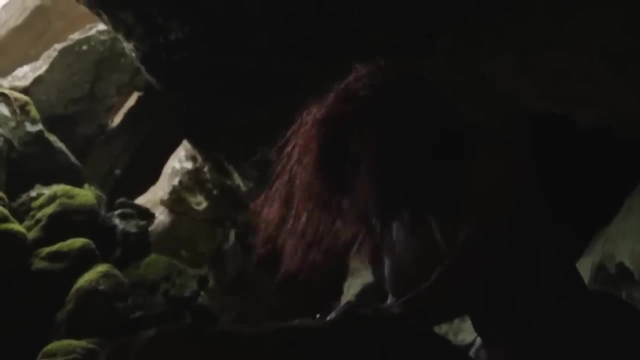 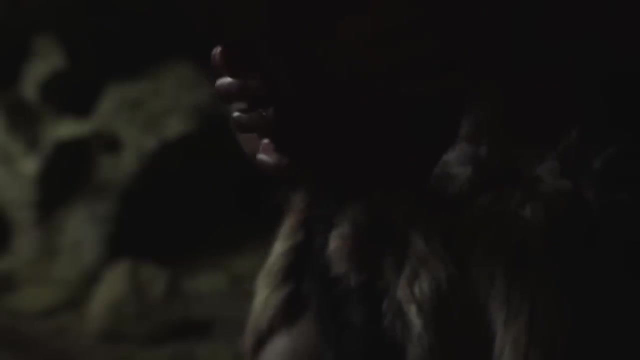 Zodalan 大咆猫. The années plus paused just 0: 00-話. The death of a peer puts the entire group into peril. The group must overcome the shock. It needs communication. This murder scene could be reinterpreted. 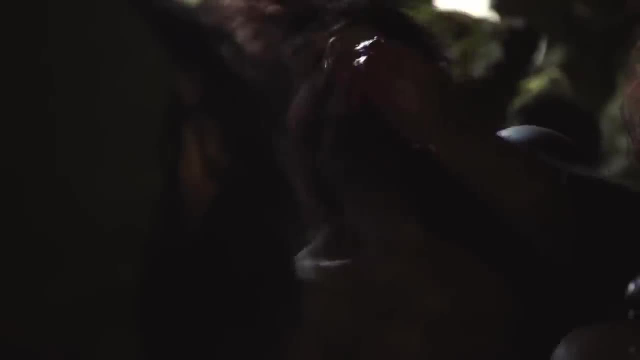 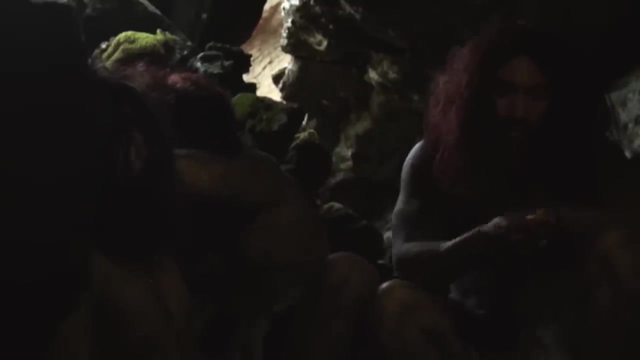 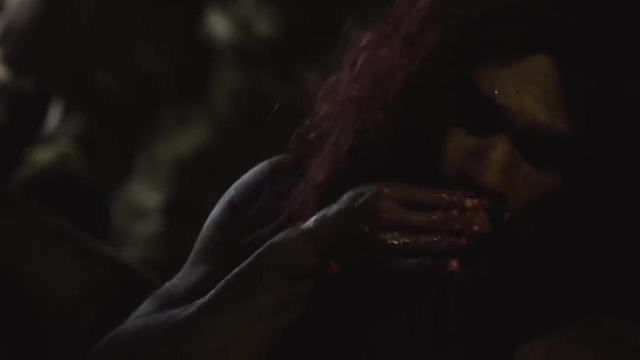 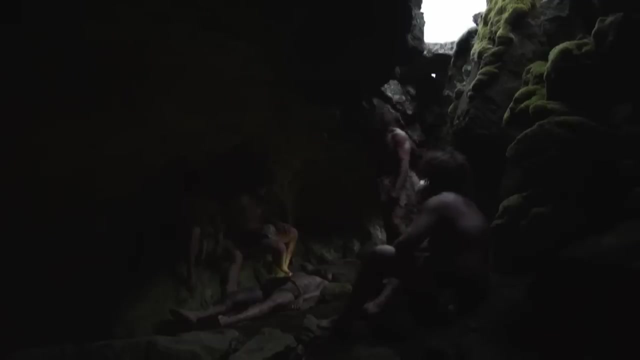 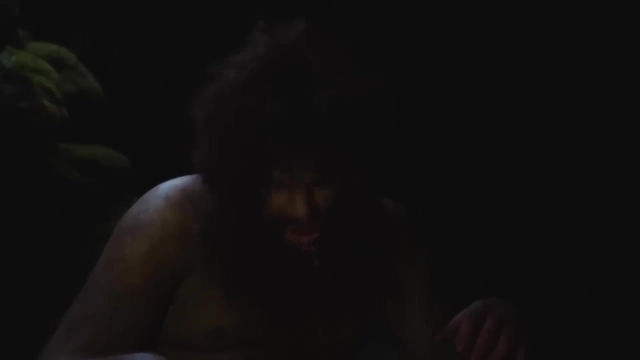 They crack the skull of the dead open, mashed his bones and ate it. Could hunger be the reason? The primitive tradition, eating brains of dead to gain wisdom could have been in play. The reddish rock, the abyss, the abyss. 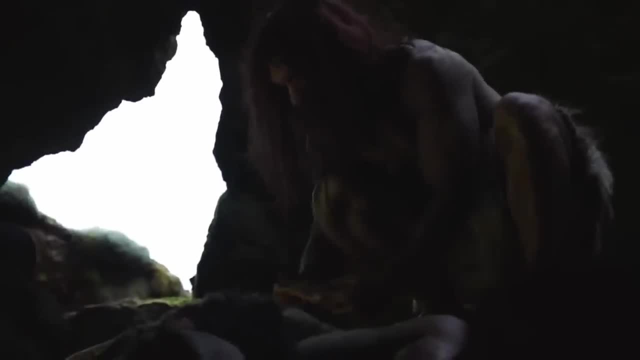 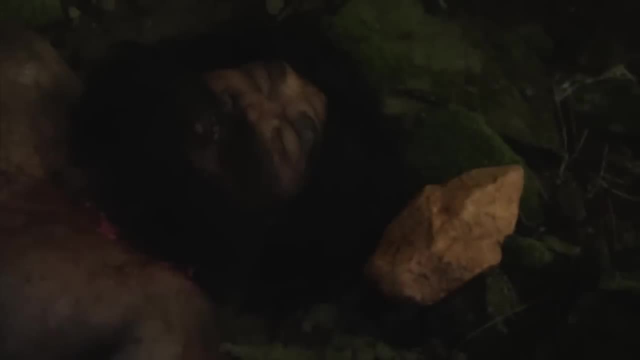 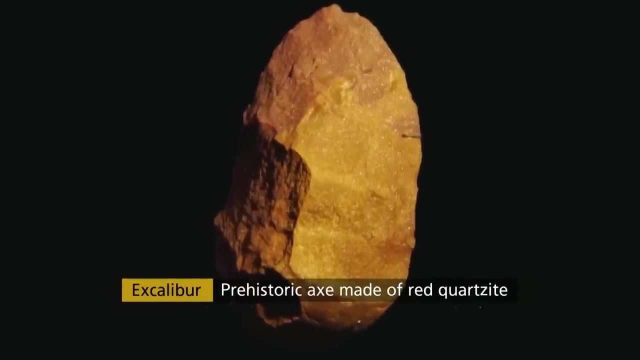 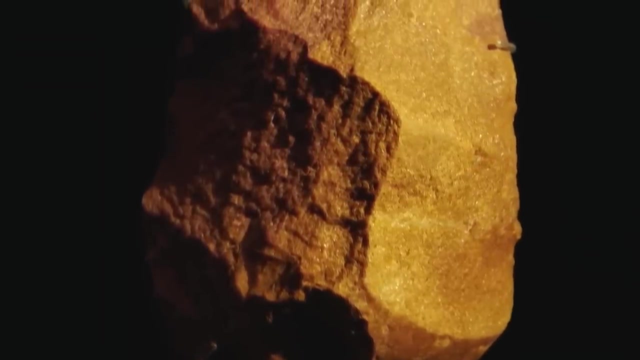 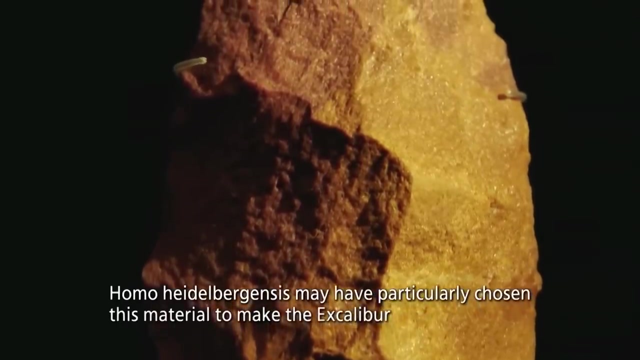 the abyss, traveled far to obtain, was used for this particular purpose. This is why the stone axe was placed next to the corpse, Evidence for the beginning of a spiritual ritual. In this case, language is no longer an impossibility. It is for this reason that we think that Excalibur was selected as the first material. 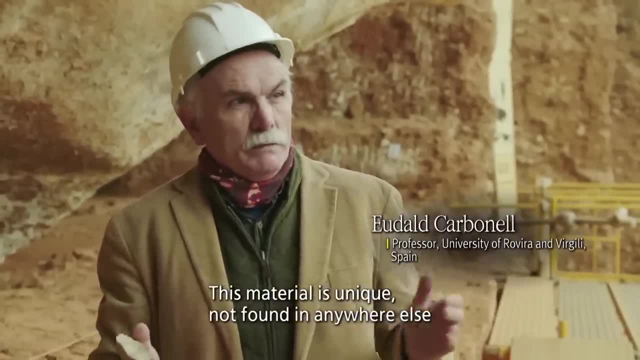 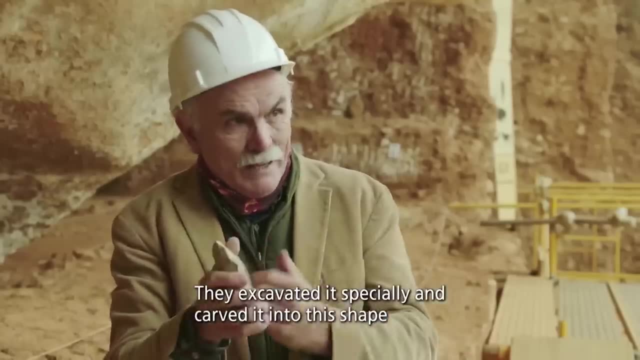 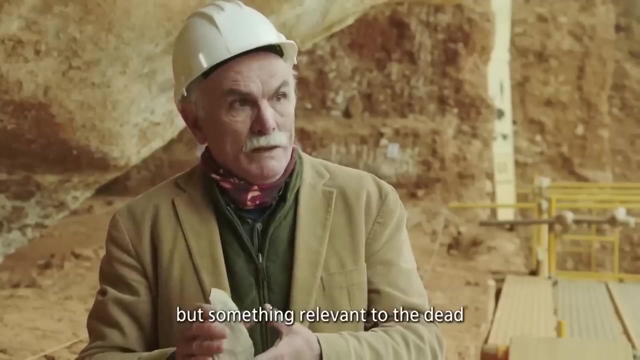 and this first material- unique because we have not found this material in the camp or anywhere else- was specially collected and carved to have these characteristics, And that is why we think that Excalibur could be an object not only to work but also a motive. 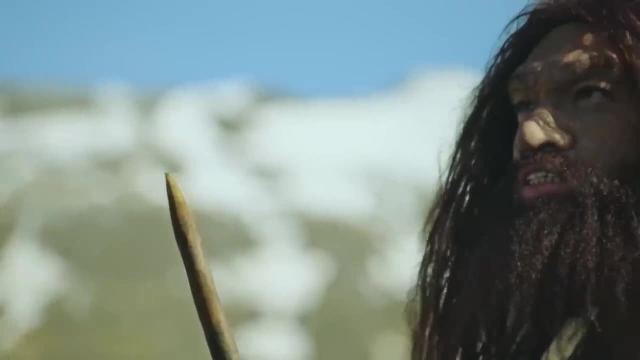 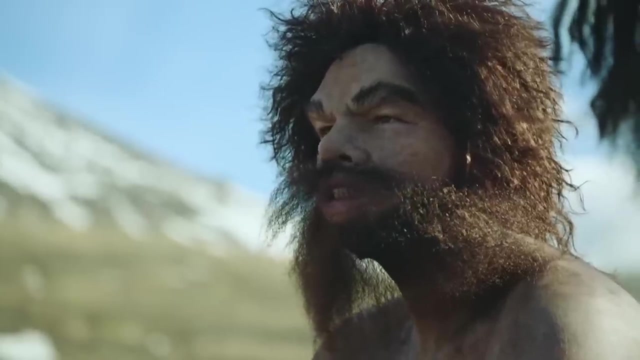 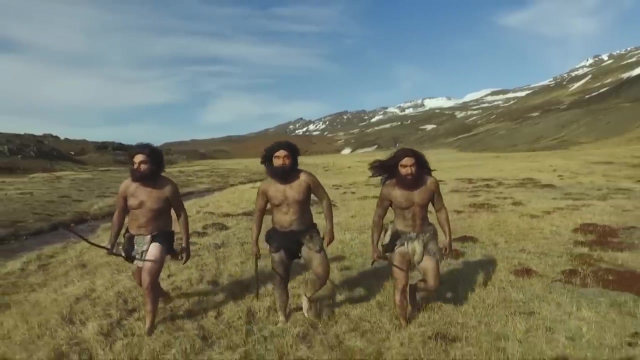 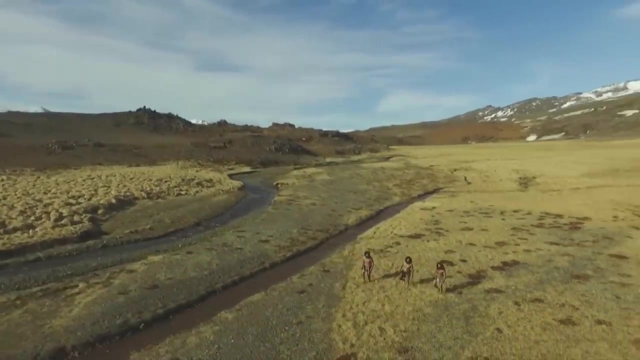 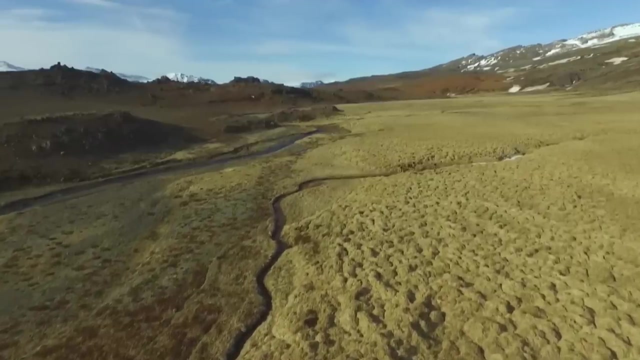 to associate with the dead. The climate is becoming increasingly colder. Those with larger bodies manage to bear beyond their limits. Ultimately, yielded by drastic changes of the earth, they disappear. Next, a stronger humankind, better suited for the coldness, appears. 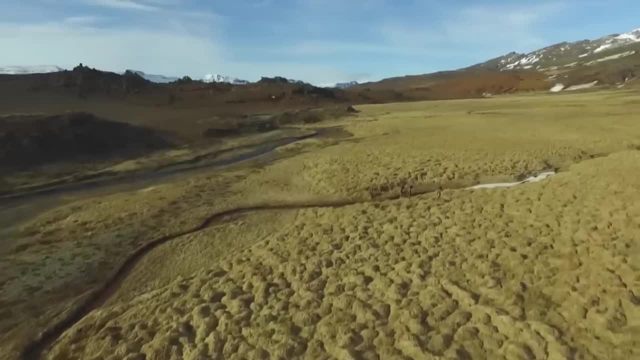 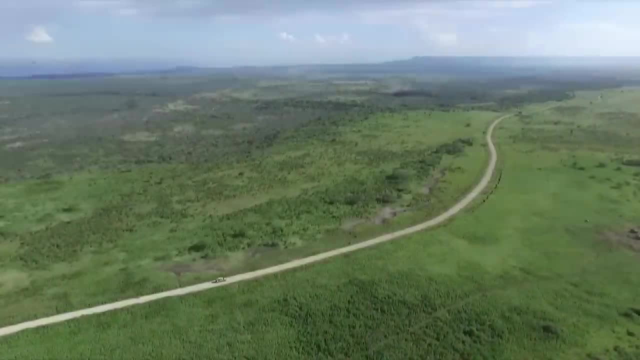 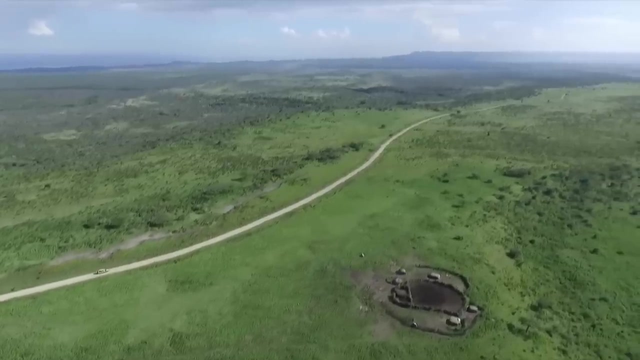 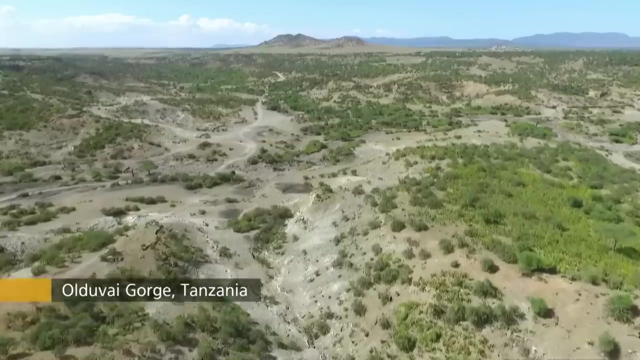 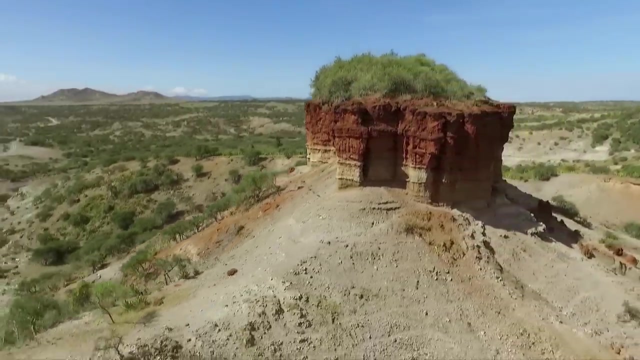 Let us look up at what we call the Mesozoic. held an ancient record of climate change. Once we thought that modern humans had gradually evolved from a single ancestor and became us. However, just now, just now, Just like other creatures, we had many branches. How did we come to know this? In 1975, Kenya, remains of Homo erectus were excavated. It was a surprising discovery because another human kind was known to already exist in this stratum. This was evidence that two different human kinds had coexisted. 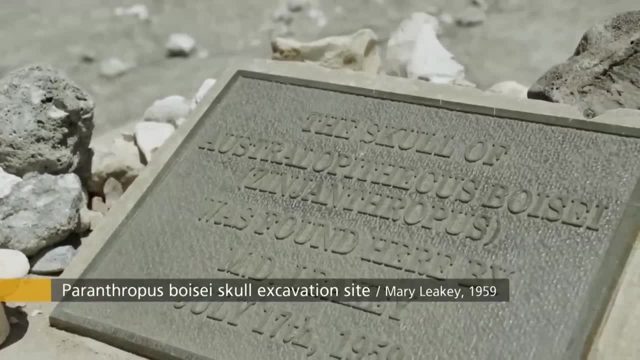 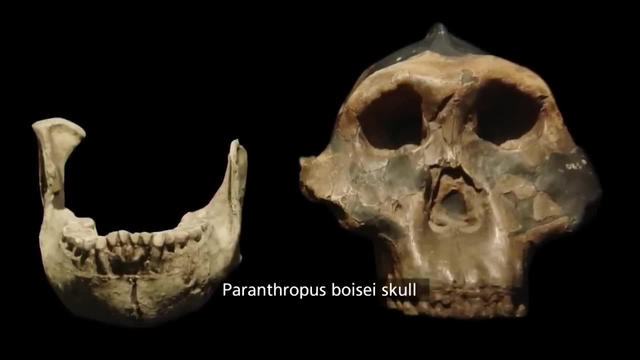 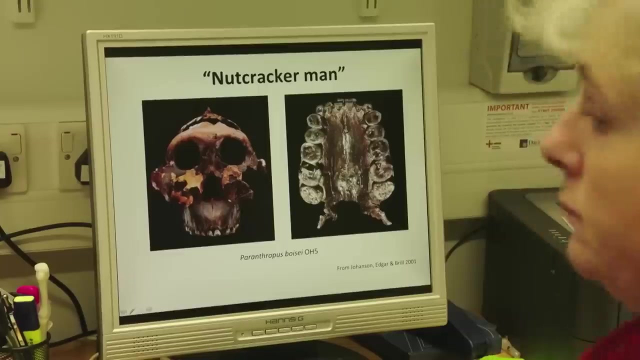 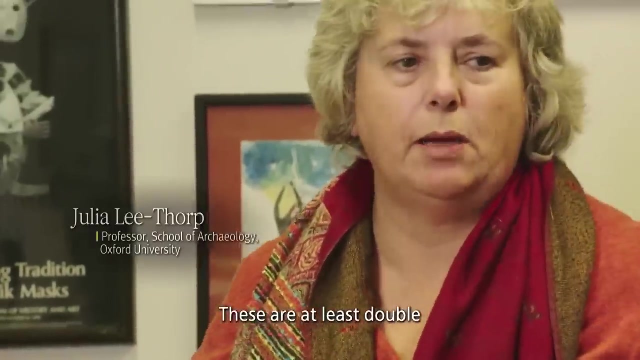 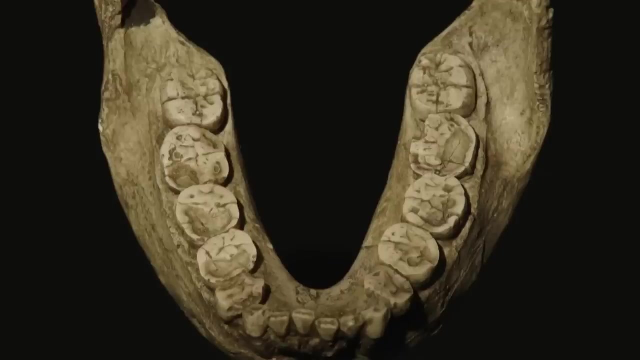 Here is the protagonist. Modern tooth molars are going to be maybe a centimeter by a centimeter, but these are at least double. so they have really very large teeth, huge teeth. Their molars were relatively huge compared to their incisors. 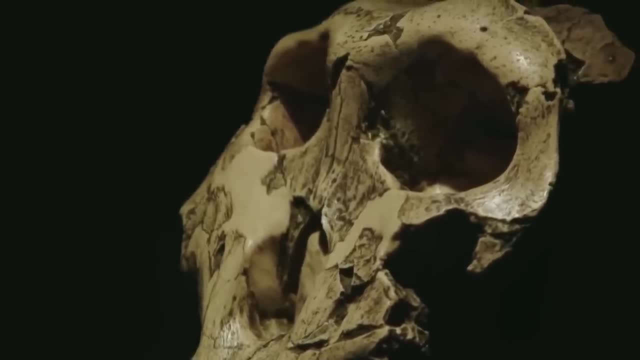 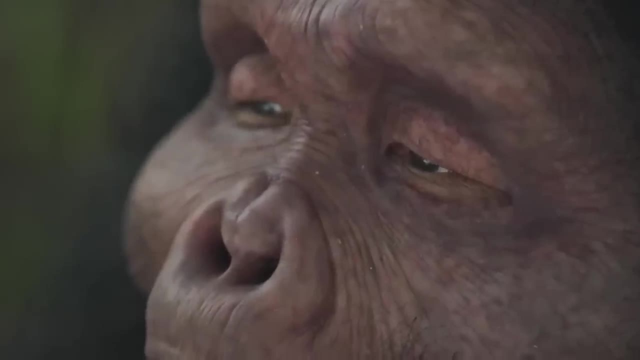 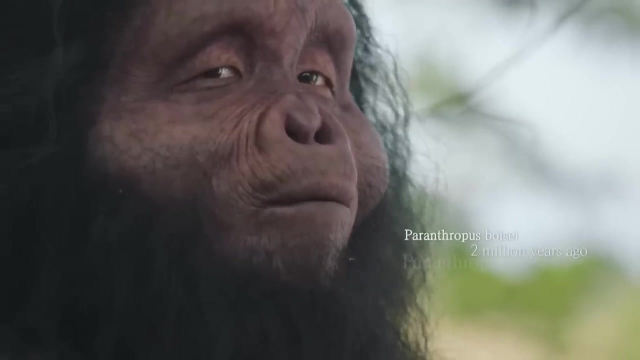 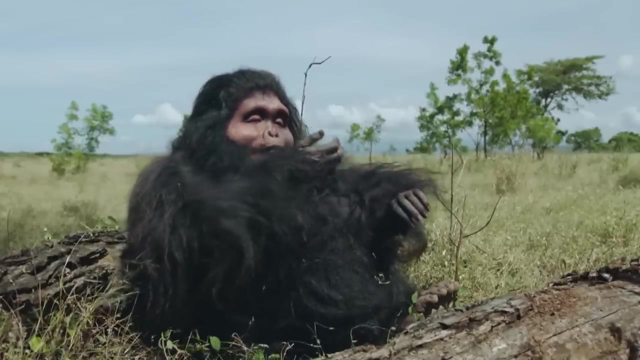 Their faces were wide and flabby. Their teeth were long and long. A human species that lived about two million years ago. The shape of their jaw gave them a nickname: the Nutcracker Man. Their brain was about one-third the size of ours. 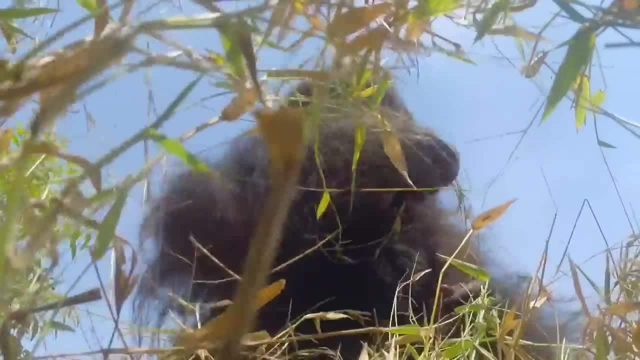 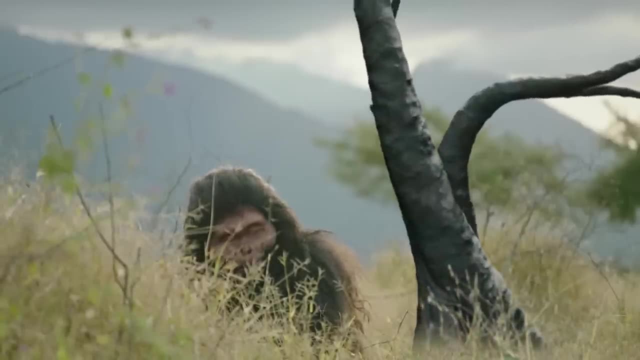 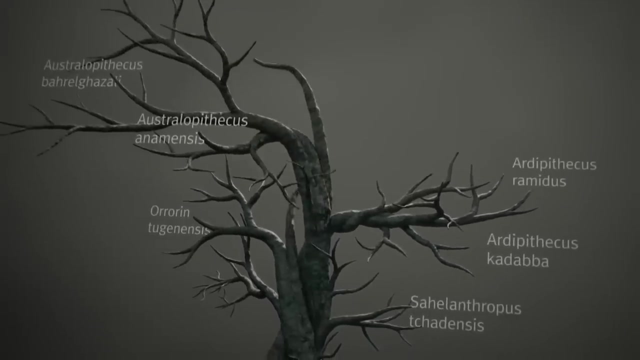 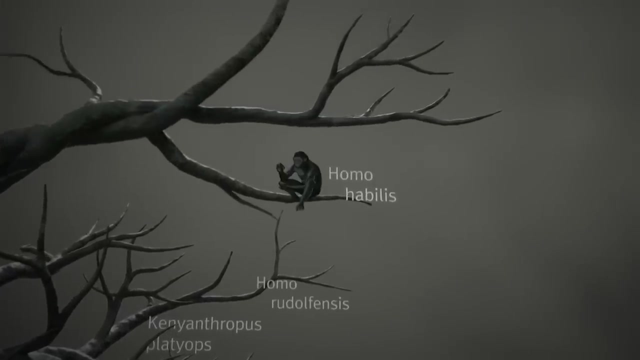 The brain was about one-third the size of ours. At that time, about five to six human species competed against one another for survival. About five million years after, since the tree of humans grew, Three human species with gracile frames- Homo habilis, Homo rudolfensis and Homo ergaster- existed in Kenya, Africa. 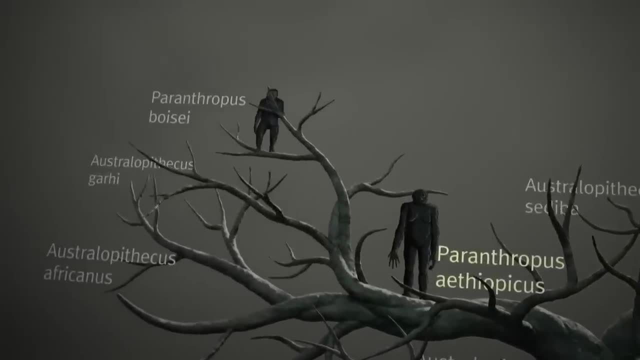 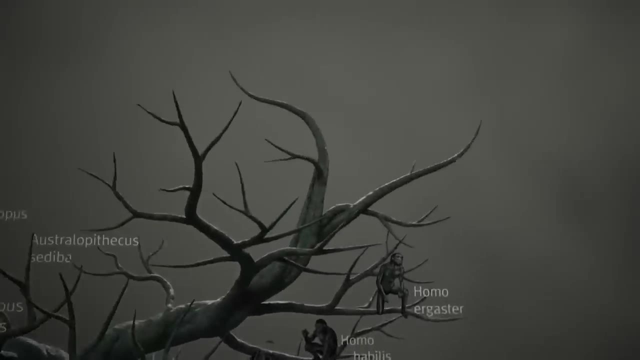 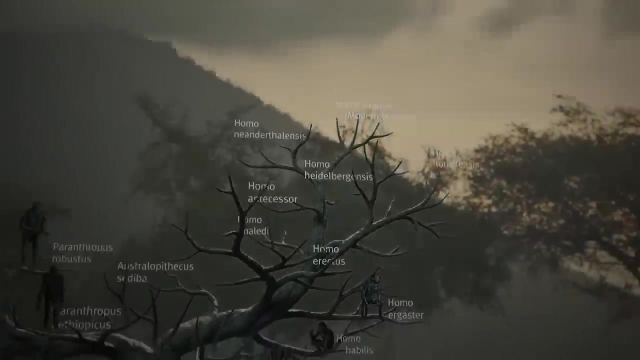 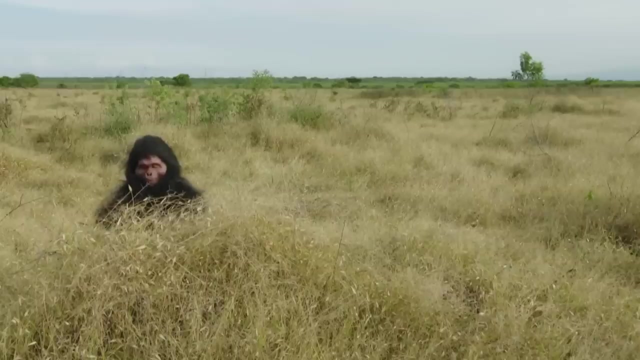 At that time, there also lived more robust species like Paranthropus boisei. We Homo sapiens were a member of the gracile species. Just like other creatures, humans have a sizable family with numerous branches. Boisei were vegetarians. 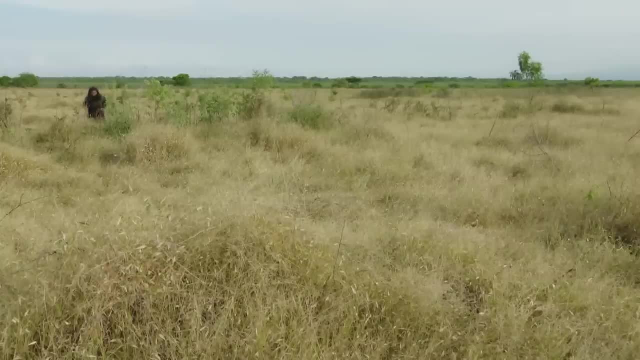 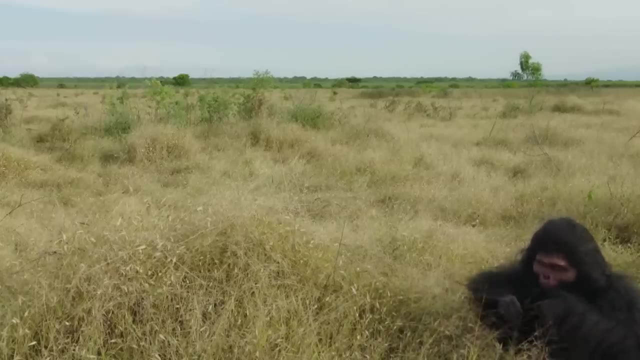 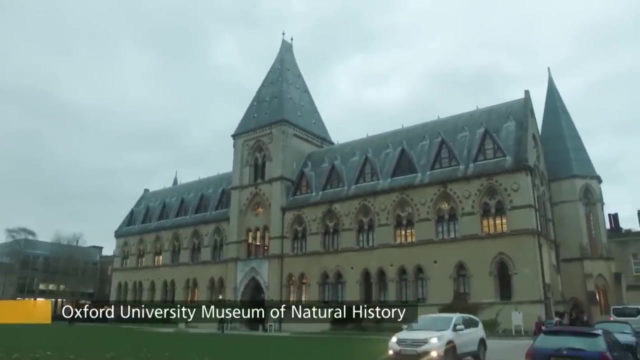 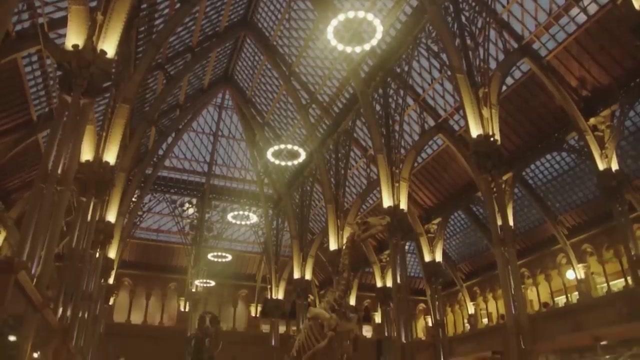 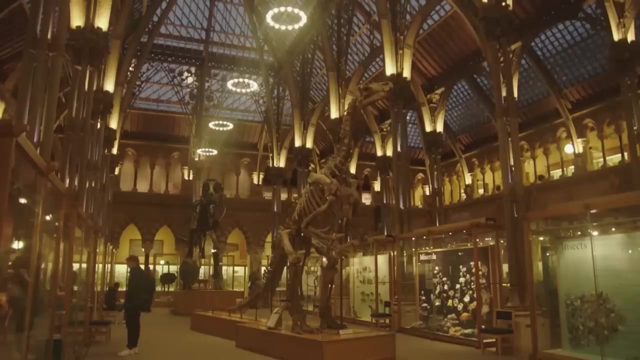 Males were 130 centimeters tall and weighed 49 kilograms on average. How did they maintain this physique? The This room preserves time which dates back two million years ago. This room preserves time which dates back two million years ago. Professor Macho uses the teeth of primitives to travel through time and space. 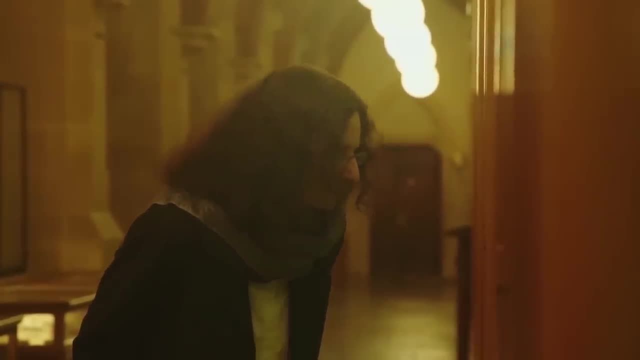 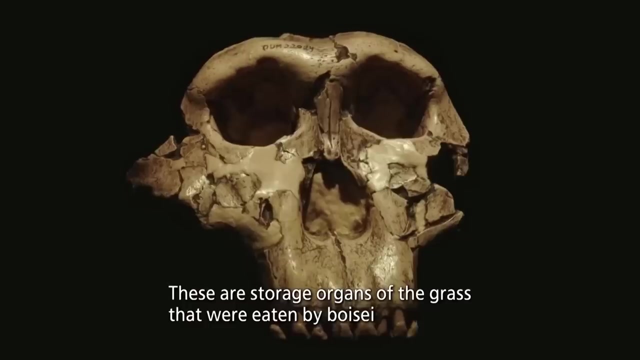 Professor Macho uses the teeth of primitives to travel through time and space. What these things are are the storage organs of grasses that were eaten by Boisei. What these things are are the storage organs of grasses that were eaten by Boisei. 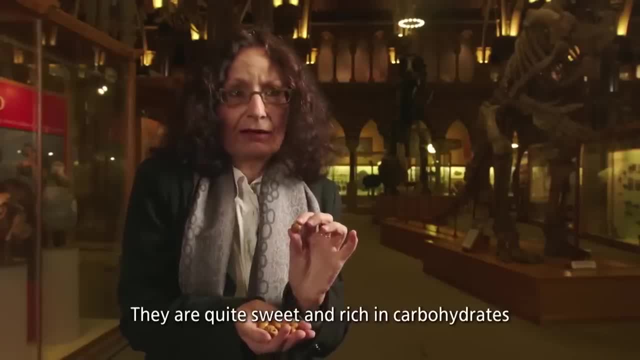 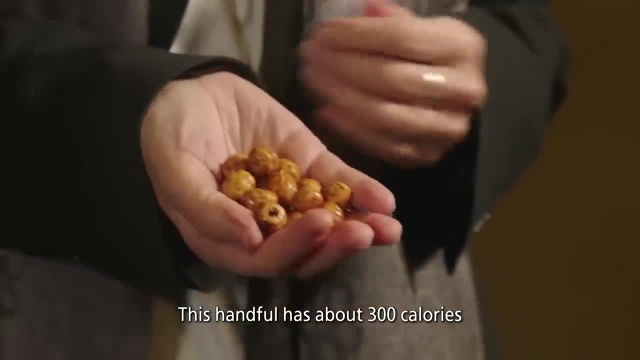 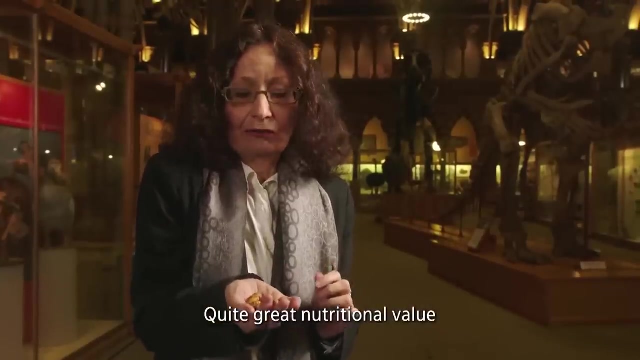 They're relatively large. They're as large as chickpeas. They're quite sweet and they're rich in carbohydrates. They're relatively large and they're rich in carbohydrates. This handful has about 300 calories, So actually quite great nutritional value. 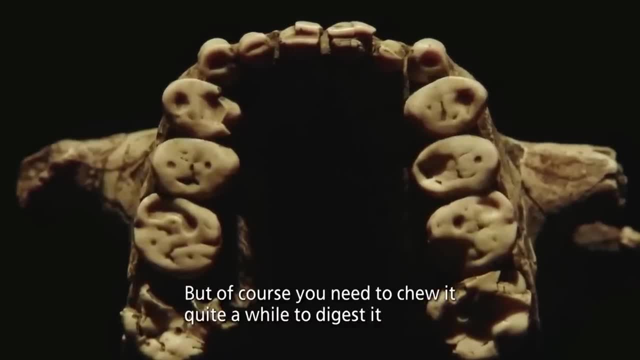 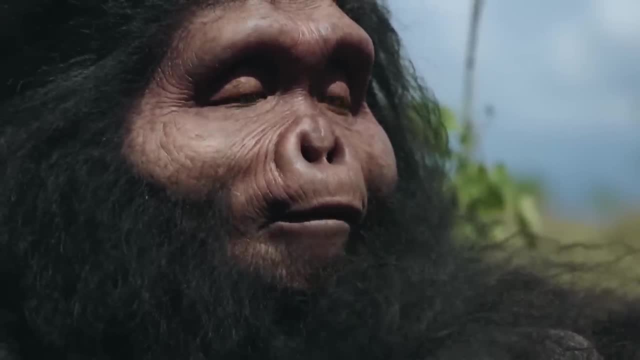 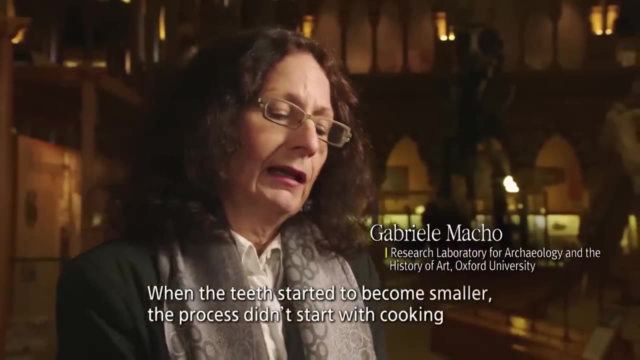 But of course you need to chew it quite a while to digest it. Their strong jaw and wide face were developed because they had to chew excessively When the teeth started to become smaller. the process didn't start with cooking, but it started with the emergence of hormone. but it started with the emergence of hormone And generally we associated with habitual consumption of meat And generally we associated with habitual consumption of meat because meat is high in quality. because meat is high in quality, You don't need to eat that much. 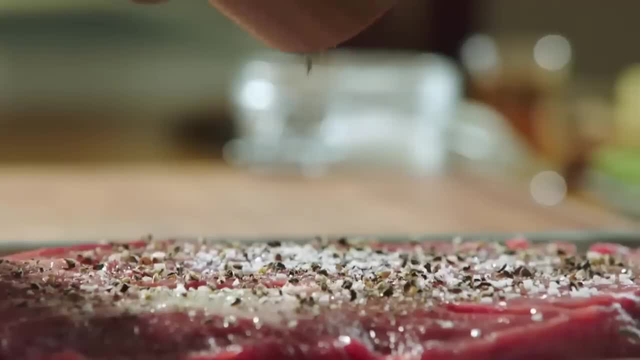 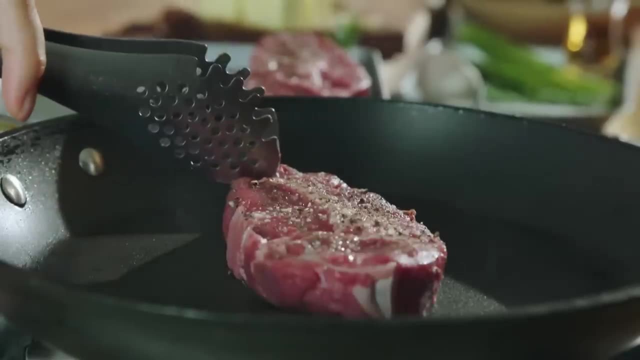 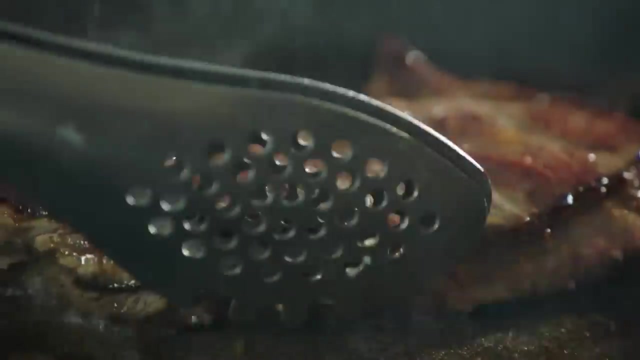 What did eating meat mean to humans? What did eating meat mean to humans? First, hunting became a necessity. They had to devise complicated strategies compared to when eating plants. Consequently, their brains were enlarged. Mainly, the brain is a chunk of fat. 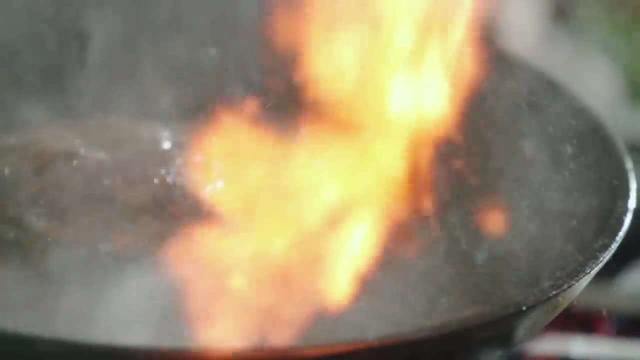 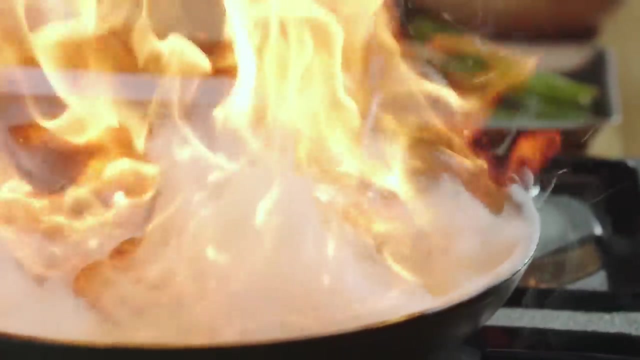 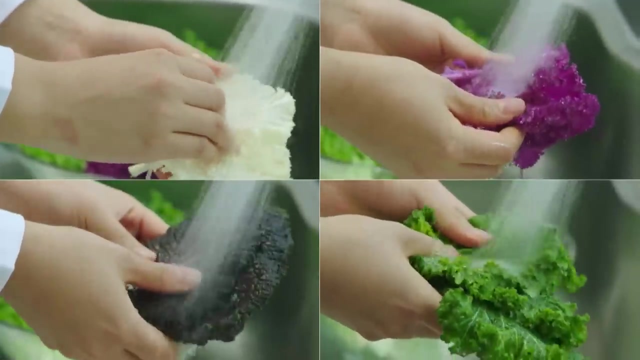 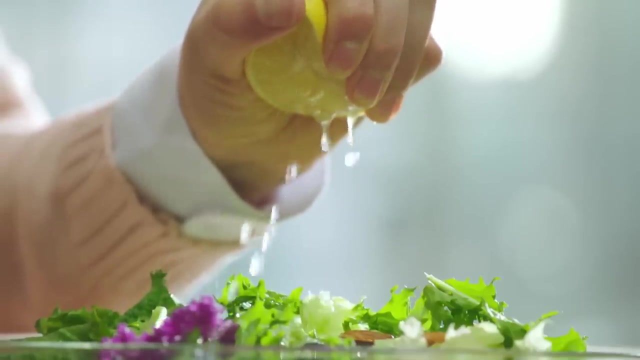 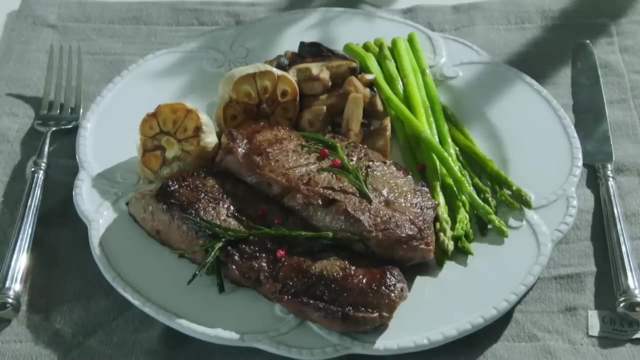 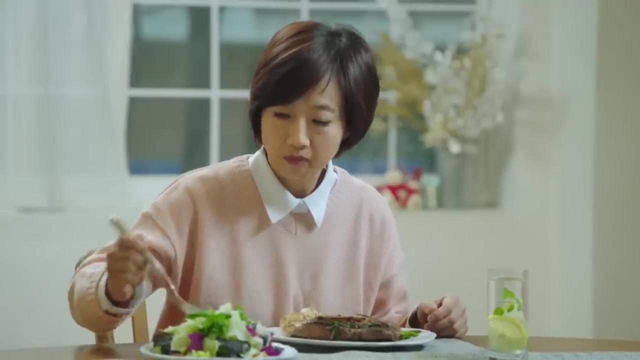 It requires an extreme amount of nutrients To consume the same calories. substantial amount of grass needs to be consumed, just like Boisei. Humans can only consume a limited amount of energy. Naturally, the brain has no choice but to compete with other organs for energy. 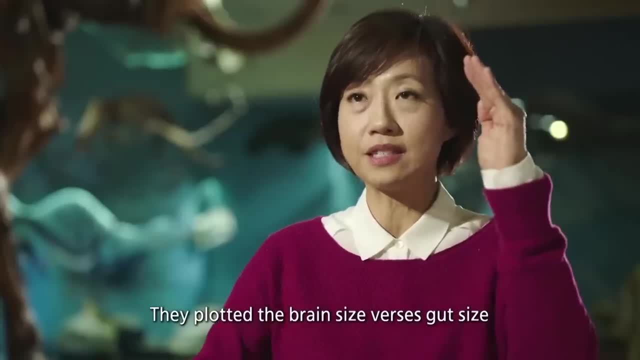 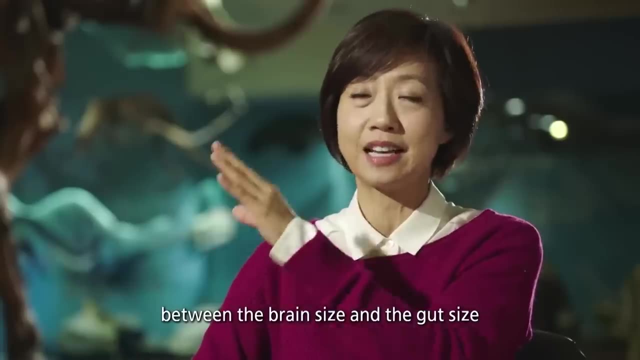 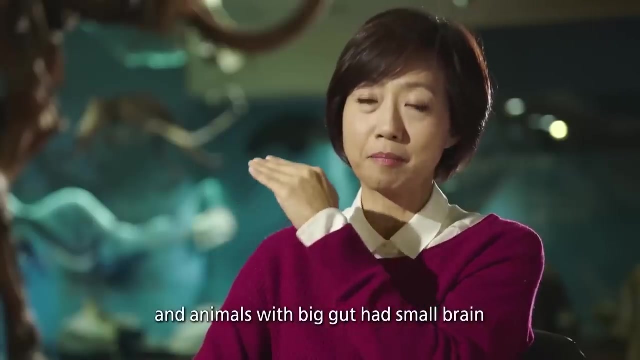 They plotted the brain size versus gut size and showed that there was indeed an inverse relationship between the brain size and the gut size. In other words, animals with big brain had small gut and animals with big gut had small brain. So there was the compatible data. 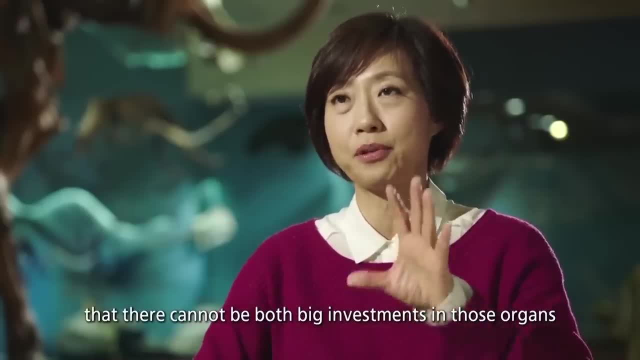 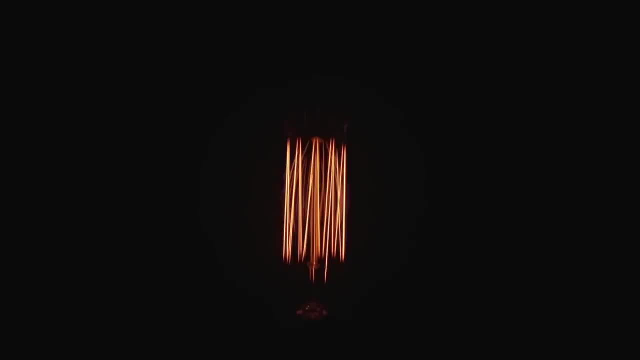 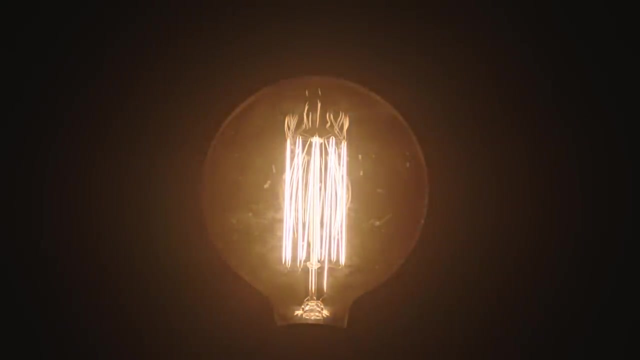 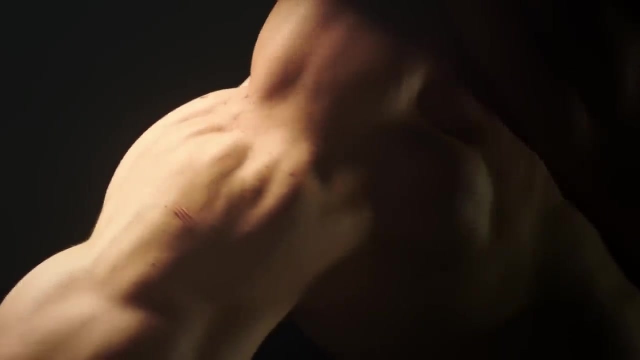 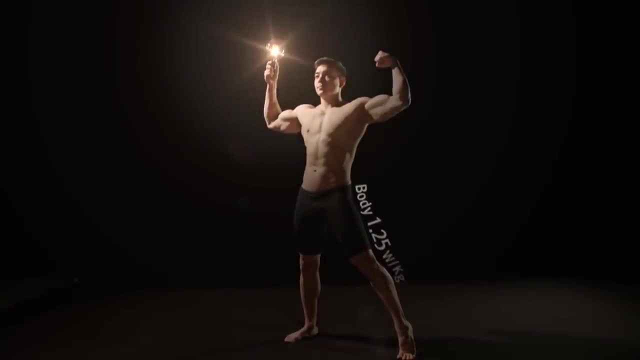 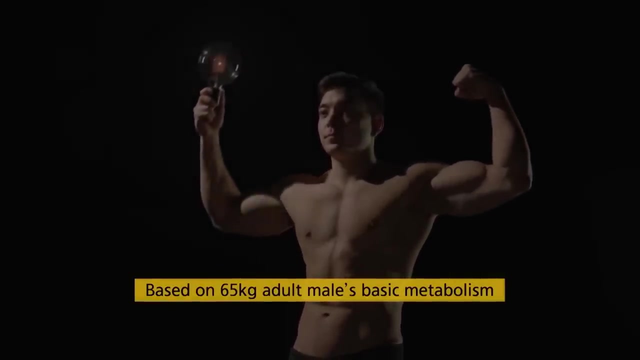 So there was the compatible data. So the compatible data To show that there cannot be both big investment in those organs. Our bodies consume 1.25 watts of energy per kilogram on average. Muscles use 0.5 watts per kilogram. 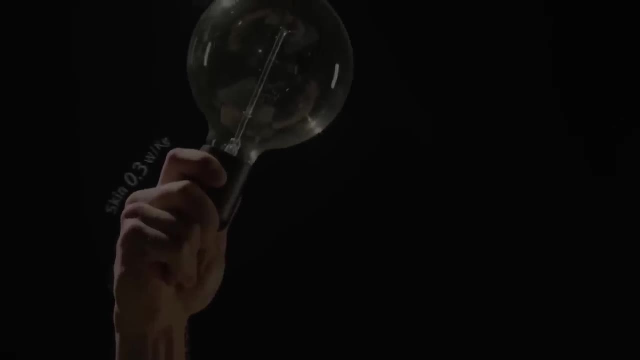 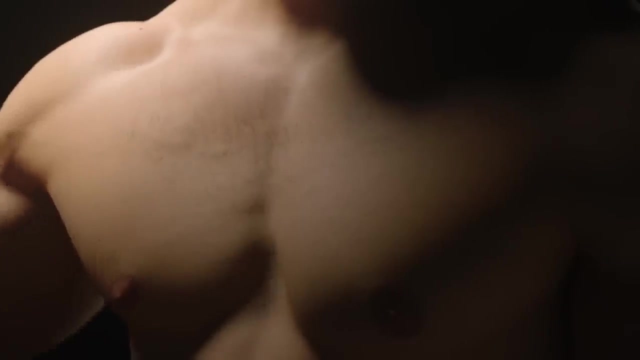 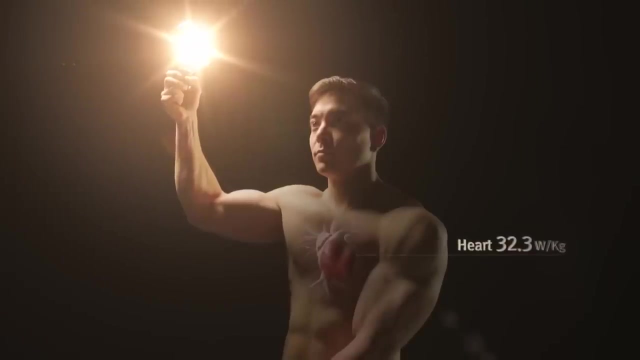 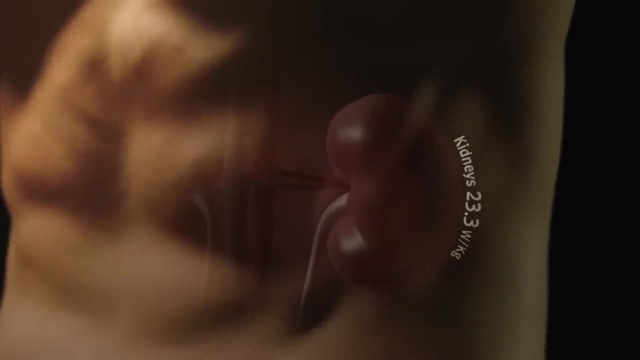 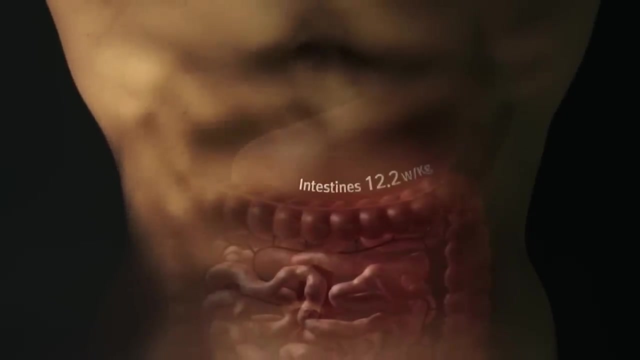 The skin 0.3 watts. It accounts for a large space, but it is energy efficient. Next, there are the more expensive tissues. The heart uses 32.3 watts, The kidneys 23.3 watts, The intestines 12.2 watts. 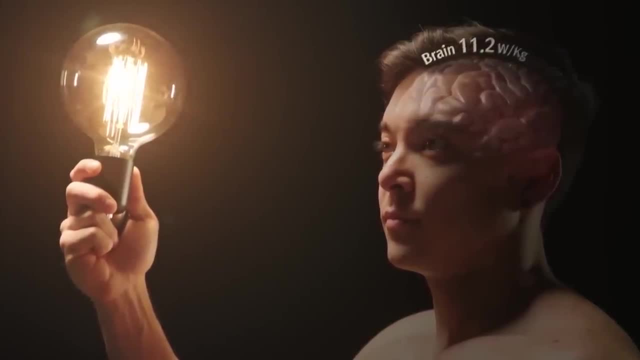 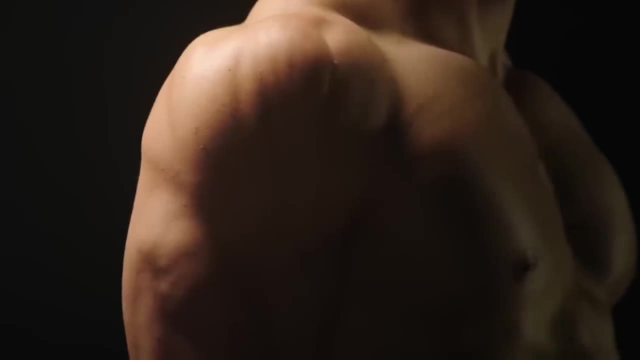 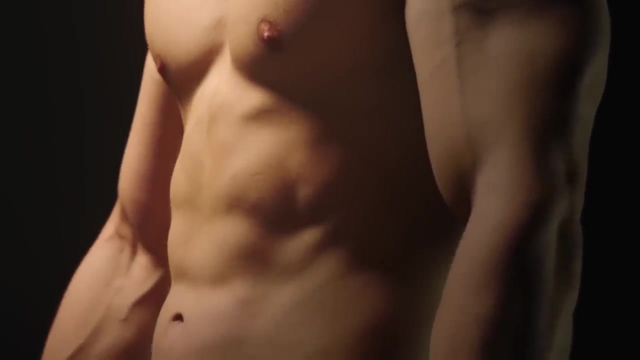 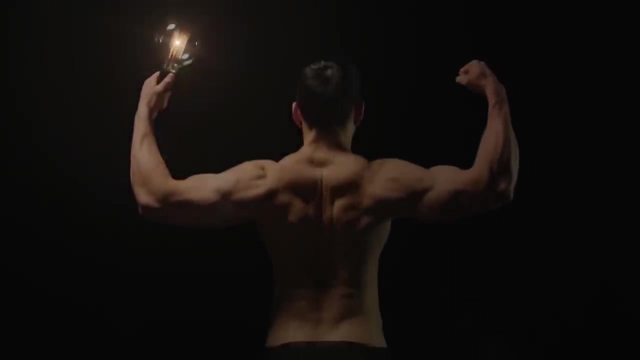 And the brain 11.2 watts. The heart and kidneys have to maintain their sizes to fulfill their functions. However, the intestines can become shorter if the quality of diet is improved. When humans began eating meat, they evolved to have shorter intestines and larger brains. 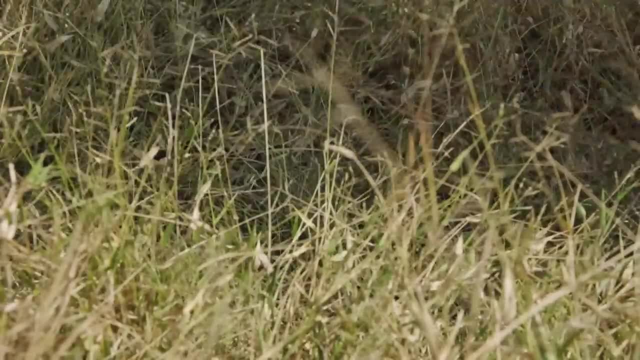 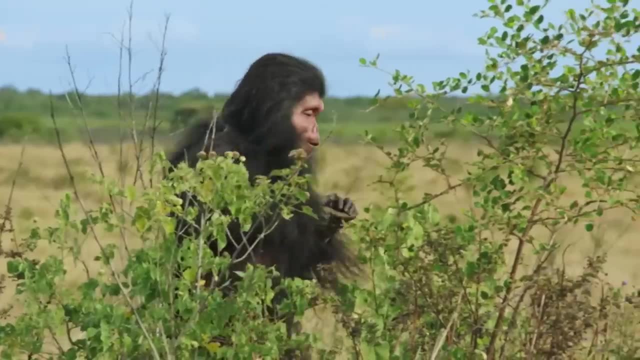 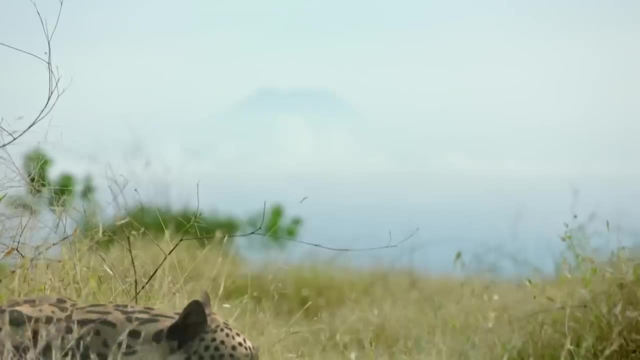 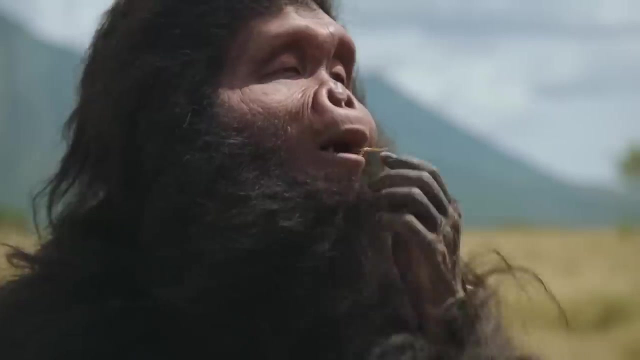 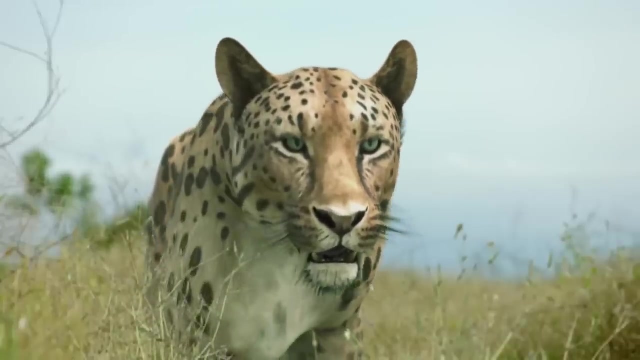 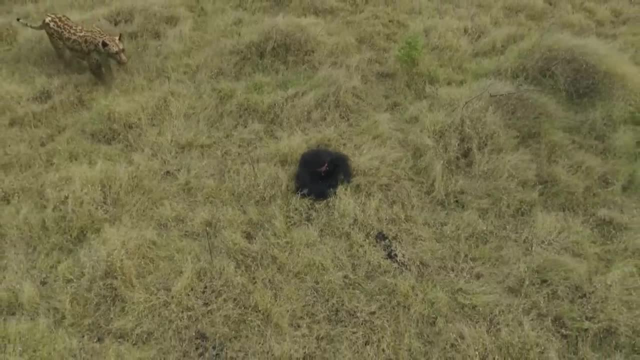 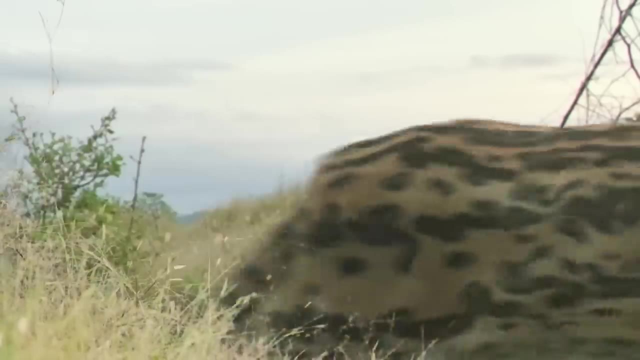 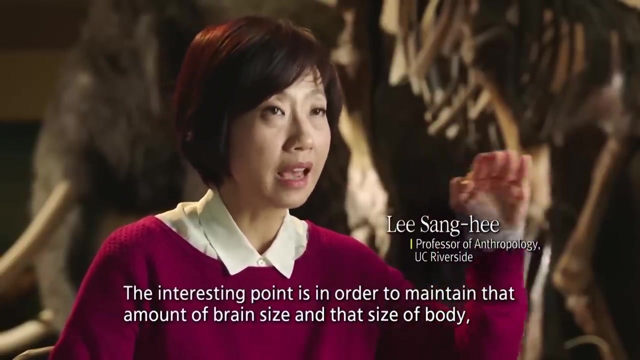 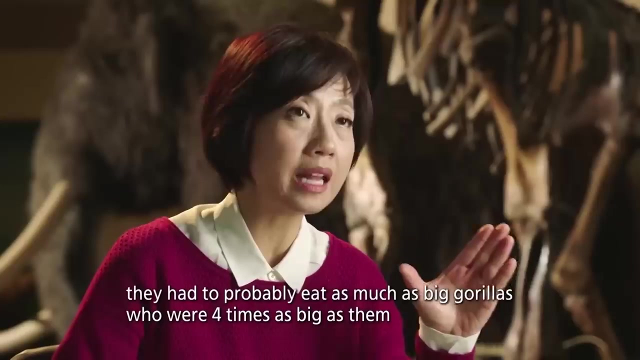 A life spent eating just to gain enough energy to find more food, Living slowly, always in search for pastures. Was this a good strategy? The interesting point is, in order to maintain that amount of brain size and that size of the body, they had to probably eat as much as a big gorilla, who were four times as big. 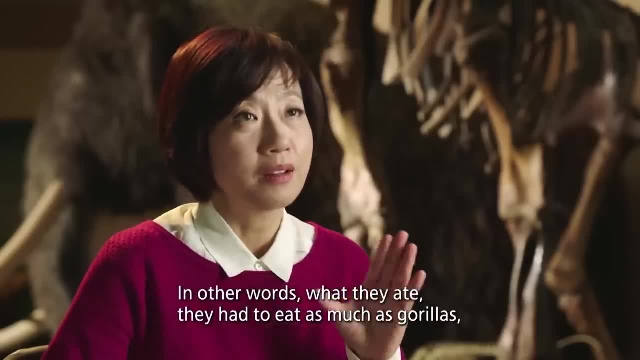 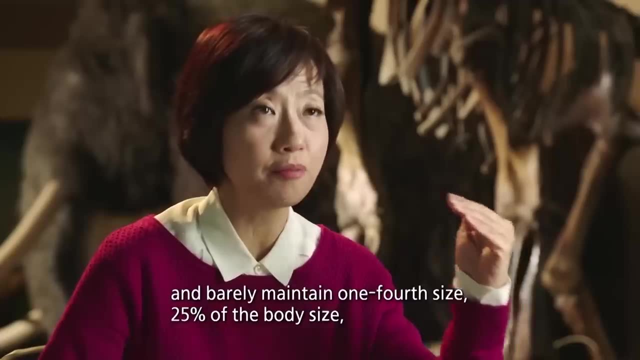 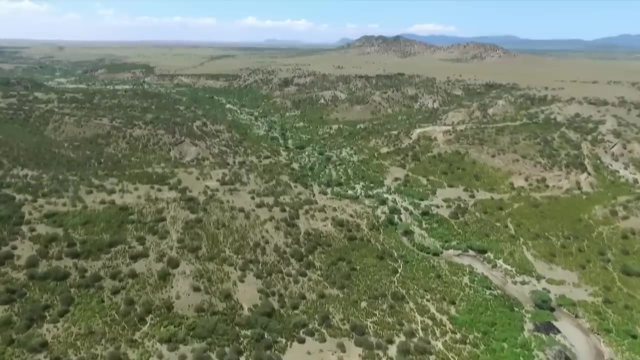 as them, In other words, what they ate. they had to eat as much as gorillas and barely maintain one fourth size, 25% of the body size, meaning the quality of their food was extremely low. The land where both robust and grassy humans 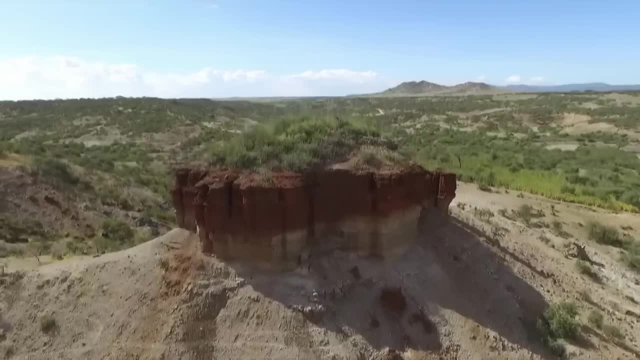 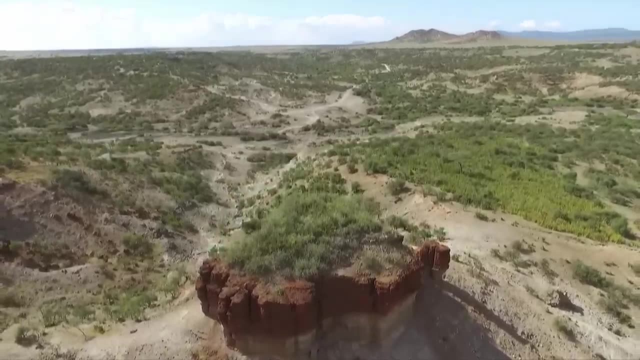 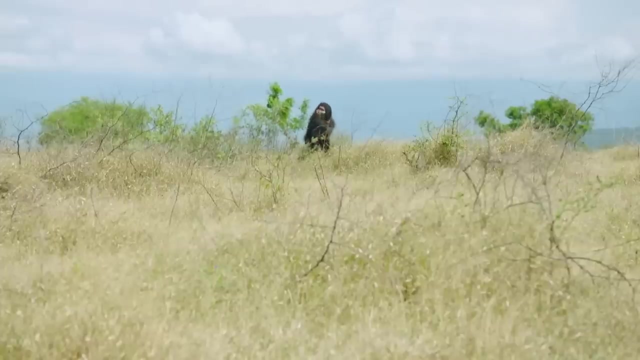 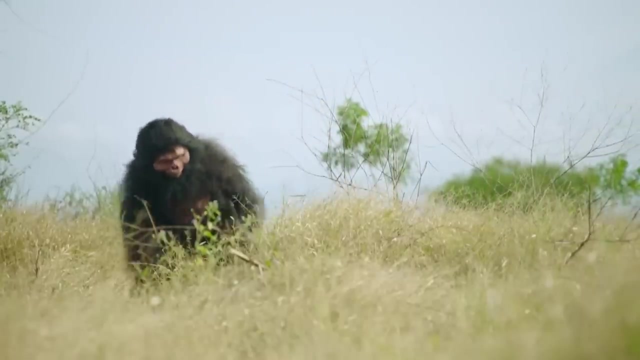 roamed. A battle was fought between the brain and the stomach. Boisei, which chose the stomach, may not have been unfortunate, While the grassy humans, who chose meat, starved without food, they thrived for about a million years. The land where both robust and grassy humans lived was extremely low. 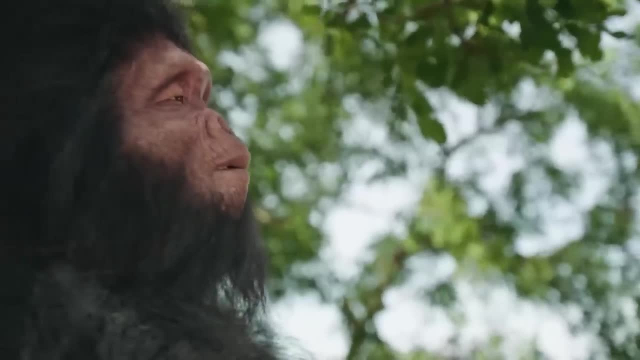 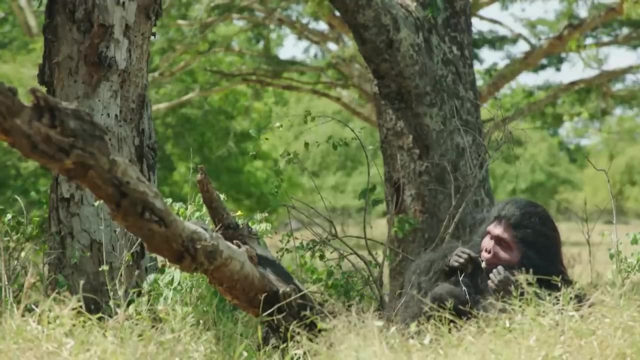 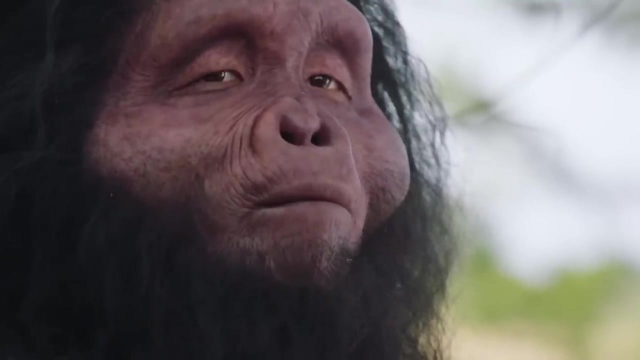 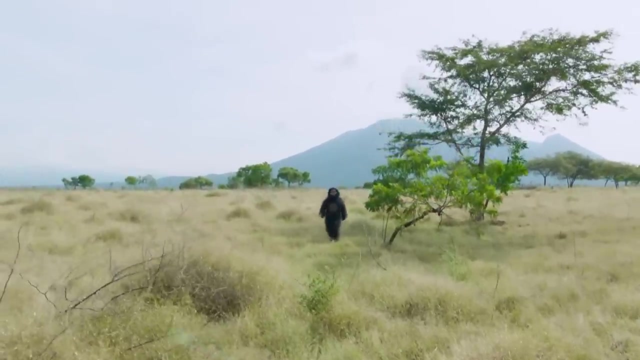 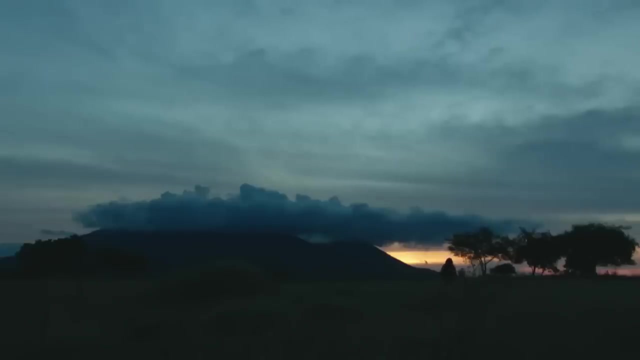 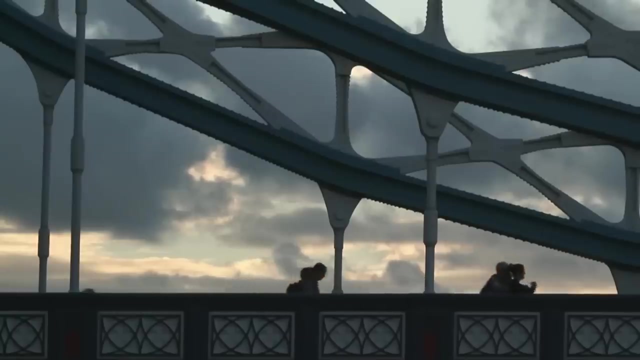 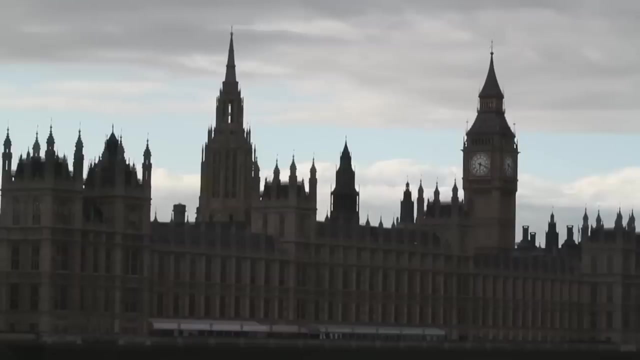 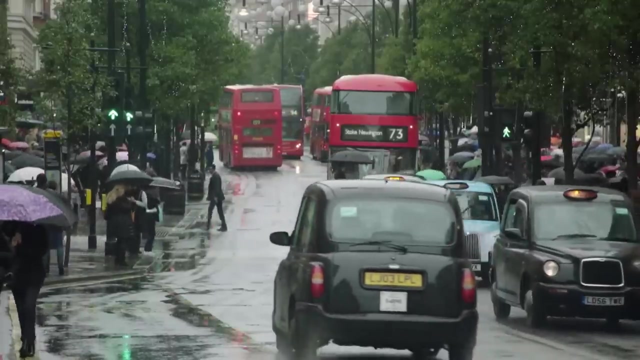 The land where both robust and grassy humans lived was extremely low. The land where both robust and grassy humans lived was extremely low. Fossils show that Boisei disappeared approximately 1.2 million years ago. communist, We do not have to eat all day like Boisei. 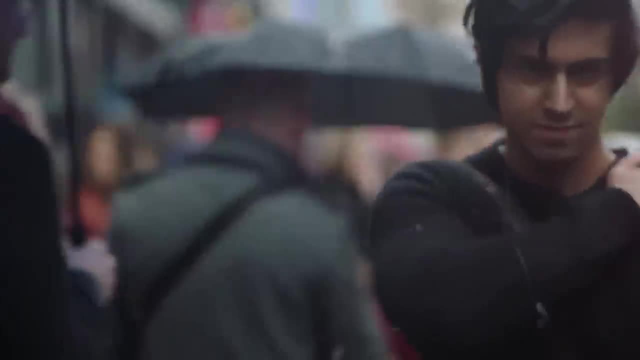 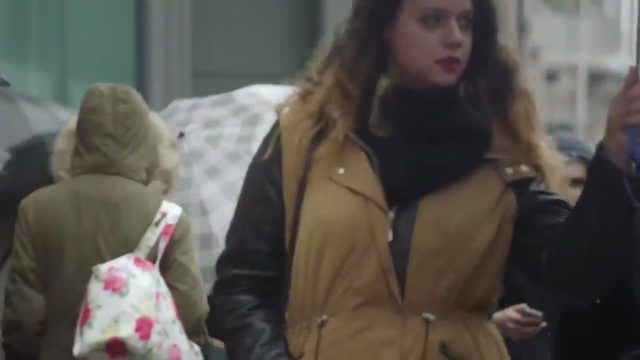 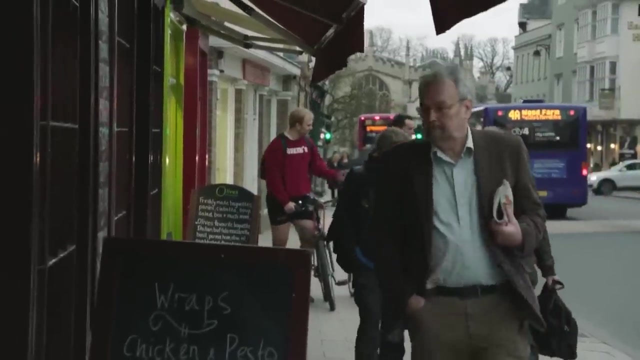 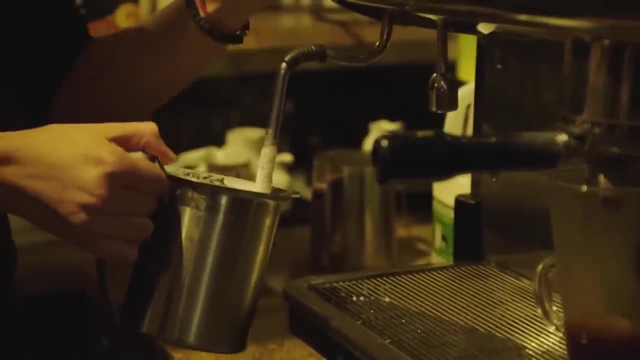 Just like Homo heidelbergensis, we are the most intelligent creatures on this earth, With greater ego than any other species. we also live in communities. It seems like much has changed, but most remain similar: A latte, a large latte. 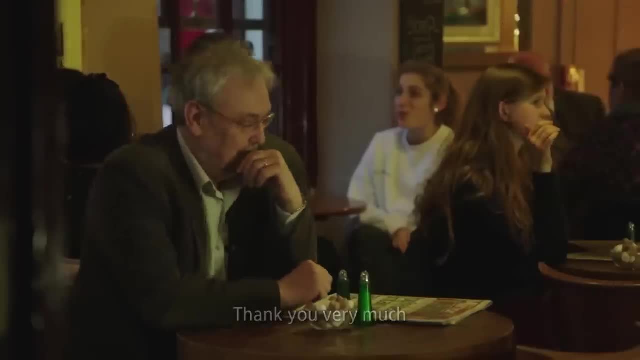 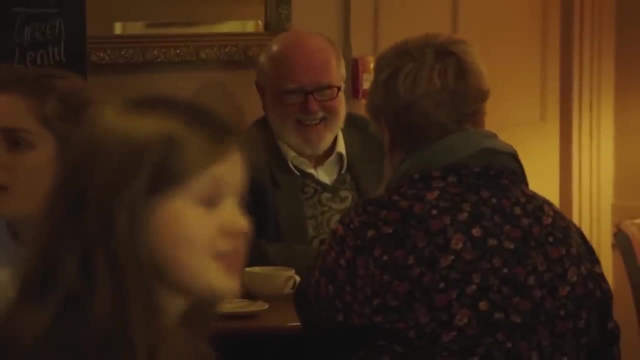 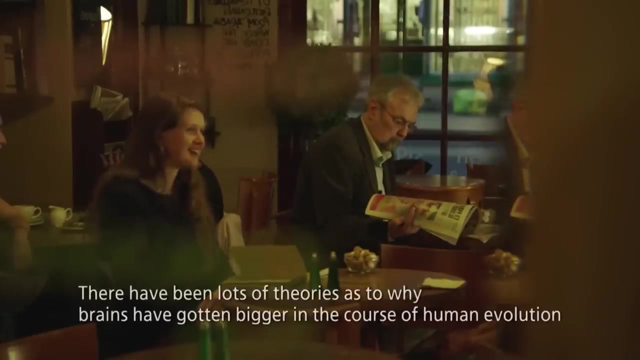 Thank you very much. Professor Robin Dunbar is interested in why the human brain grew bigger. Instead of studying bones and rocks, he conducts cognitive experiments. There have been lots of theories as to why brains have got bigger in the course of human evolution. 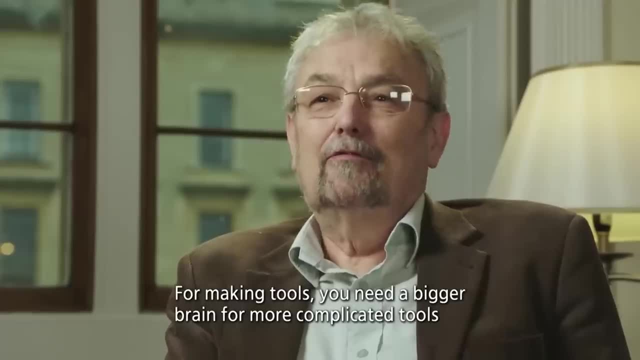 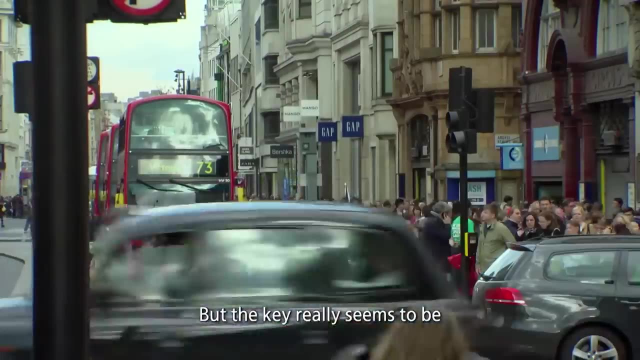 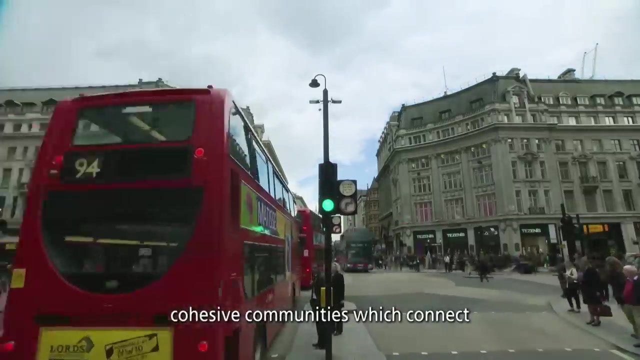 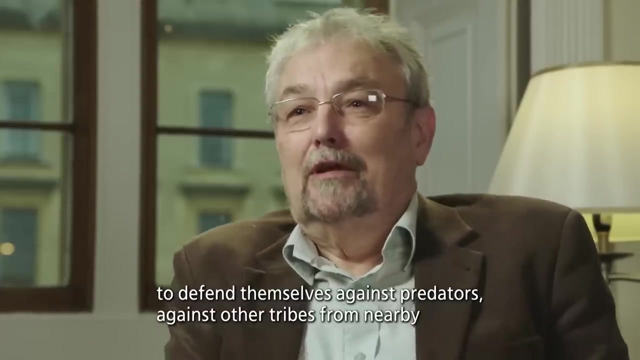 For making tools. you need a bigger brain for more complicated tools, perhaps for meat eating, but the key really seems to be to be able to create large communities which are bonded together, cohesive communities which can act to defend themselves against predators, against other tribes from nearby. 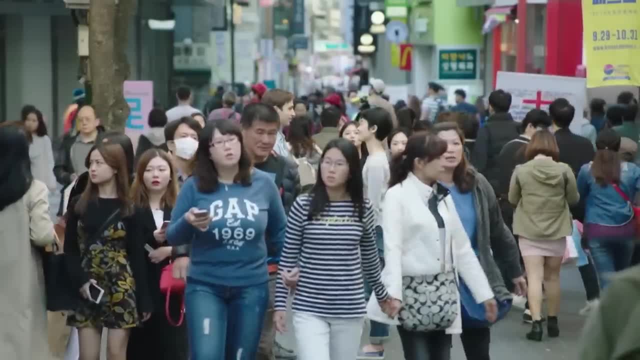 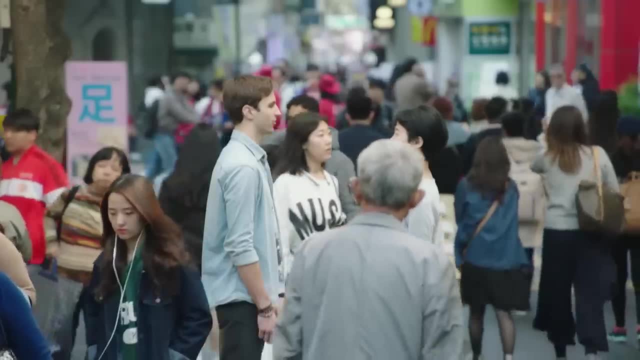 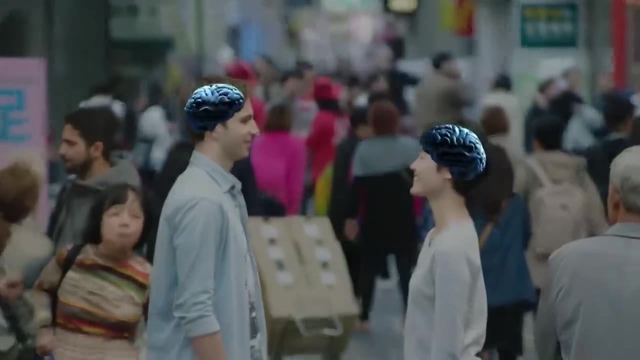 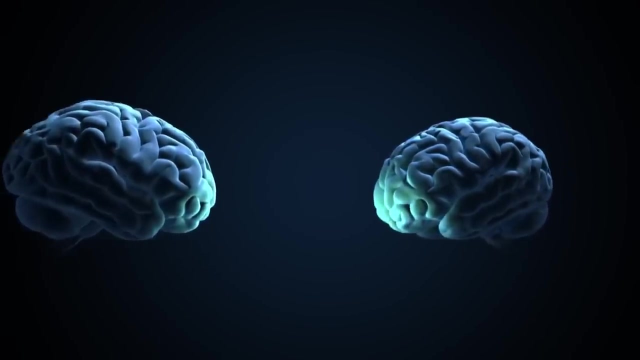 Apes formed groups to stand up against predators. The size of these groups was correlated to the size of the bones, The size of the brain. This applies to humans as well. The orbital frontal cortex is a part of the frontal lobe located close to the eye. 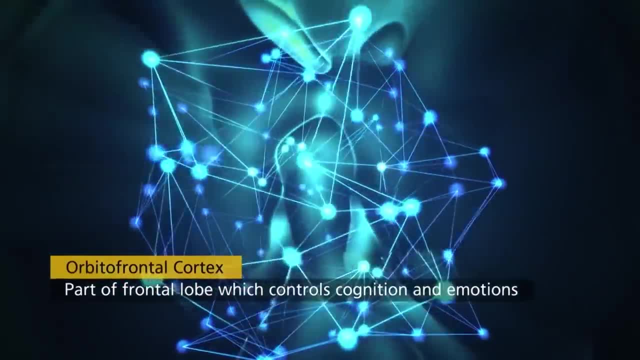 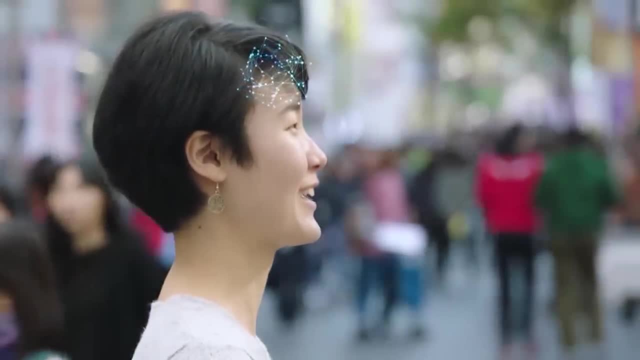 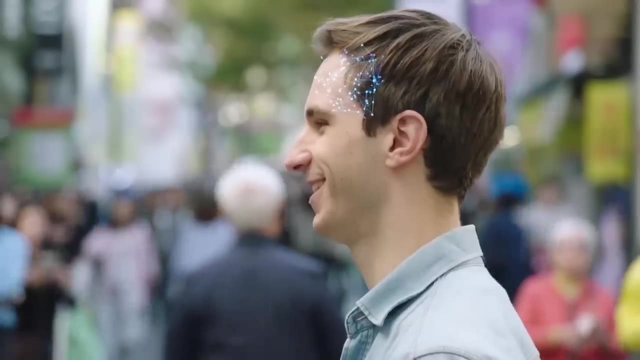 The larger the group which a person interacts with, the larger the orbital frontal cortex becomes. People with larger orbital frontal cortex have a higher desire to contact a greater number of people within the same time. We all want to communicate with others and make sense of them. 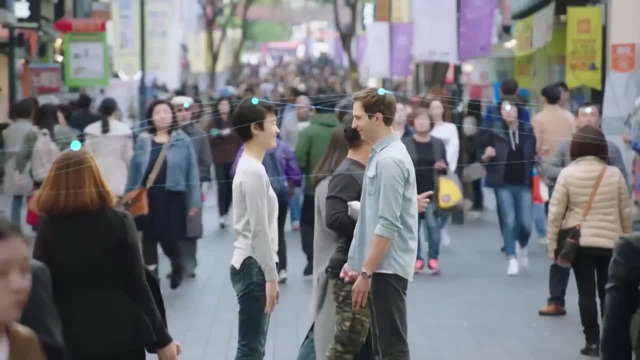 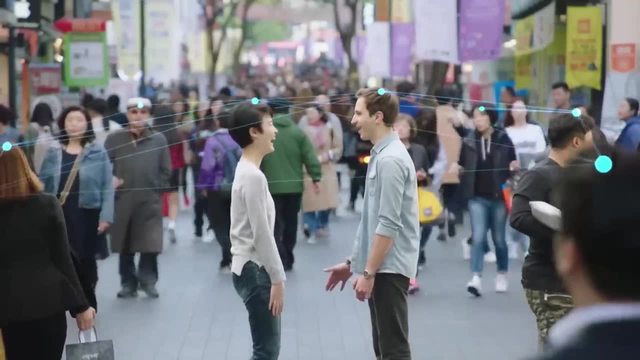 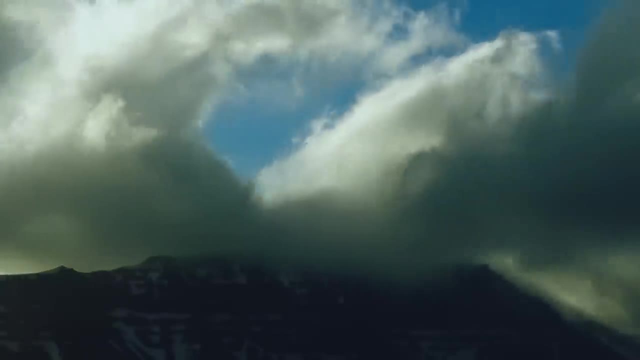 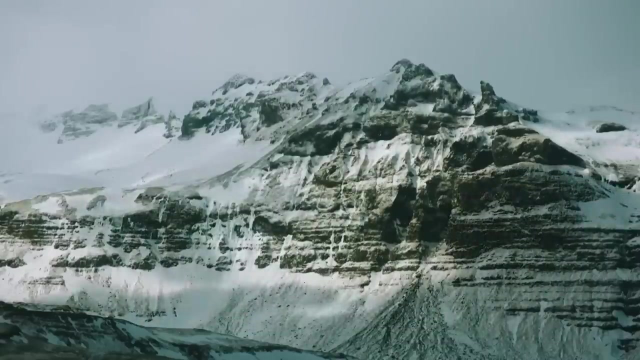 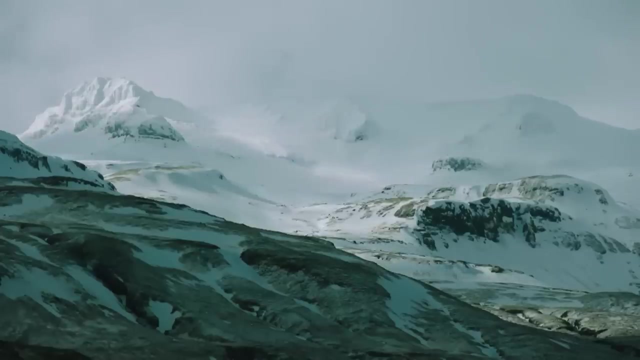 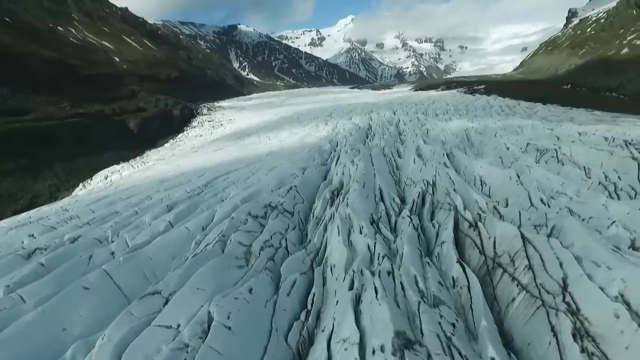 We are a species that overcomes the limitations of our body through forming relationships. Groups are skins that hold mankind together. The Now we are at the era when formation of groups determine the survival of humanity. The Earth enters its last glacial epoch. 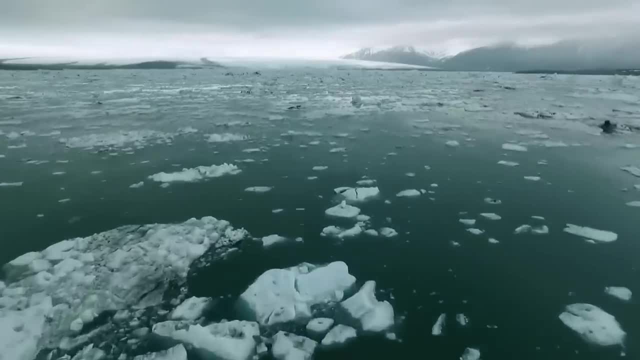 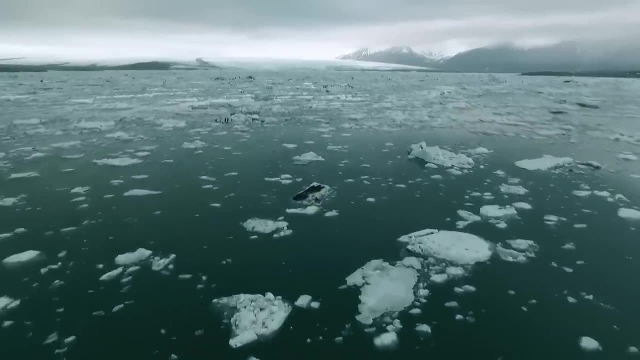 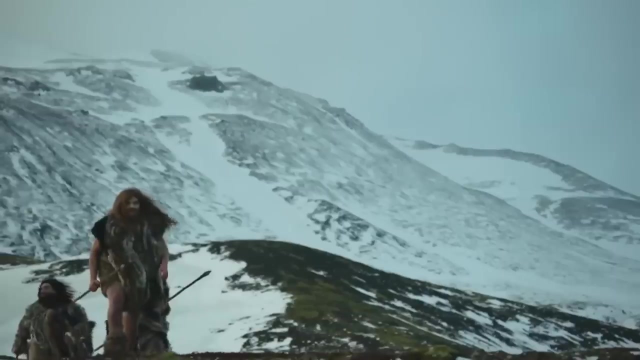 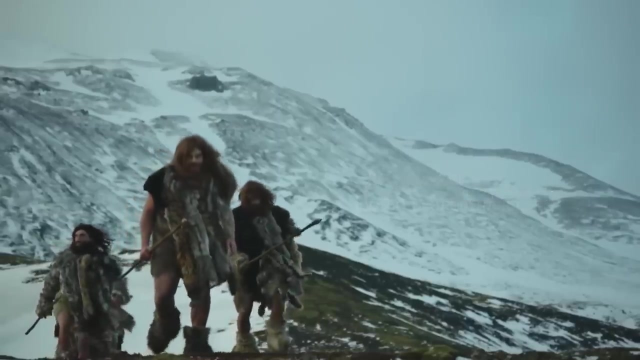 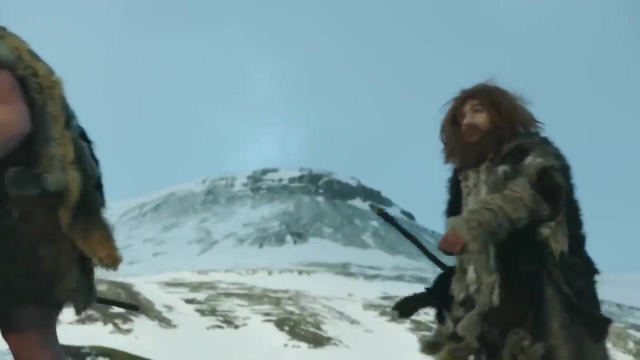 There was a human species which lived in this unforgiving coldness. They were Neanderthals, who appeared about 300,000 years ago. 100,000 years later, we Homo sapiens would appear and compete with them. 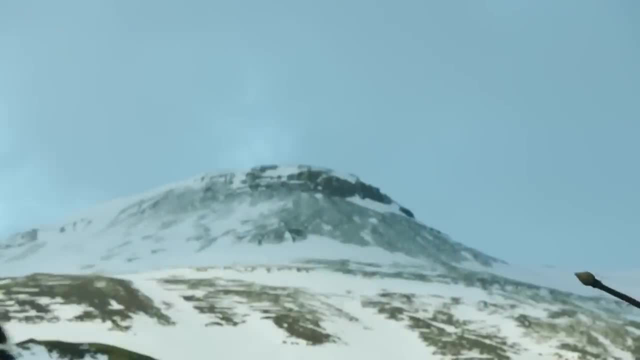 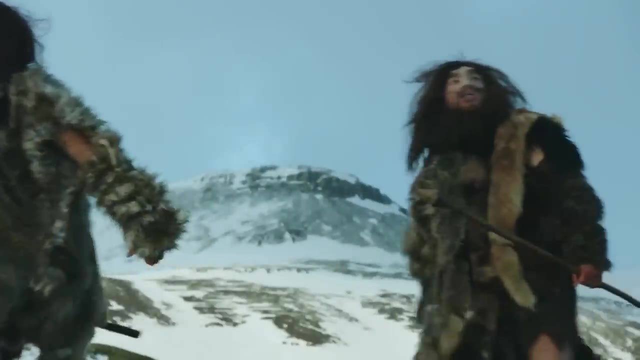 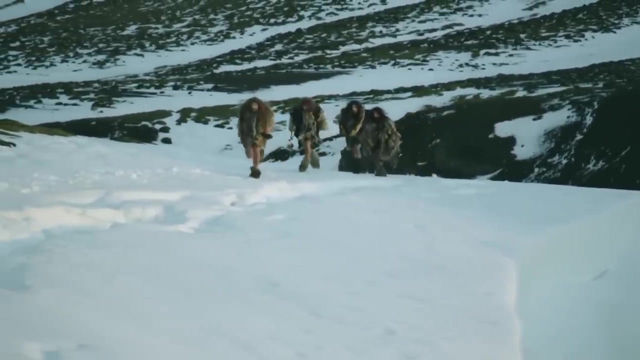 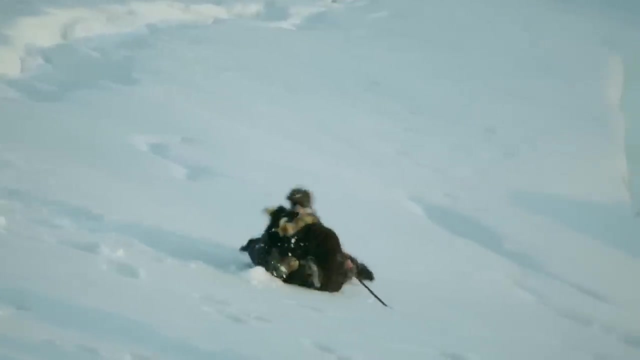 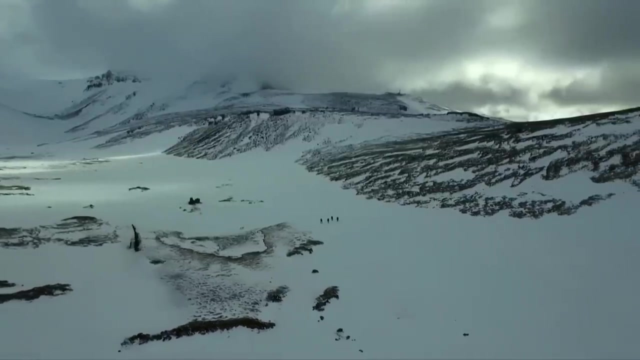 They had larger brains than us. At most, they lived about 30 to 35 years. They had short lifespans and led a busy life moving from place to place. Although their entire population never exceeded 70,000,, they spread across the frozen continent. 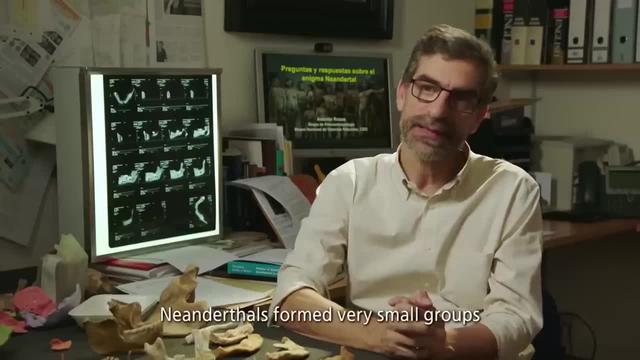 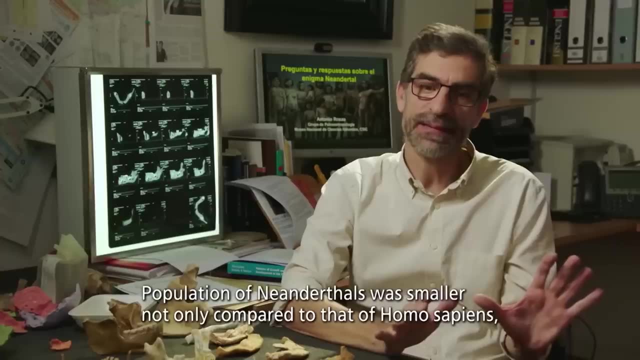 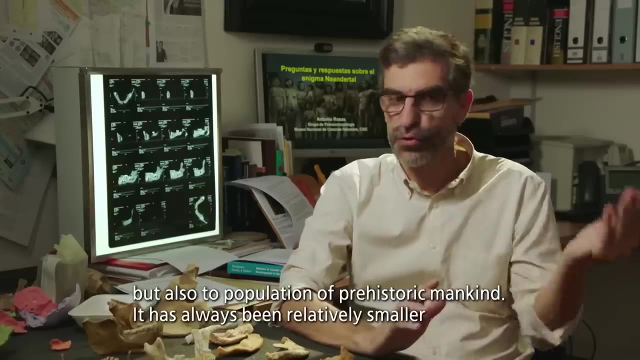 Neanderthals, we know, were a group of people who were very small. In fact the Neanderthal population in general is much smaller if we compare it, of course, with the Sapiens population, and even in prehistoric times, 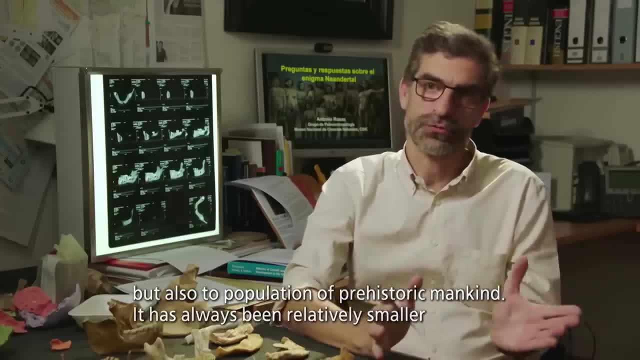 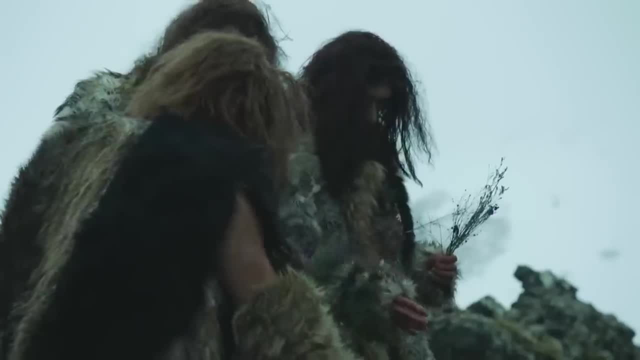 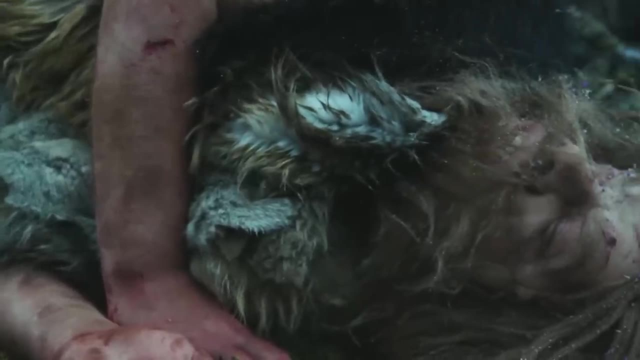 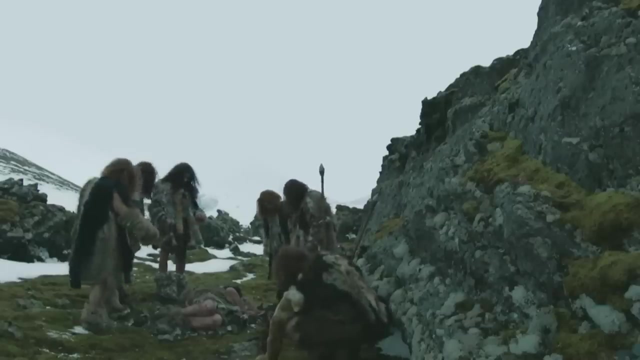 In other words, there were very few Neanderthals in the Neanderthal population. Living in harsh climates, they understood the importance of each other well. Funerals were held for the dead. Could it have been because of the miserable reality? 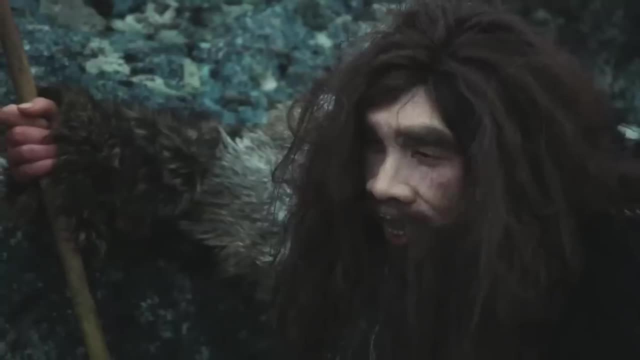 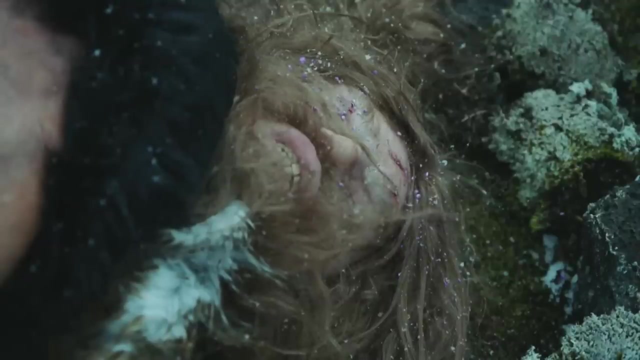 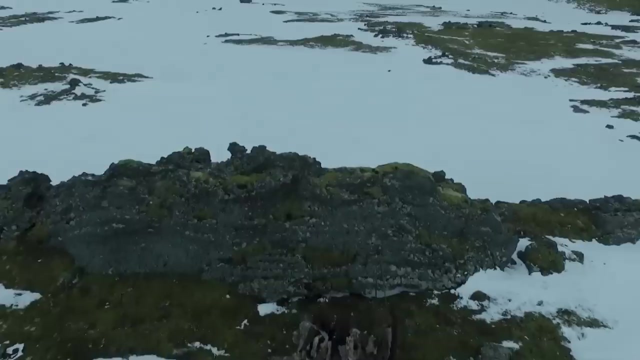 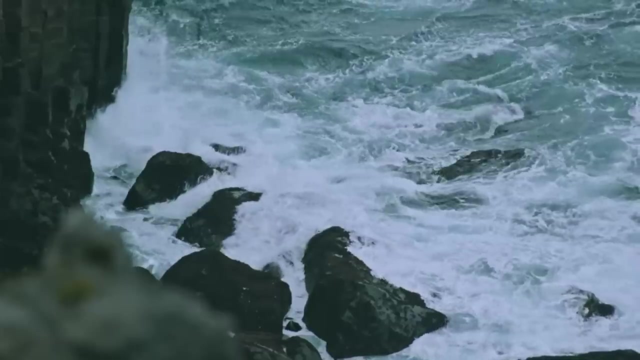 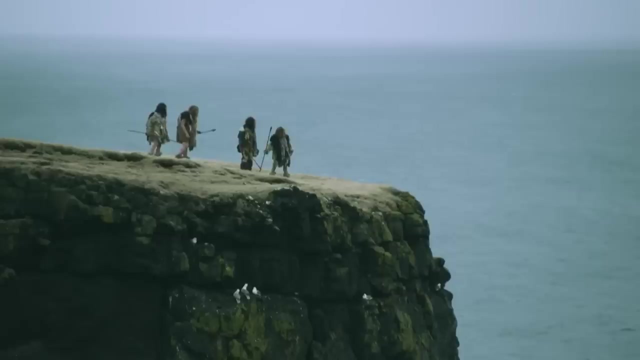 They knew feelings of grief and loss. Although their day-to-day lives were filled with hardships, they knew deeper meanings in life. Like us, they were curious about what lies beyond death. Perhaps they had developed burial rituals faster than we had. They acknowledged the loneliness better than anyone else. 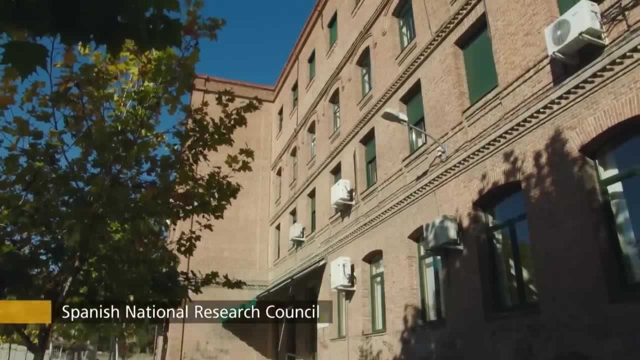 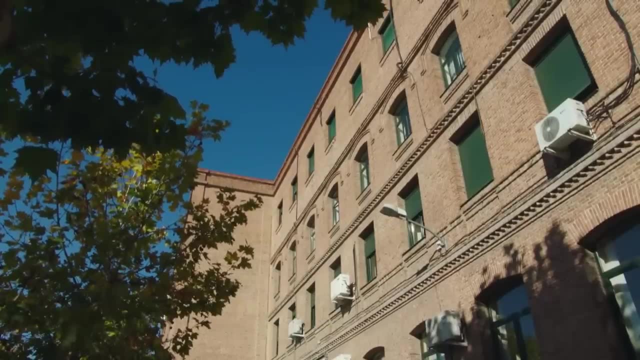 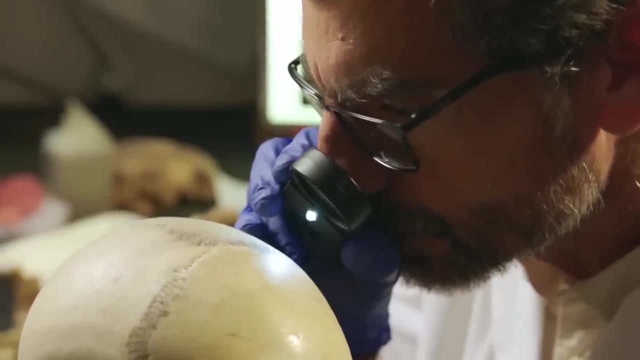 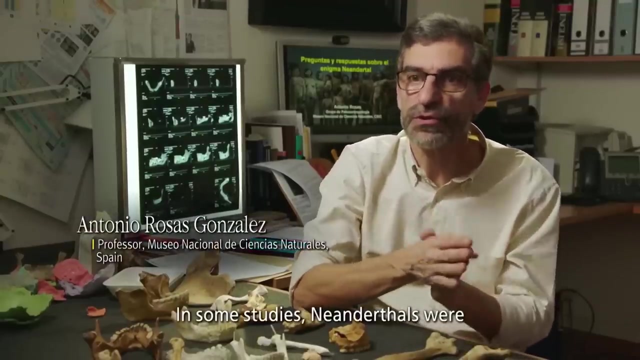 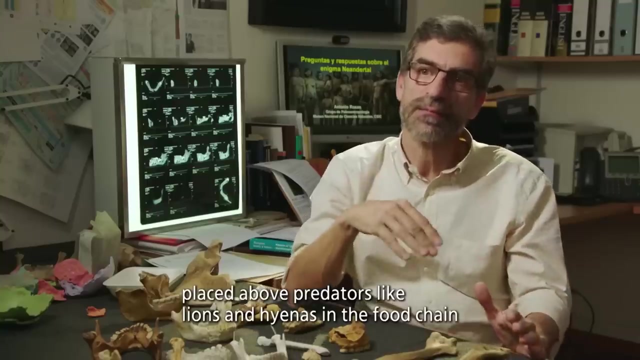 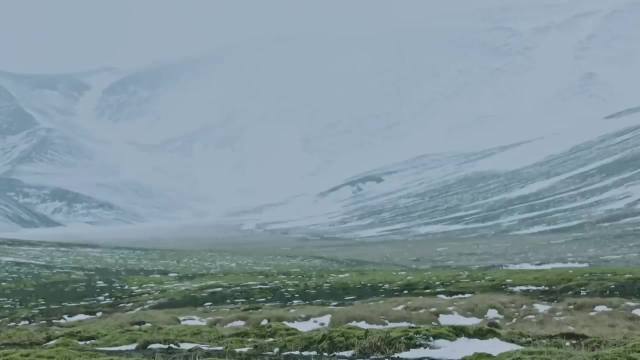 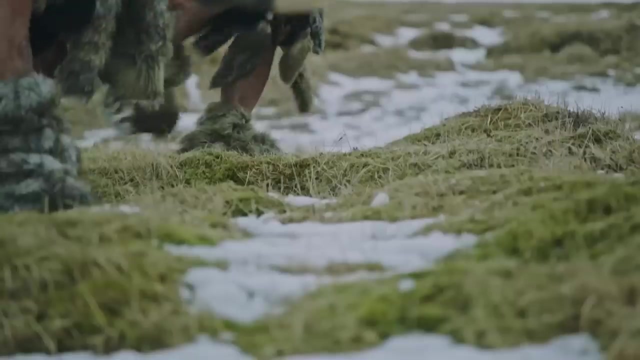 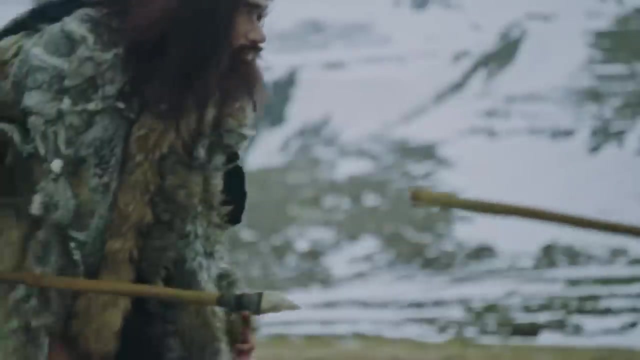 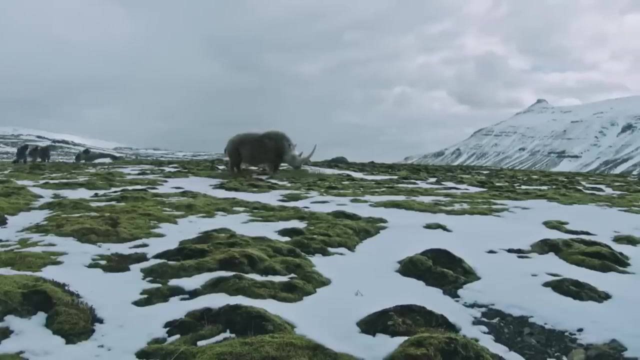 Although they lived in a similar period of time as us, Neanderthals have some unique characteristics. Neanderthals were violent and capable of hunting. They brought down deers, bears, buffaloes and even mammoths If the opponent was a powerful beast. 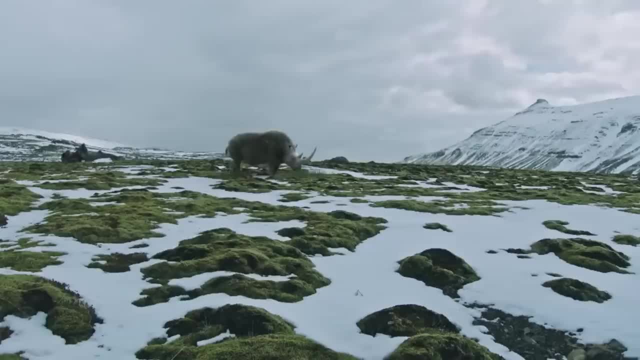 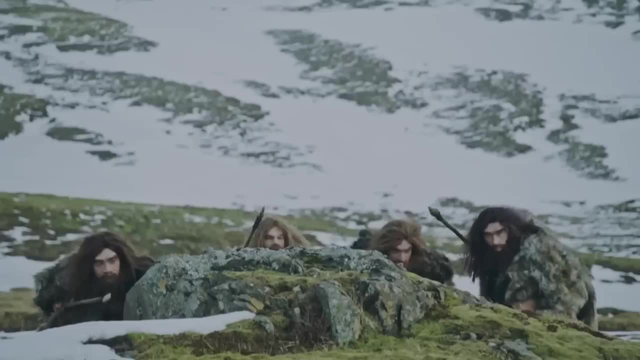 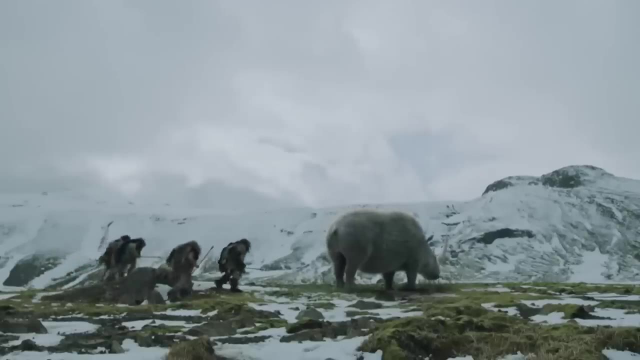 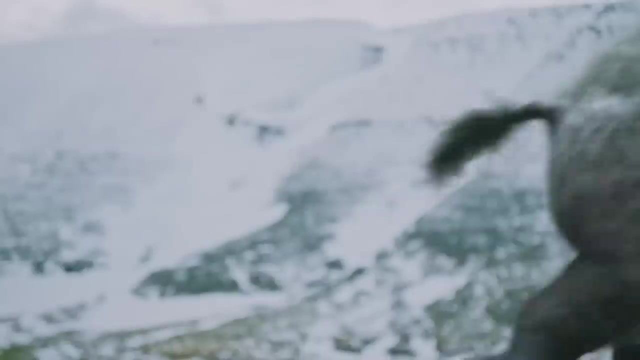 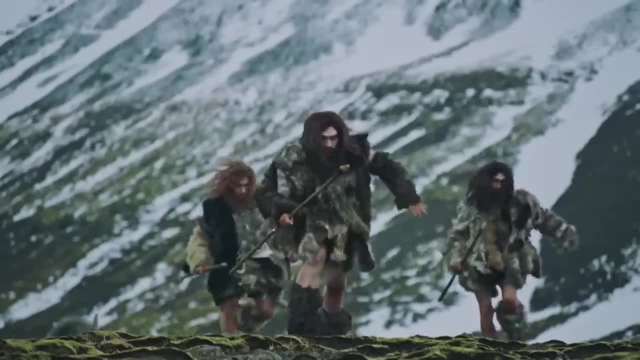 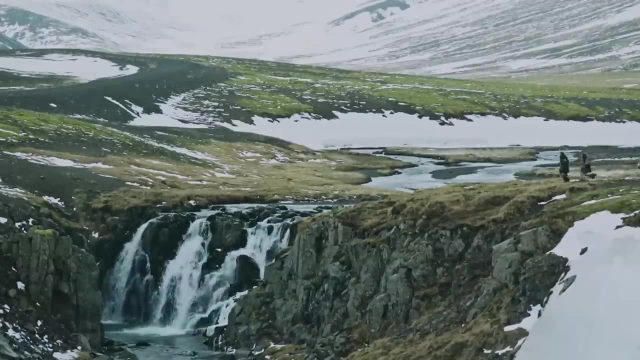 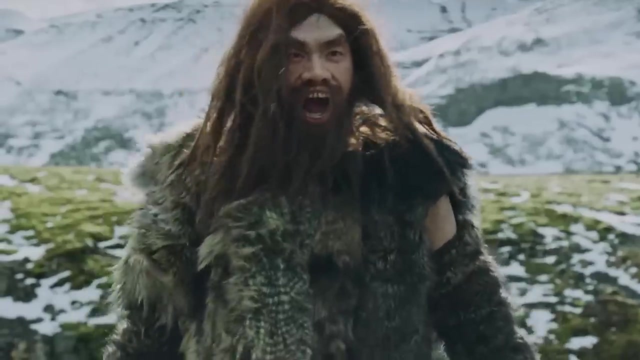 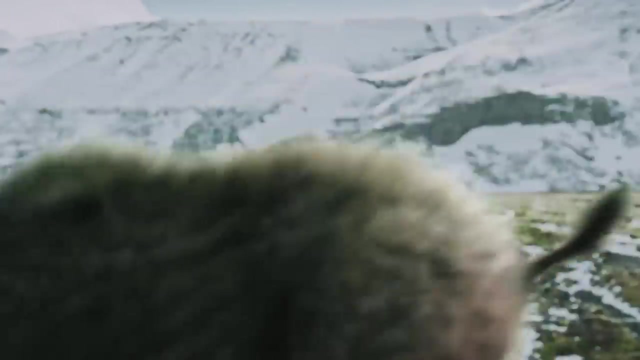 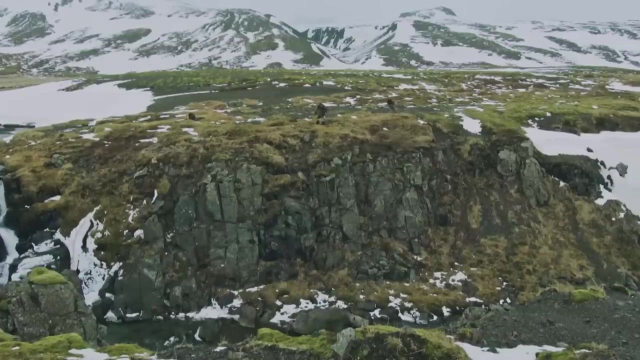 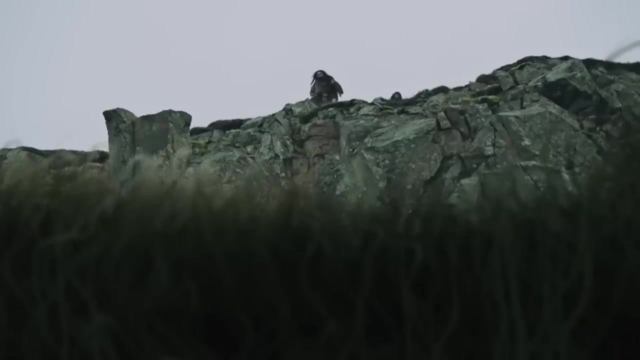 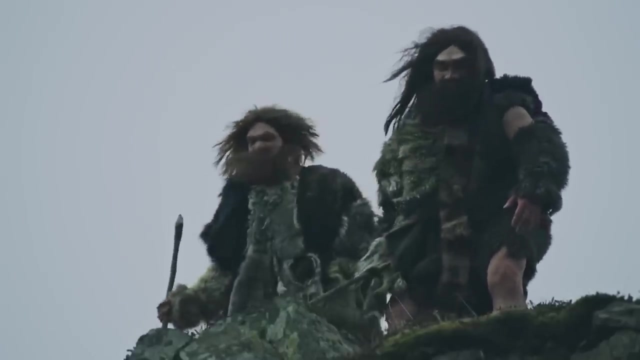 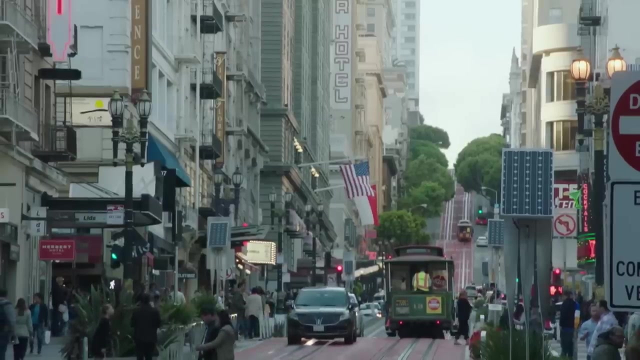 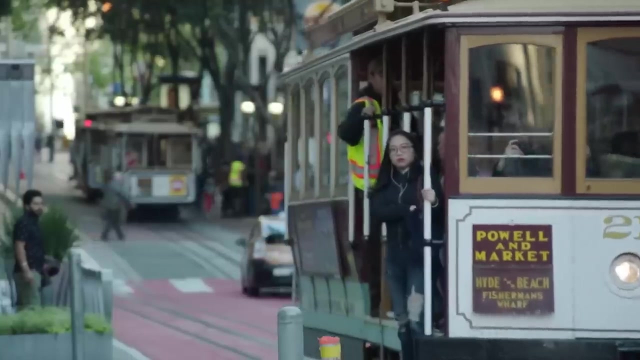 Huns determined the fate of the group. Each death was a painful loss, especially since they have a small population population, An intelligent, strong and brave human species. unfortunately, these strengths may have led to their downfall. Neanderthals were stronger and more muscular than Homo sapiens. 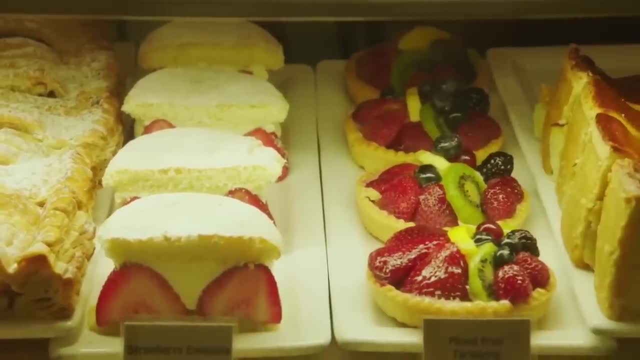 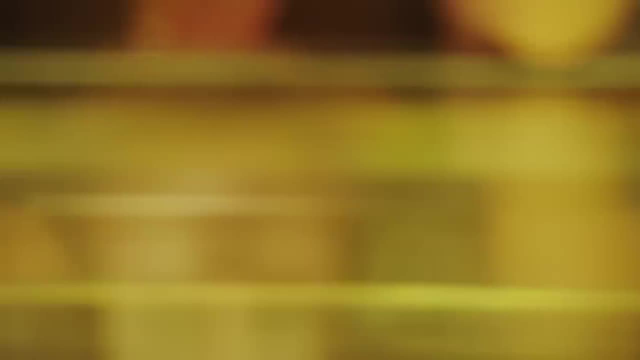 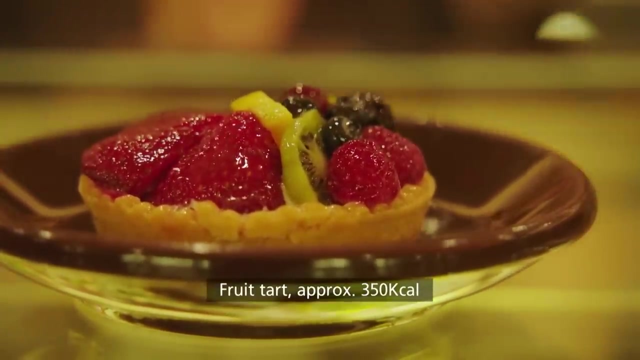 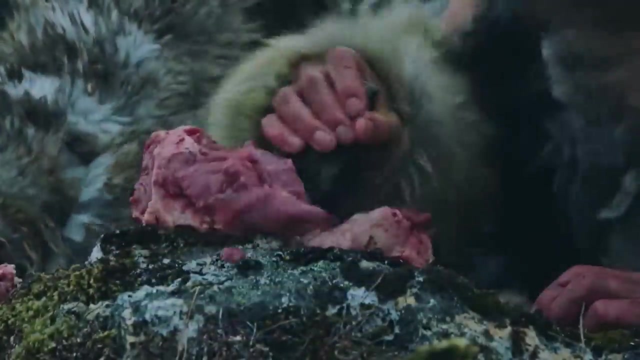 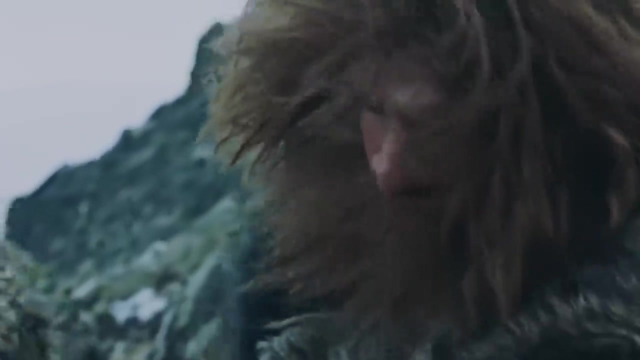 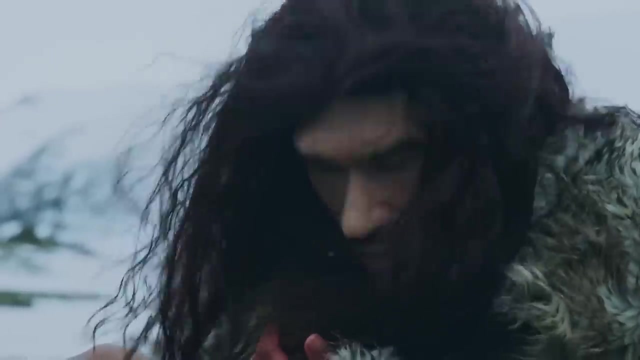 In order to maintain their body heat and strength, they needed up to 350 kilocalories more than us each day. If it were today, this slice of pie would be sufficient. Neanderthals had to hunt Throughout their lives. they either feasted or starved, depending on the outcome of their 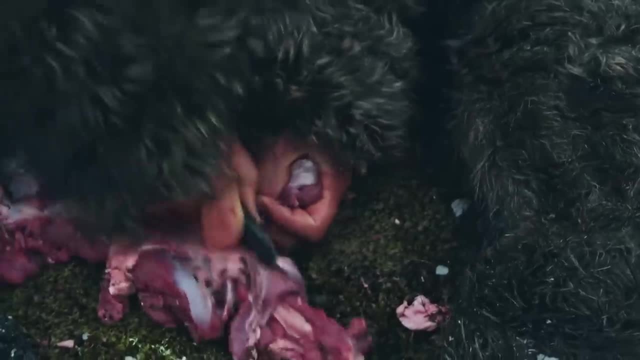 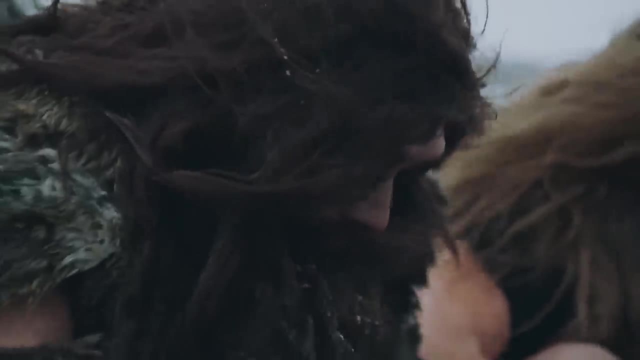 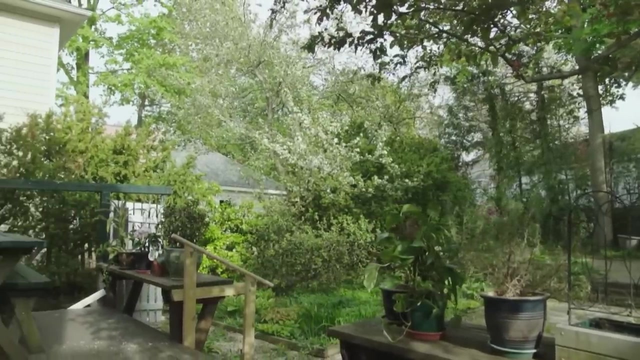 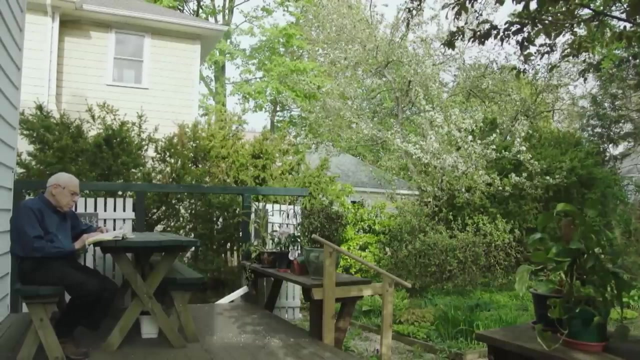 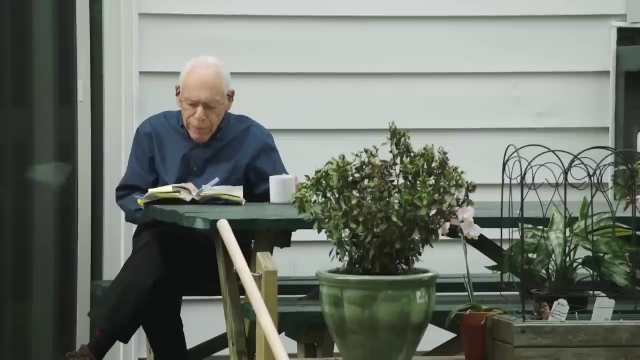 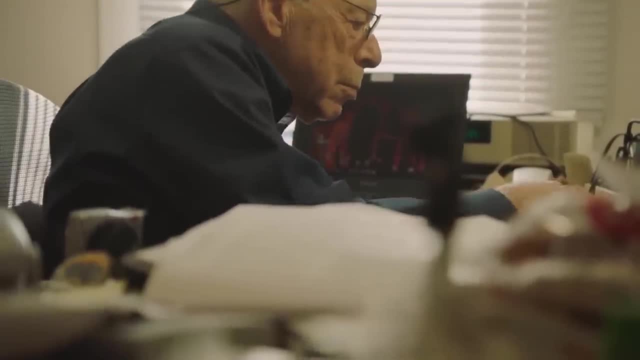 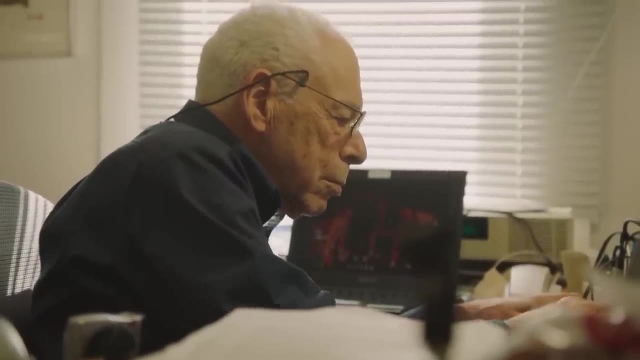 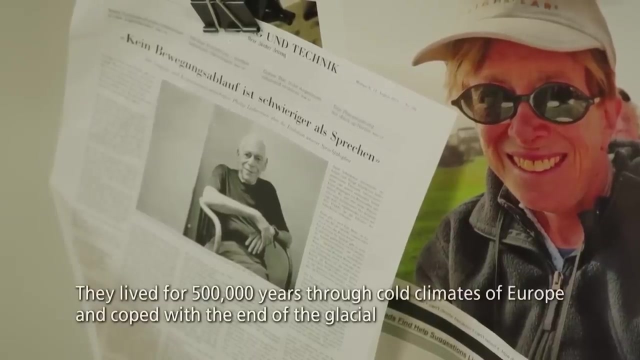 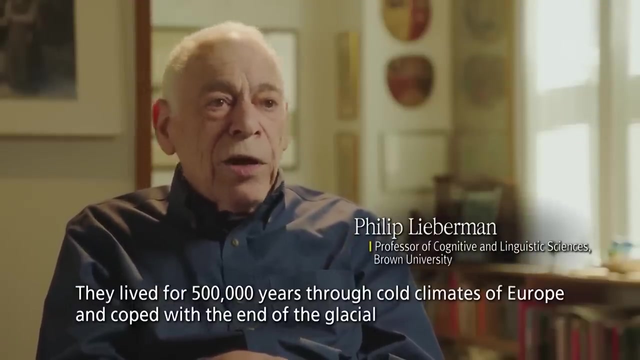 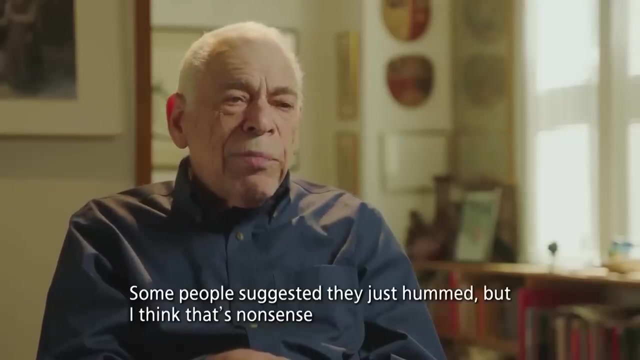 Philip Lieberman does not think that language is an exclusive property of Homo sapiens. They lived for several hundred thousand, five hundred thousand years in very cold climates in Europe that would cope with the end of the glacial. So the Neanderthals clearly had a language and some people have suggested they just hummed. 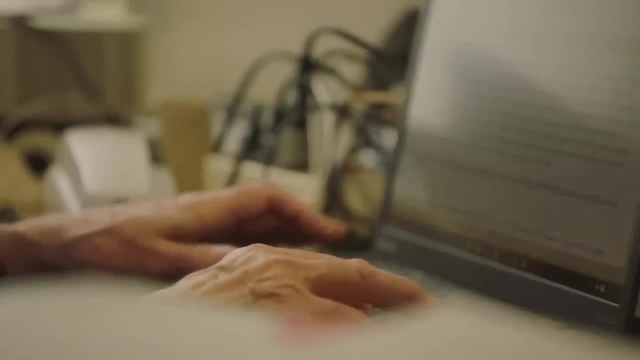 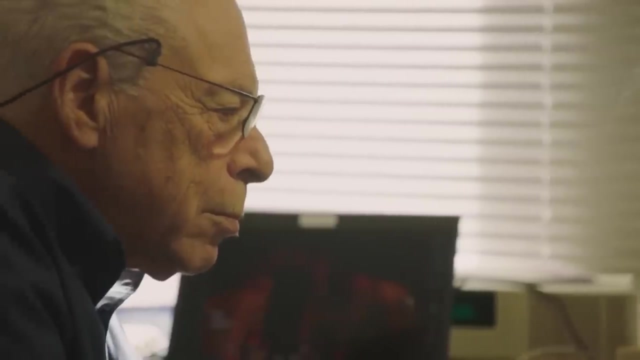 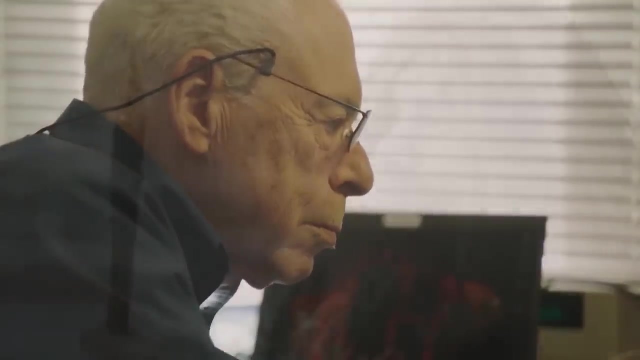 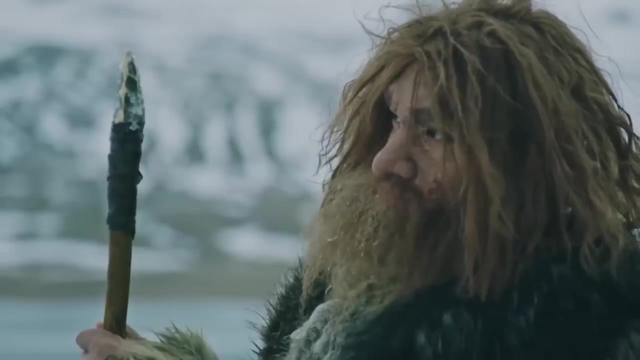 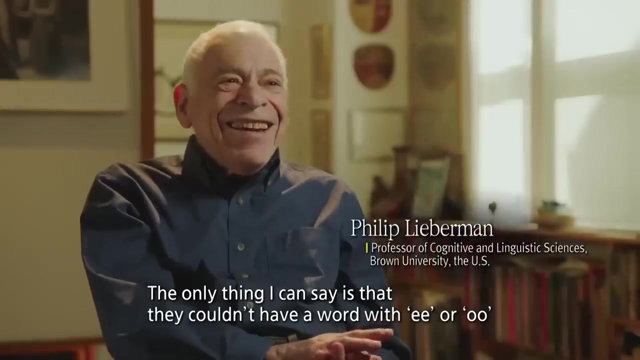 That's, I think, nonsense. The fundamental function of language is communication. It fortifies relationships. As complex as their lives had been, they must have had a language. The only thing I would say is: you can't have a word with an E or an O, and it's probably. 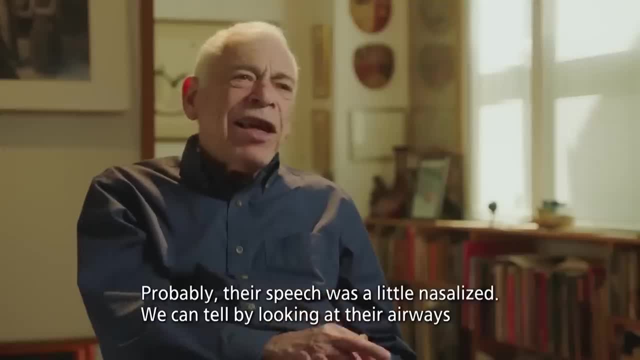 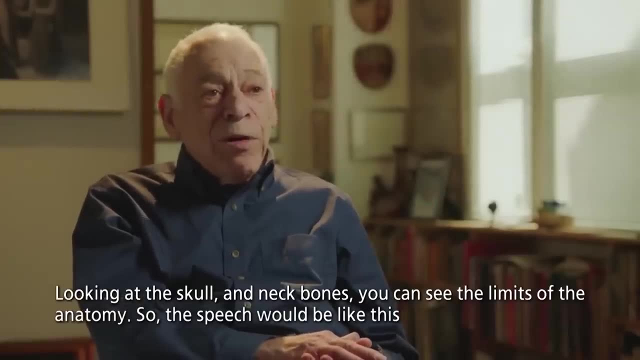 their speech was a little nasalized And we can tell that by looking at their airways. when you reconstruct, you look at the skull, you look at the neck, neck bone, bones of the neck. you can see the limits of the anatomy. 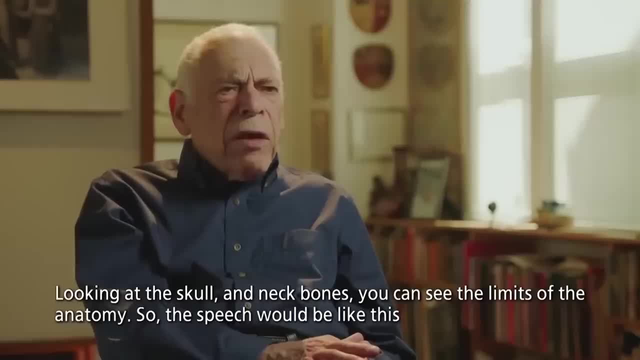 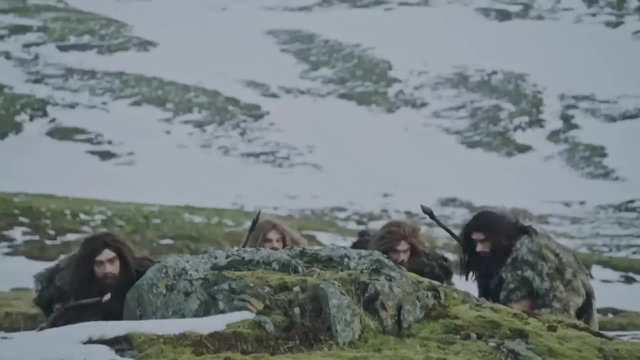 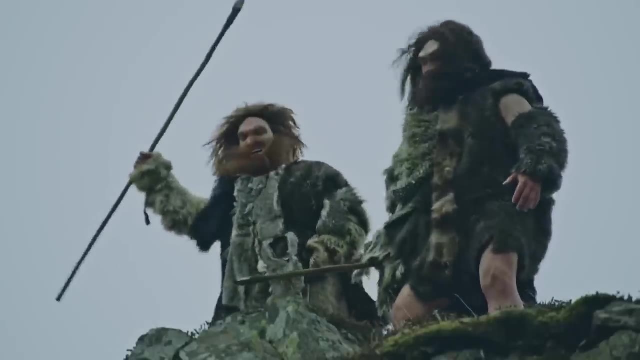 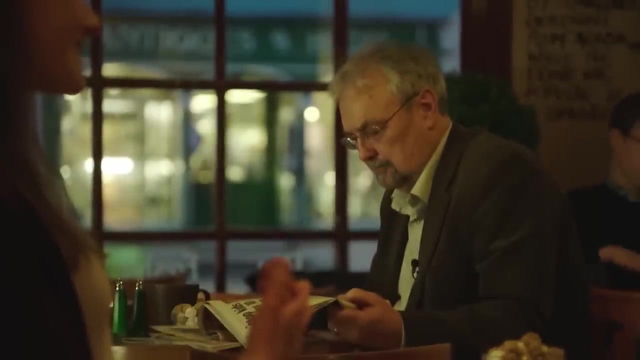 would do it, So the speech would be a little nasalized. Oh nice, Oh nice, Oh yeah, I have mine. Okay, A system of song-like sounds to convey emotion, Gestures with meanings, Languages, consolidate groups. 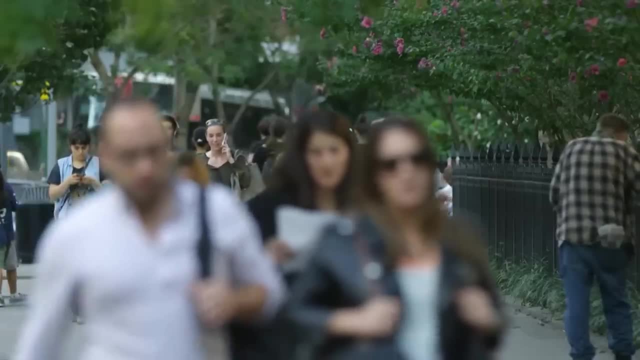 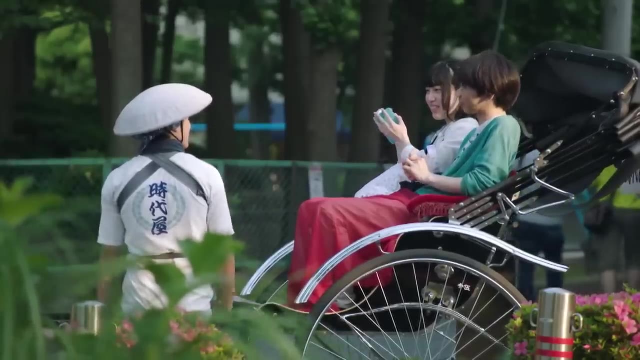 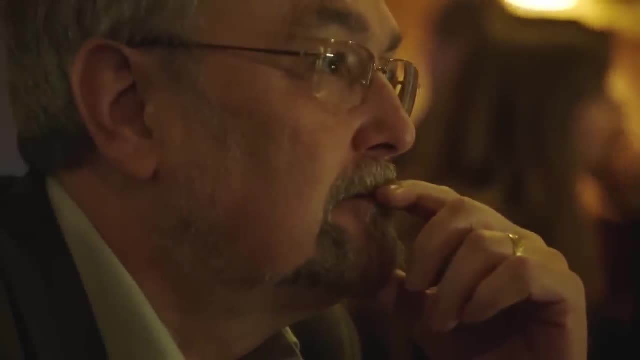 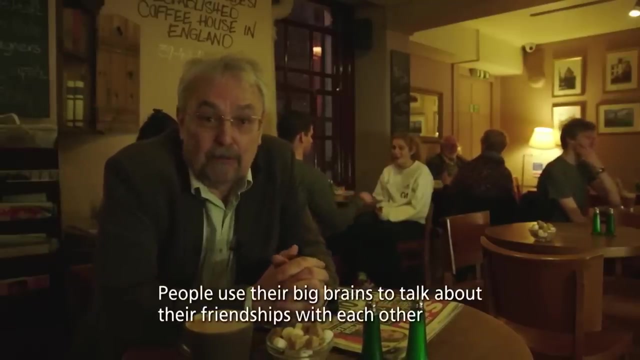 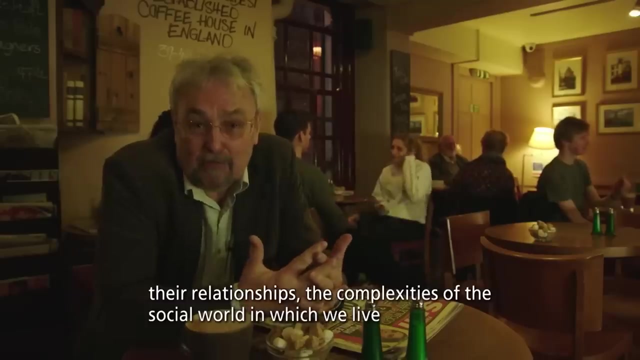 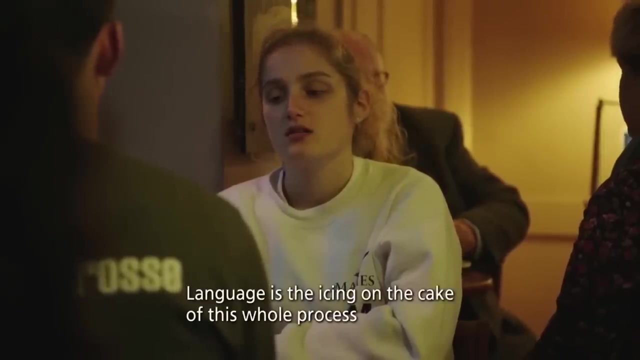 Professor Dunbar believes that these human relationships had an effect on the human brain. People use their big brains to talk about their friendships with each other, their relationships, the complexities of the social world in which we live. That's the icing on the cake of this whole process. 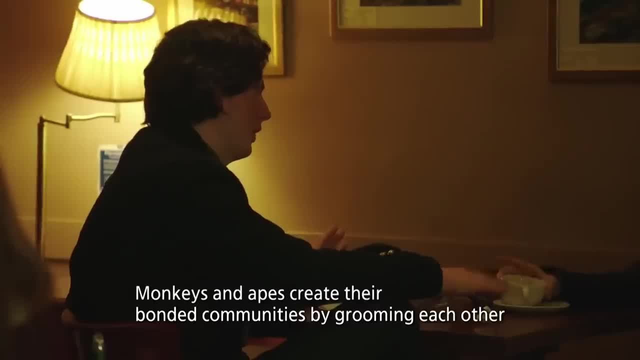 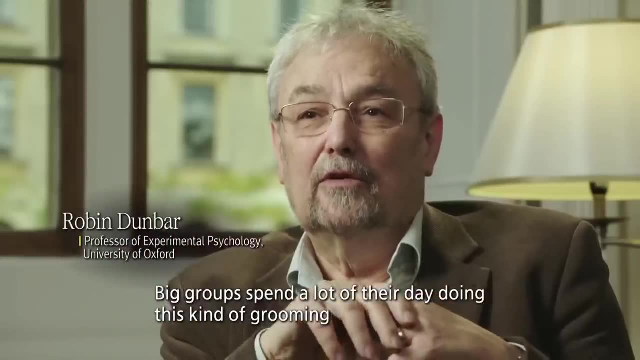 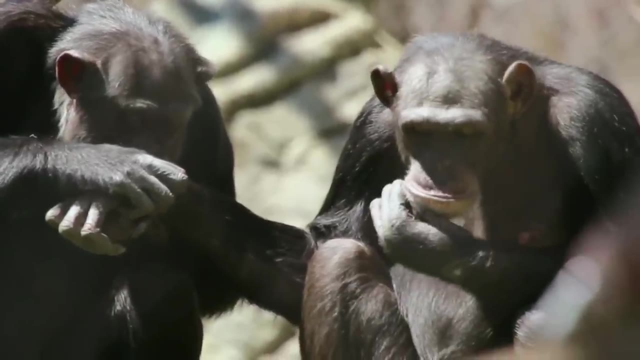 Monkeys and apes create their bonded communities by grooming each other. They live in big groups, spend a lot of their days together. They're doing this kind of social grooming to each other. Somehow, language is like grooming. Usually apes groom one ape at a time. 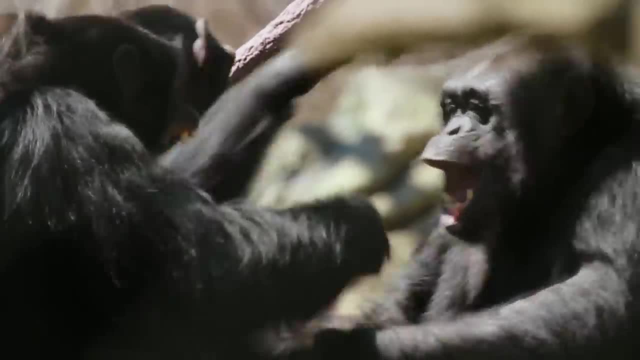 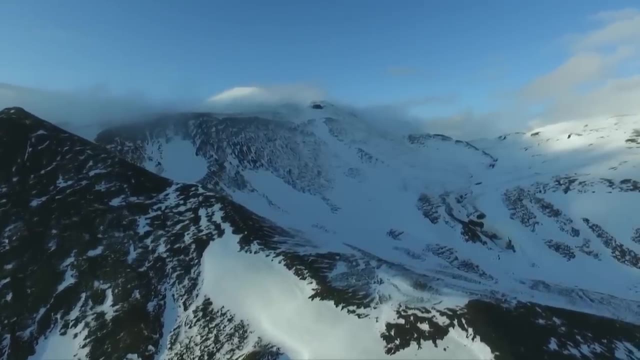 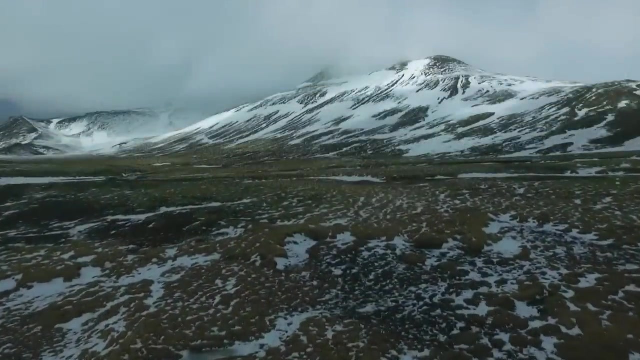 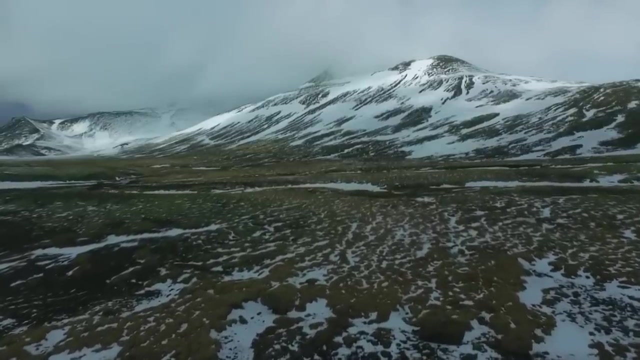 However, language is conveyed to multiple people at once. The reason humans were able to form larger groups than apes was because of this language. Neanderthals, who had larger brains than us, had entered the realm of language first, But what made them disappear? 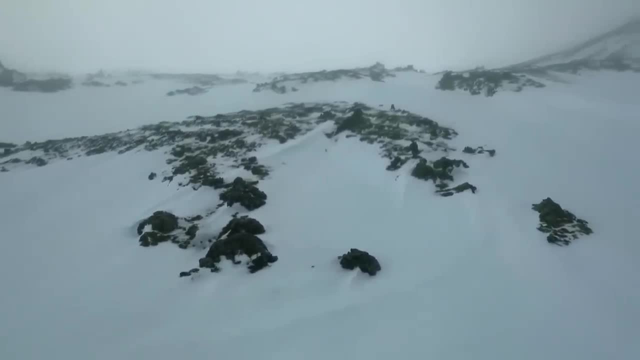 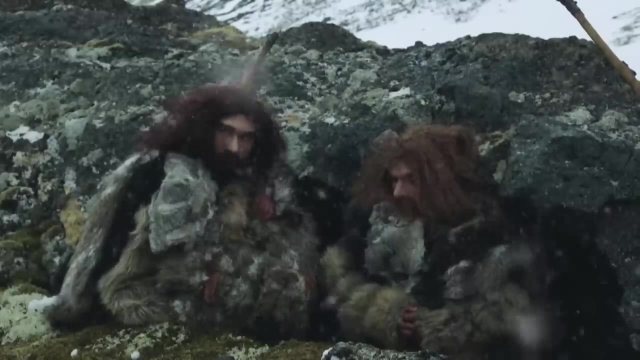 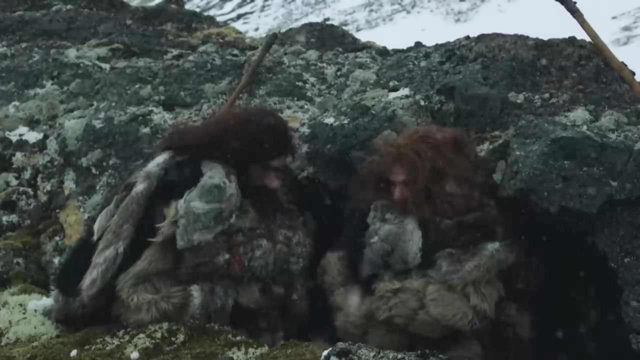 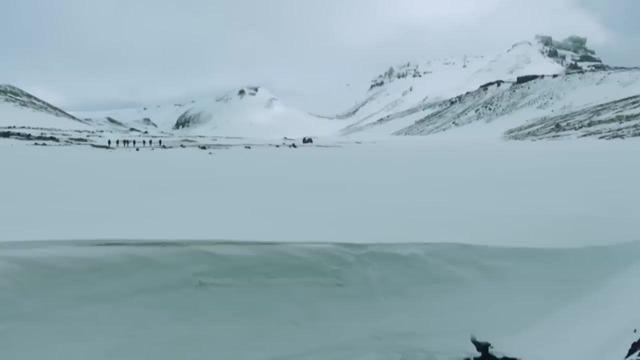 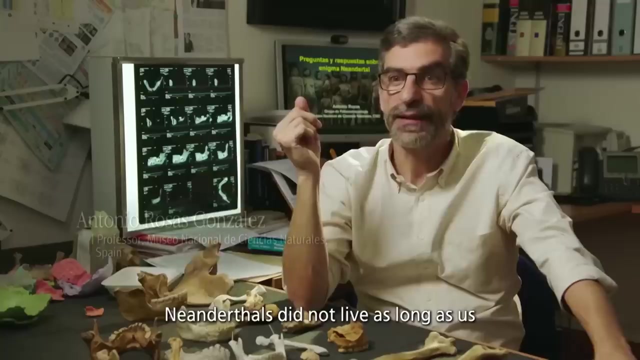 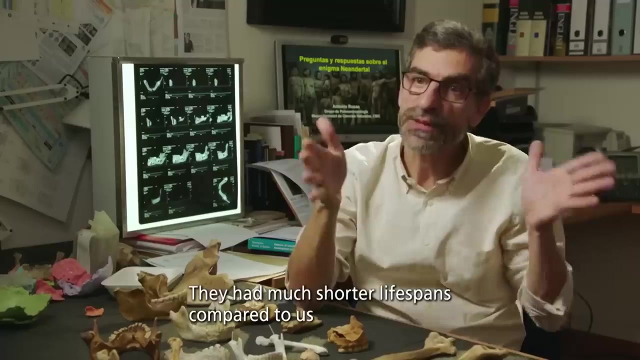 Was it the climate? We survived the cruel coldness in the final glacial epic with them? Then why is it us who are left standing? But fundamentally, they didn't live. their longevity wasn't as extended as ours, but probably their lifetimes were much shorter than ours. 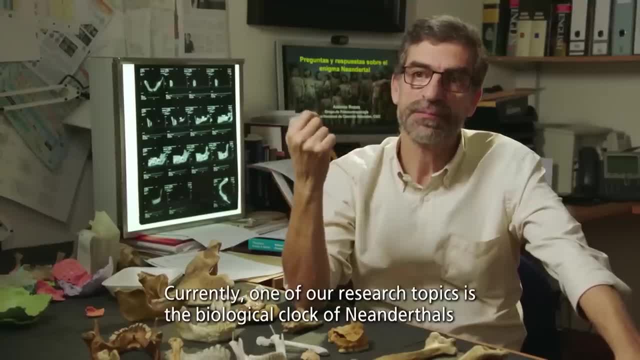 One of the aspects we are now studying is precisely the cycle of life. One of the aspects we are now studying is precisely the cycle of life. One of the aspects we are now studying is precisely the cycle of life. One of the aspects we are now studying is precisely the biological cycle of Neanderthals. 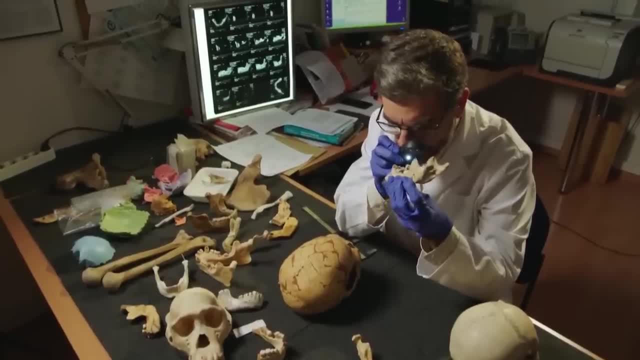 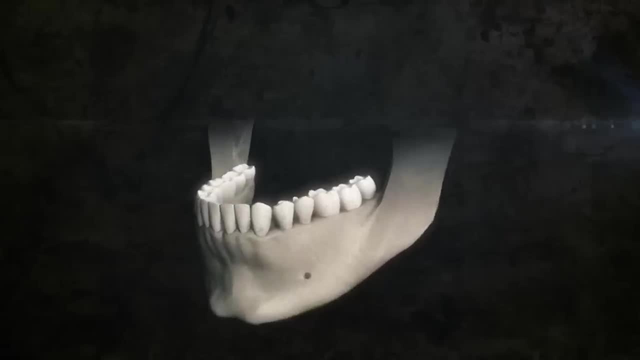 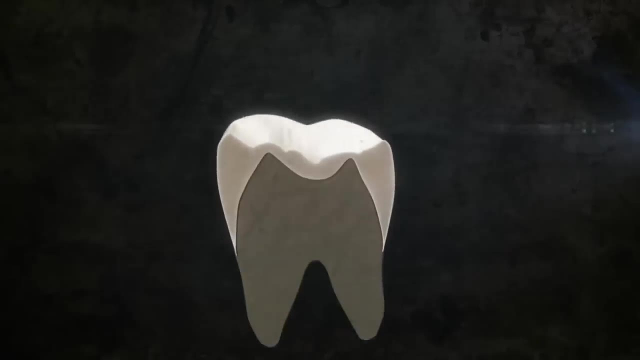 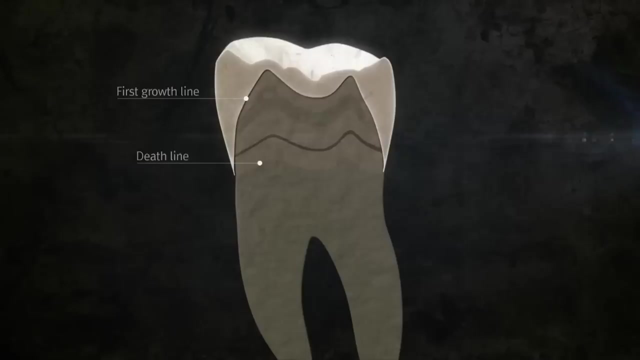 A tooth is a record keeper of an individual's entire life. It can be used to reconstruct the biological clock of primitives. Teeth grow like trees. Layers are accumulated. The part formed first rises to the top. The lower part of the tooth tells the death time of an individual. 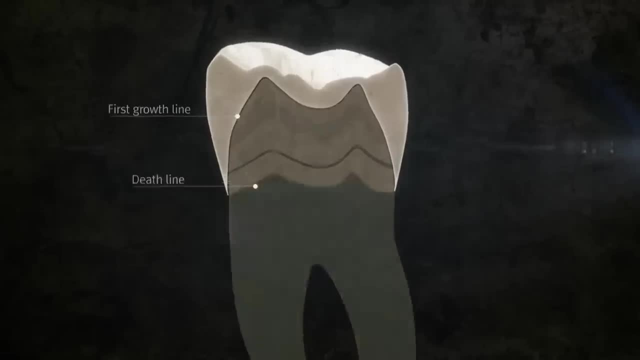 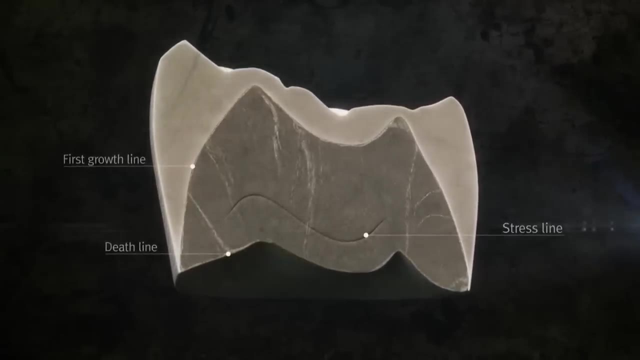 Lines are formed when an individual suffers from poor nutrition or disease. These lines can be used to speculate periods of great stress. We have seen that Neanderthals go through a crisis in their growth time. We have seen that Neanderthals go through a crisis in their growth time. 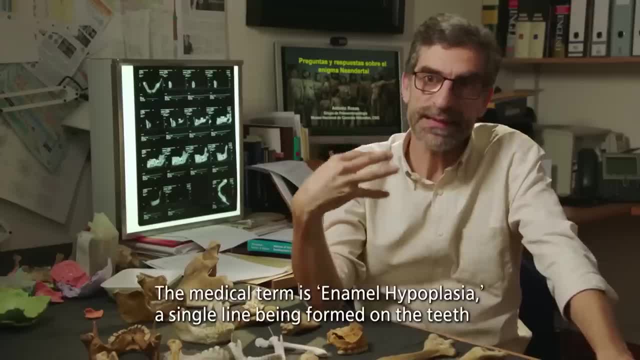 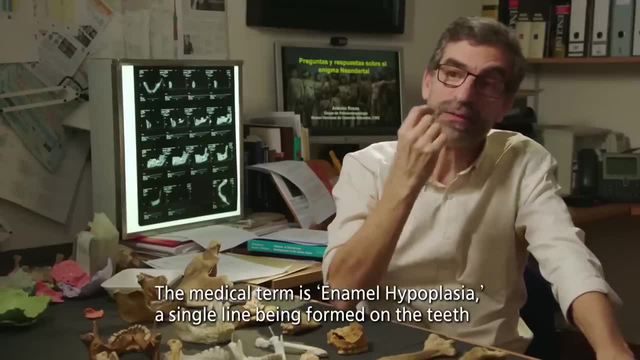 We have seen that Neanderthals go through a crisis in their growth time, en su crecimiento Y esa crisis se manifiesta en lo que llamamos técnicamente hipoplasia dental, Es decir en los dientes aparecen unas líneas. 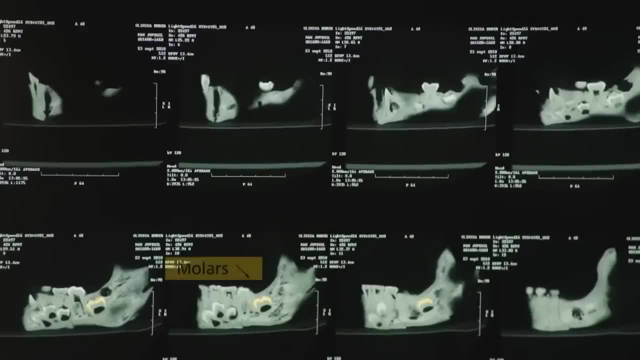 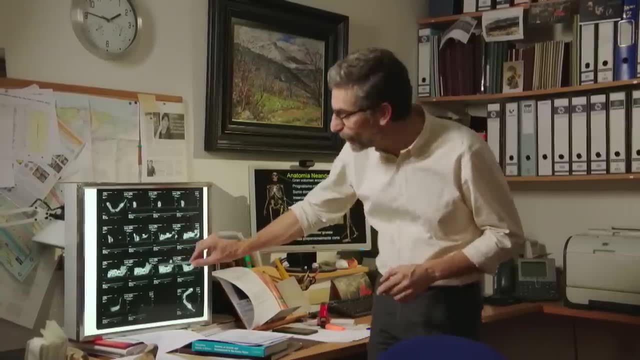 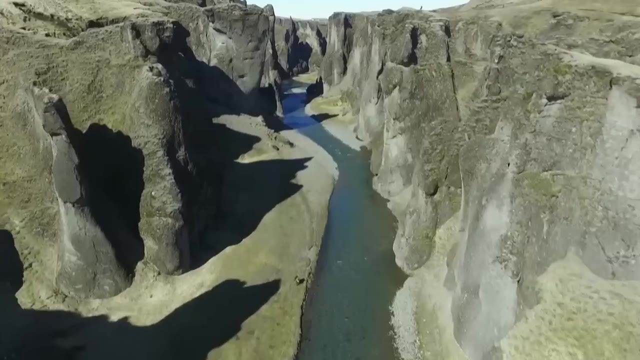 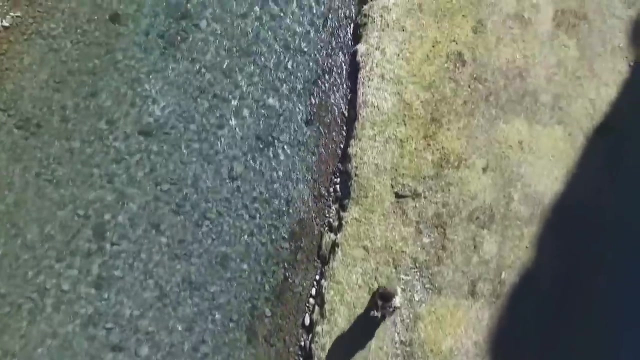 While we get permanent molars at the age of 10, they get molars at the age of 6.. Their childhood was four years shorter than ours. Neanderthals had no time to enjoy their childhood. They had to grow up fast to replace the adults who died early. 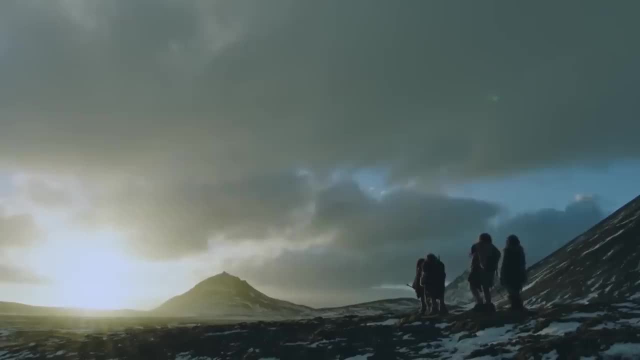 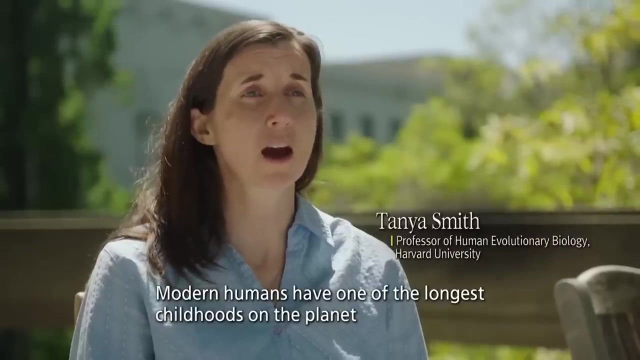 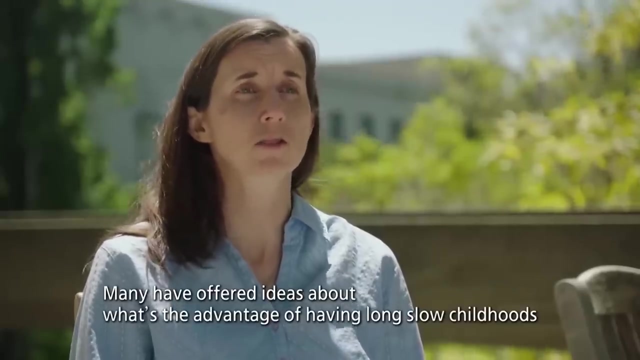 At the end of the glacial epic, their population had dwindled to 5,000.. Why would we slow down our childhoods? You know modern humans have one of the longest childhoods on the planet and many people have offered ideas about what's the advantage of having a long and slow childhood One. 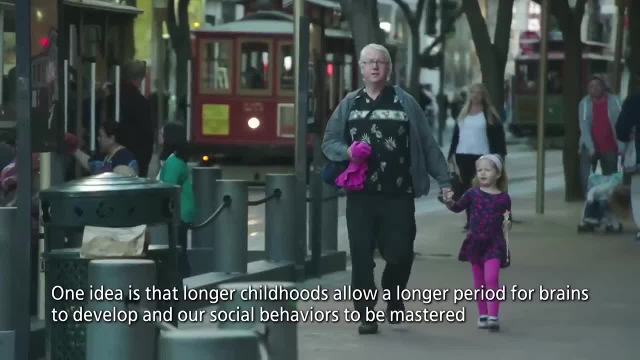 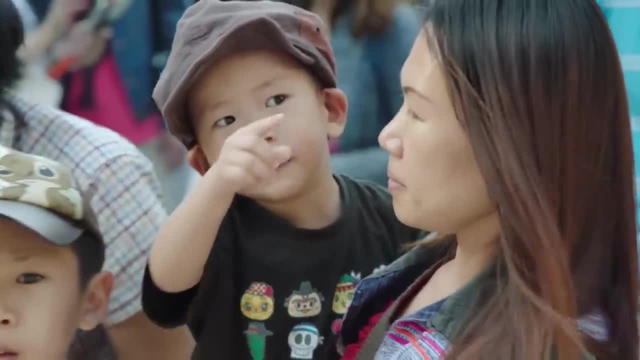 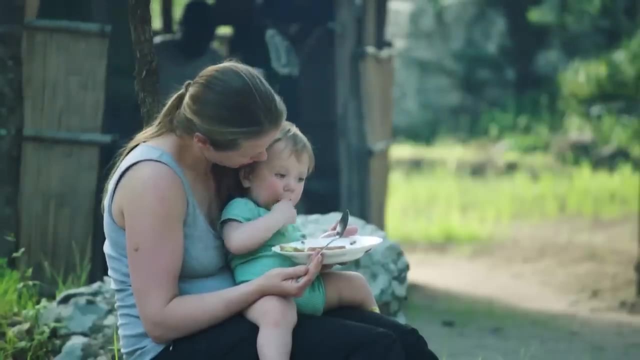 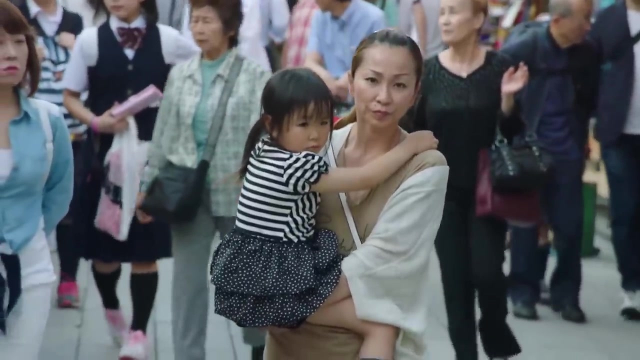 idea is that modern humans allow a longer period for our brains to develop and our social behaviors to be mastered. During childhood, we learn the complex rules of society. The brain develops in quality during this time. What Homo sapiens had and the Neanderthals did not have was a long 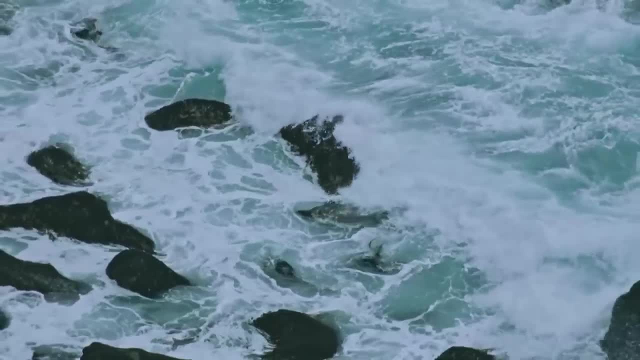 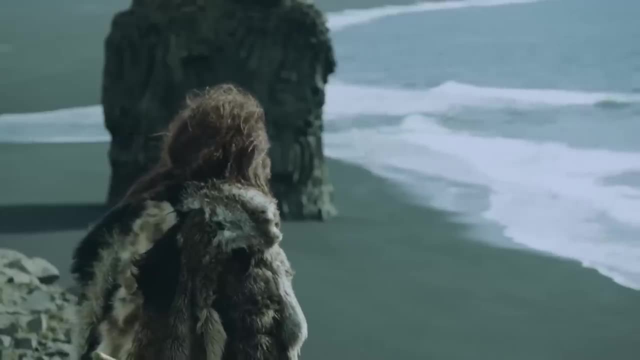 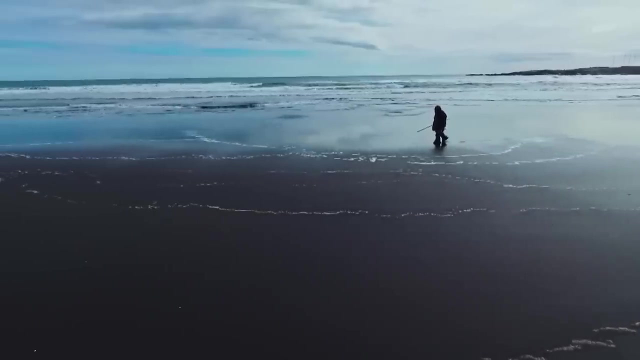 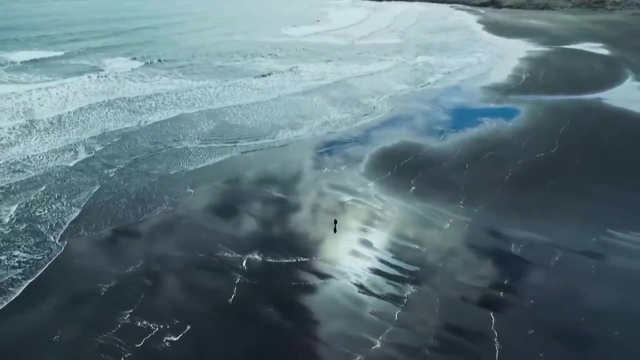 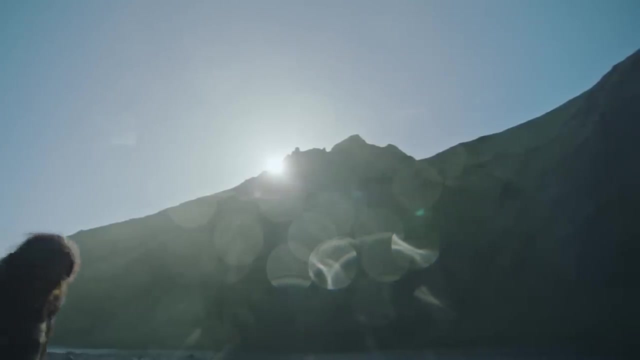 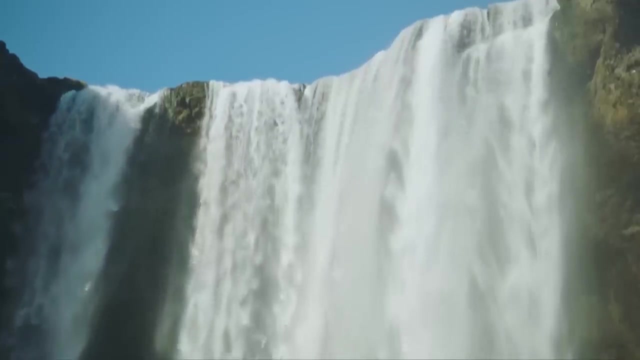 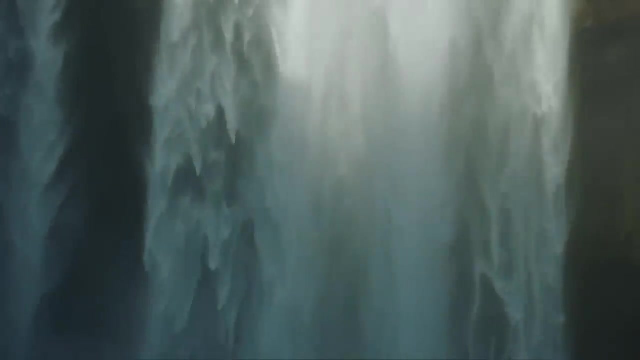 childhood, The last individual standing From 15 to 10 to 4, then to 5 and finally alone. Near the end of the final glacial epic, Neanderthals vanished from the earth. Eventually, all species may encounter such a fate. 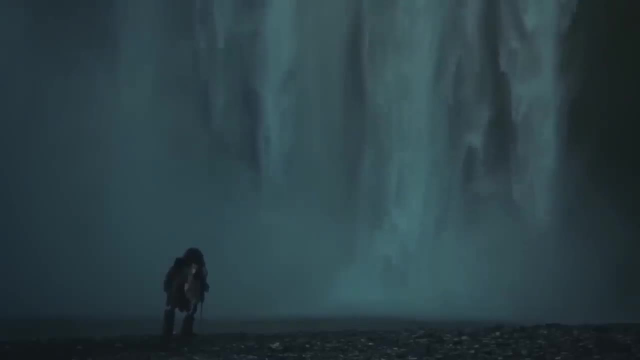 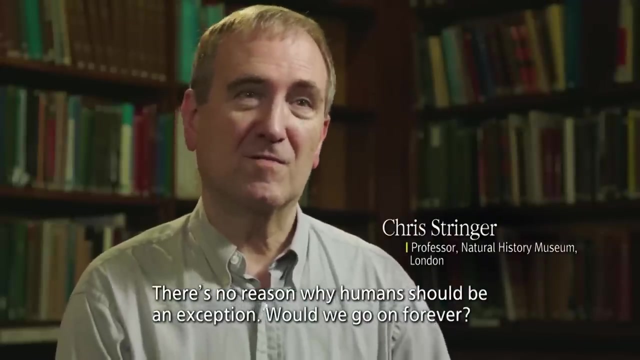 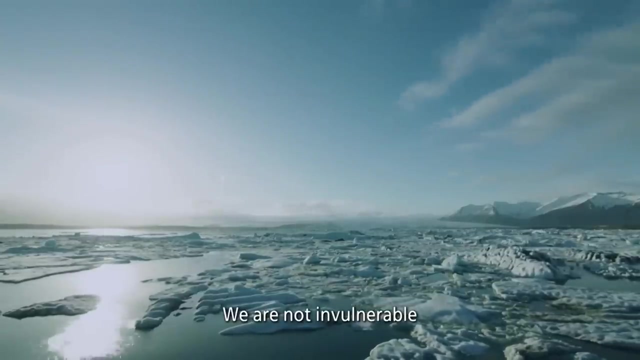 There's no reason why humans should be an exception that will go on forever. When we look in the past, it's the fate of almost every species that existed in the past disappeared In our own case. yes, we are not invulnerable. I think humans. 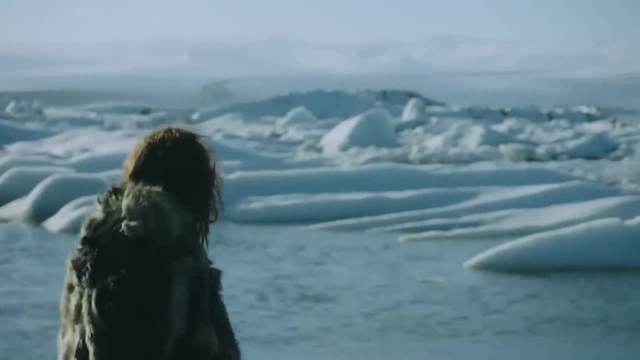 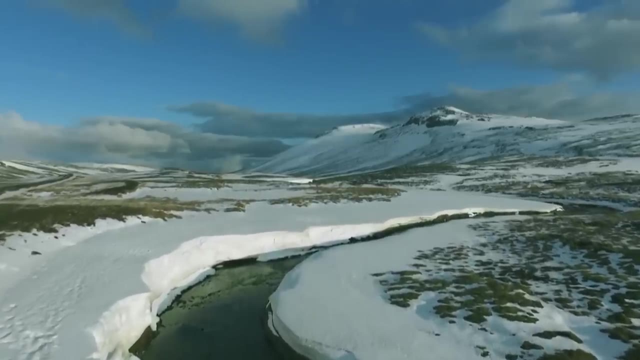 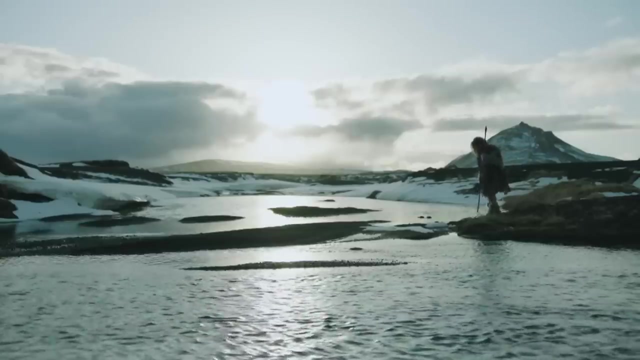 we could go extinct in the future. of course we could. Neanderthals are the only species that can survive. Neanderthals are the only species that can survive. In the final 30,000 years, Neanderthals and Homo sapiens had met.